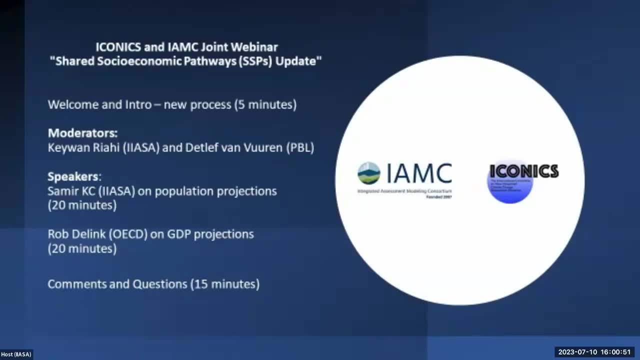 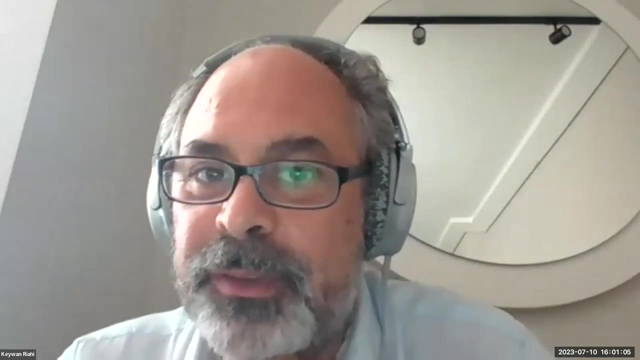 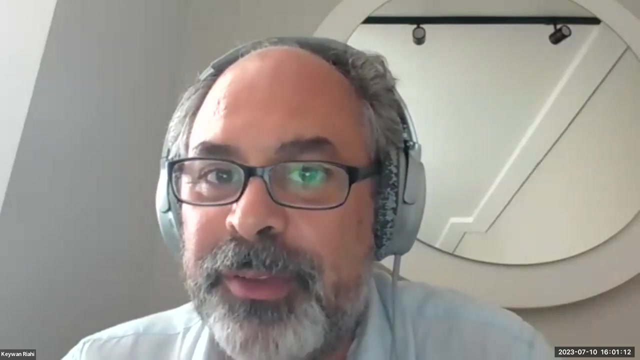 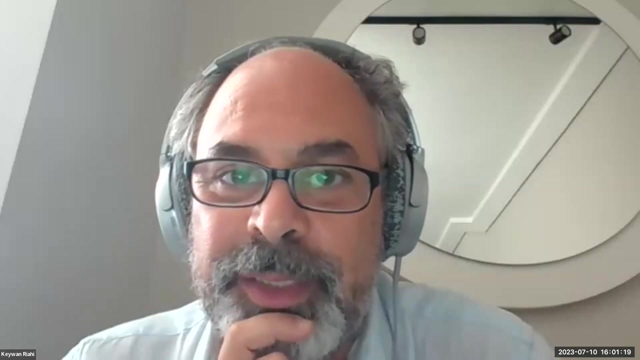 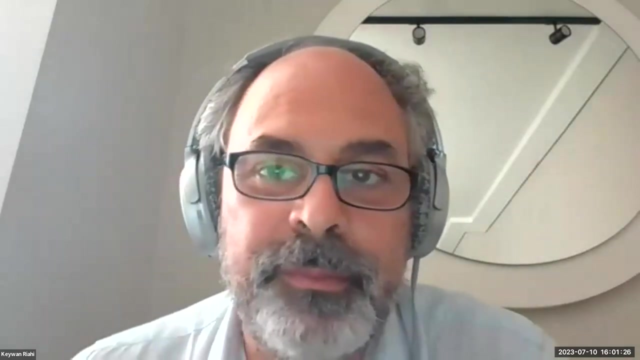 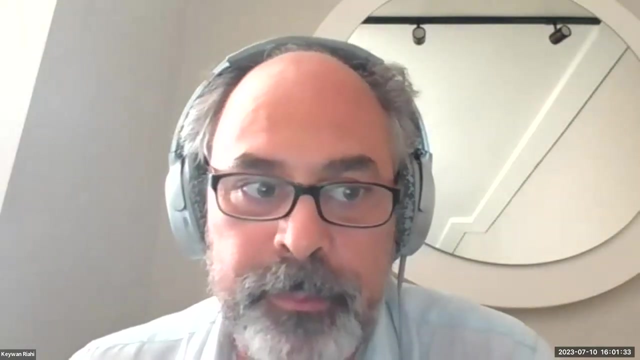 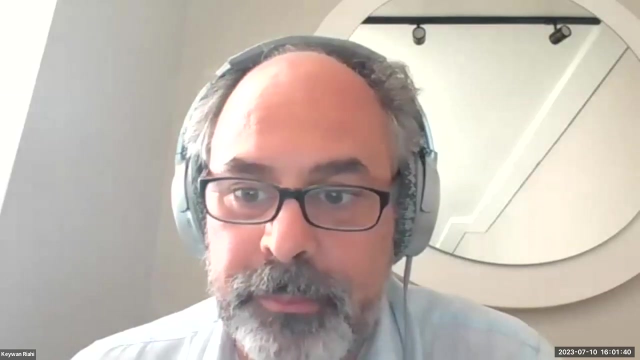 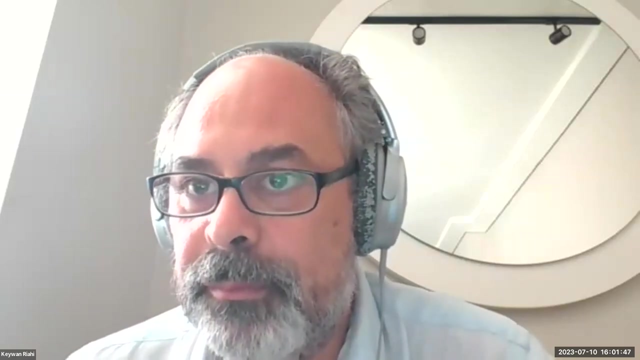 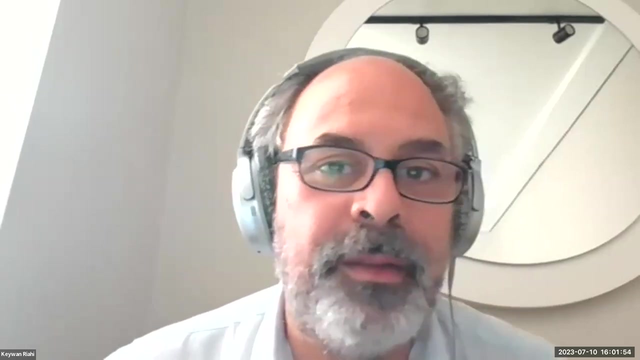 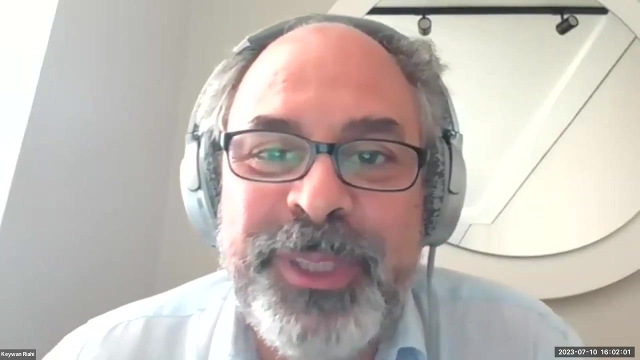 Yeah, welcome everybody. I think we are all in the same webinar room right now. Let us wait a few minutes until the participants count is stopping to go up, you know, at a little bit more than 80.. Kevin Riachi, Yeah, I think we should start. Welcome, Welcome. 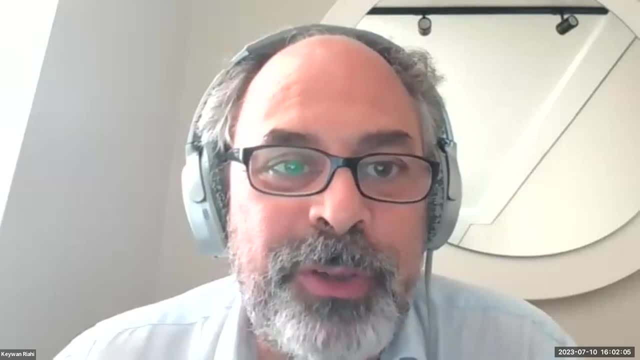 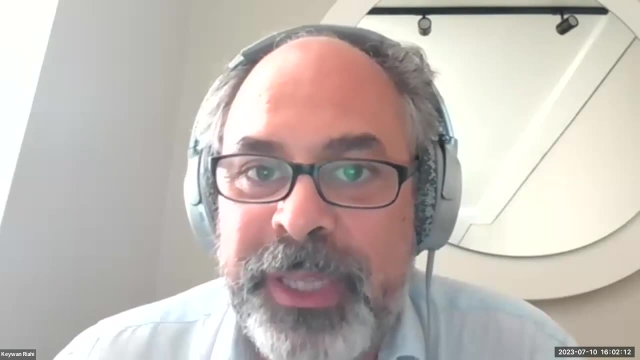 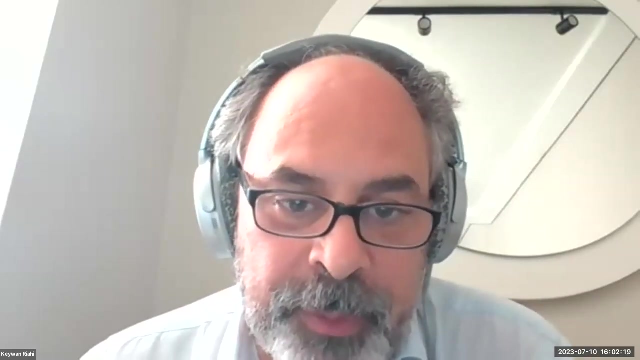 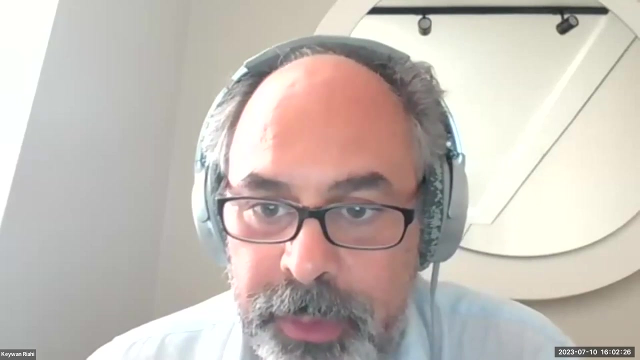 everybody to this webinar on the shared socio economic pathways. My name is Kevin Riachi, I'm from YASA and, together with colleagues, we will present new, updated SSP projections. But let me perhaps share my slides with you One second, that's just here. 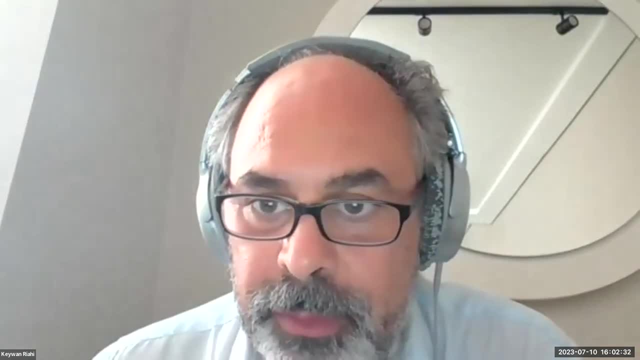 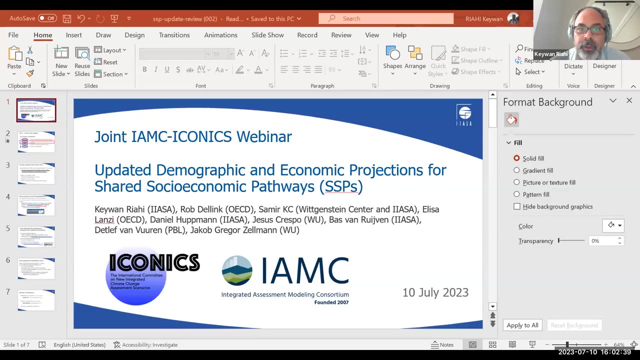 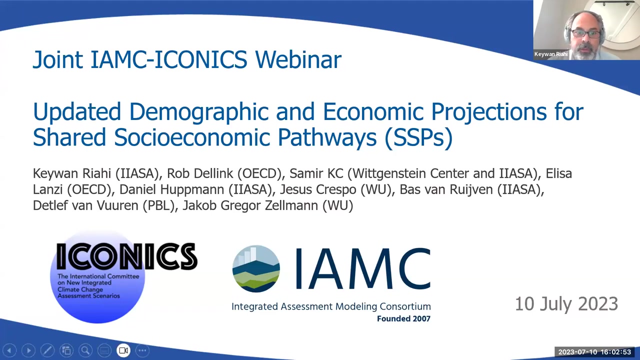 Here it is, So I hope you can see the presentation mode. Yeah, Okay, so it's quite some time since the SSPs have been developed- roughly 10 years ago- And today's webinar is about the first phase of updating the scenarios, the SSPs and particularly 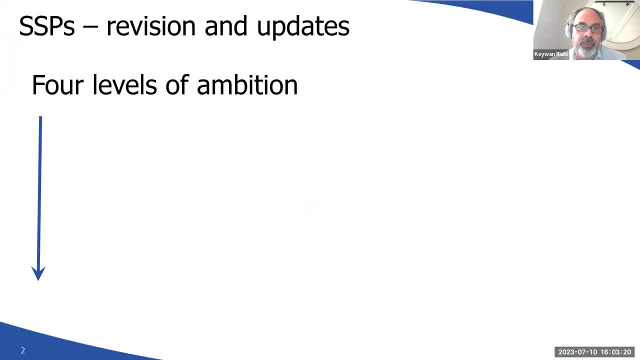 the basic elements, which are the demographic and economic projections of the SSPs. We will hear two presentations about new projections that will become available very soon and which for which you would like to organize a community review. So this is also the launch of the review process of updated SSPs. 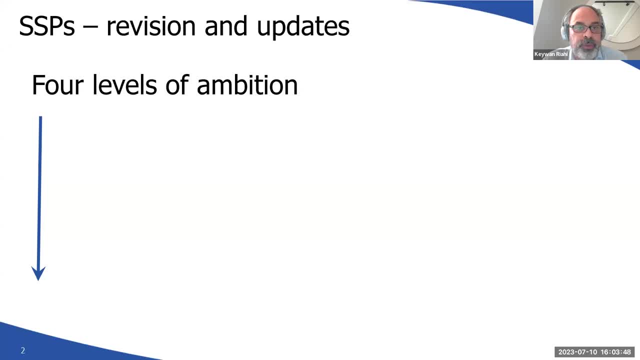 Basically in updating the shared socio-economic pathways there are. there are four levels of ambition possible. They have been there for quite some time, Since about 10 years, as I mentioned earlier- and the updates of the SSPs could include, for example, just updating the base year, so that 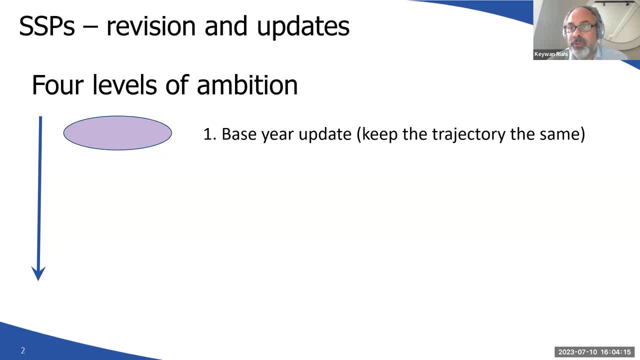 basically, the trajectories are consistent with historical projections. Such updates have been made available just recently as part of the Navigate project. We are now in the second phase, if you wish, where we have worked together with the economic teams from the OECD and also from the Vienna University. 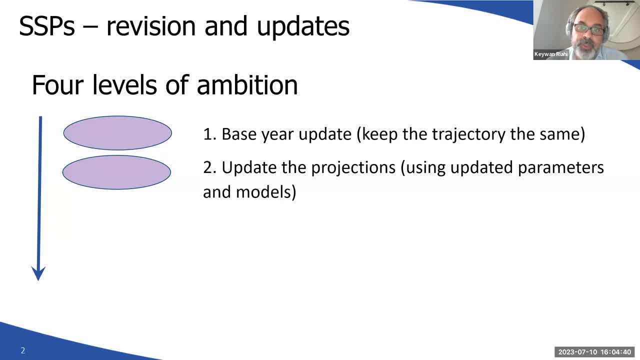 as well as with the demographers from the Wittgenstein Institute and the ASA, to provide a full update of the projections, also using updated parameters and models and particularly taking, for example, recent trends into account, such as the COVID- COVID incidents. 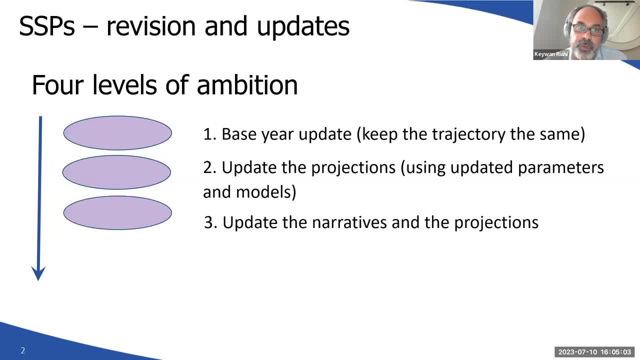 And then there are further increase of course in. I see a raised hand. I would suggest we wait with the comments et cetera to the end of the webinars. After each of the presentations you will have time to raise initially technical comments. 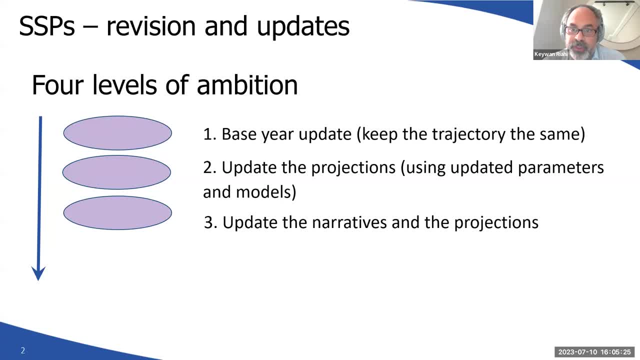 but then also at the end we'll have a discussion about the results and further explanations about the review. Yeah, so the third level of ambition would, of course, be to update not only the quantitative projections but to revisit the narratives and either expand the narratives or change. 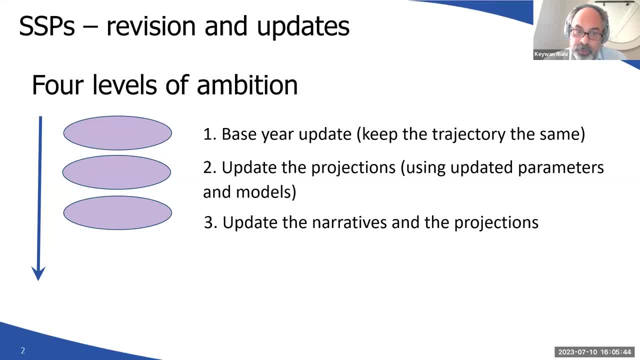 the narratives And, of course, in the very long term also, something that would be important to do is to think about updates and visions of the total framework. Today, This webinar is particularly focusing on this first phase and initial products that are becoming available for the updated projections and new quantifications using the OECD. 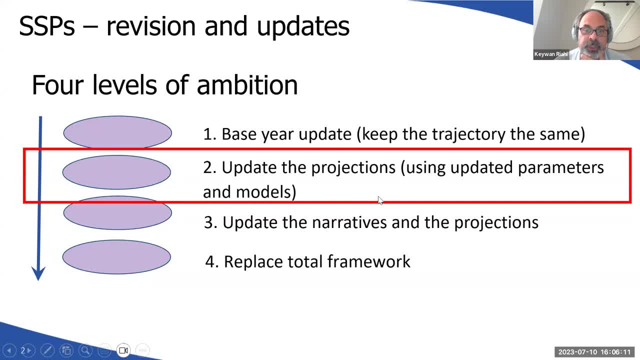 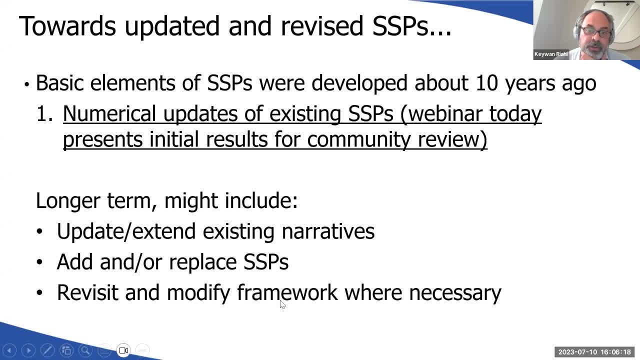 and the Wittgenstein-IASA models for GDP and population, And this will be basically the numerical updates and the longer term. Of course, the process might include also revisiting narratives and replacing SSPs, looking at at the SSP framework as a whole. 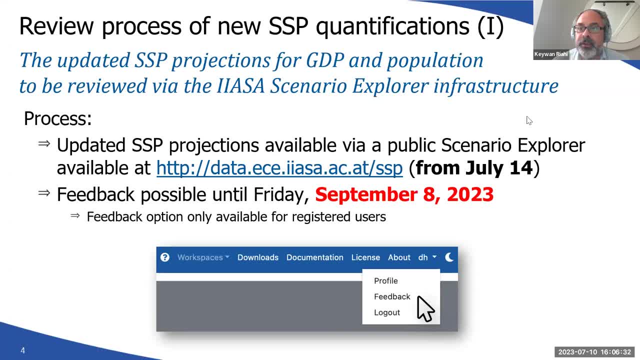 Some practical, some practical comments on basically how you on the review process. As of July 14th, the quantifications will be available to an scenario explorer where you can go, which you can visit and where you can see the data. 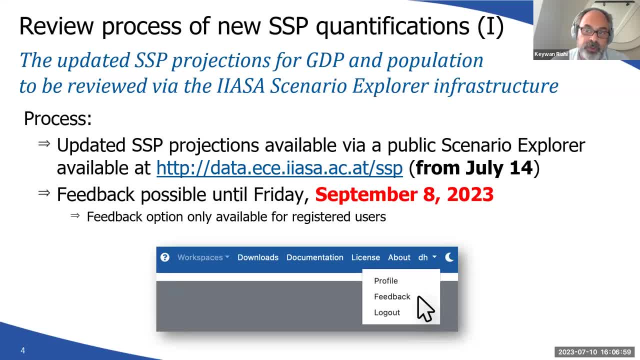 The data can also be downloaded and the scenario explorer also provides features, provides the possibility to make analysis with the scenarios, And we would like to ask you and the community to basically provide feedback on the quantifications as they look at the moment, until September 8th 2023.. 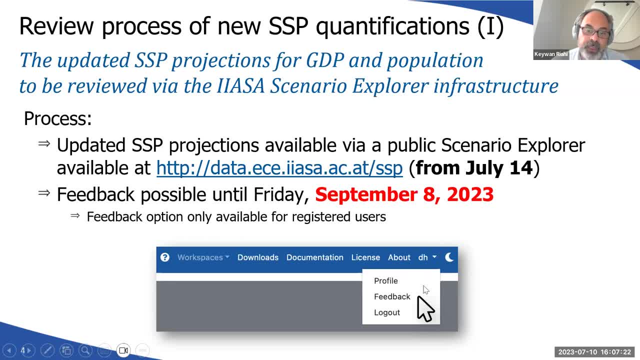 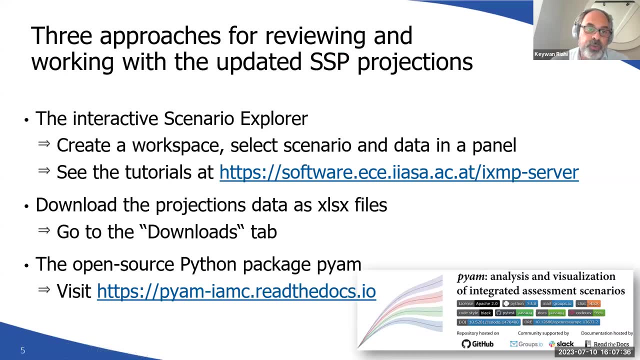 And this feedback can be provided directly in the explorer. if you register to the explorer and create a profile, There will be a button with feedback where you can provide the feedback And basically there are two different ways to use the data and to work with the projections. 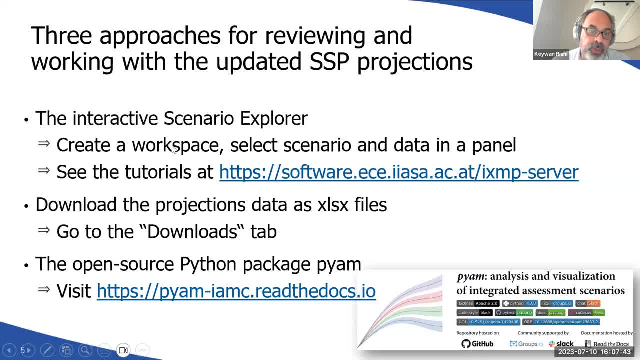 At the one hand, the interactive features in the scenario explorer, where you can create your own workspace, make analysis and share that analysis with other explorer users or with us. But you can also, if you don't want to use the explorer, simply download it. 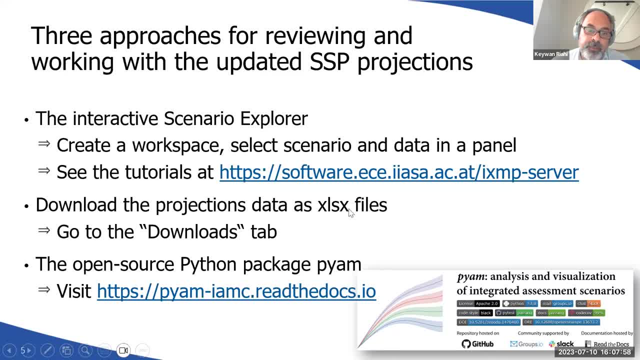 Simply download Excel files later on and work in your make your own analysis to review the data, Or you can use an open source package, a Python package, which enables to, for example, do relatively easy visualizations of the data that will be made available at the end of. 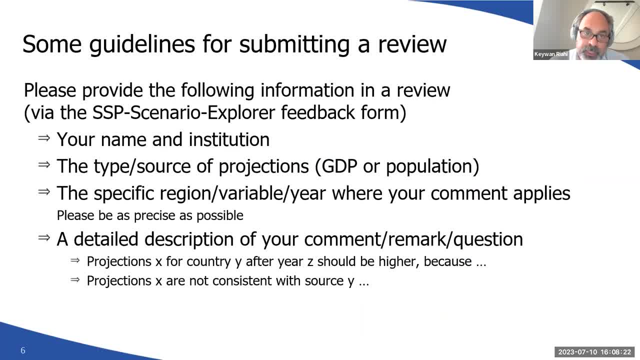 this week Some further guidelines for submitting the review. We would like to ask you, if you provide review comments or feedback, to please state your name and institution, to please be clear about what part of the data you are commenting on, whether this is, for example, the GDP projections or the population projections. 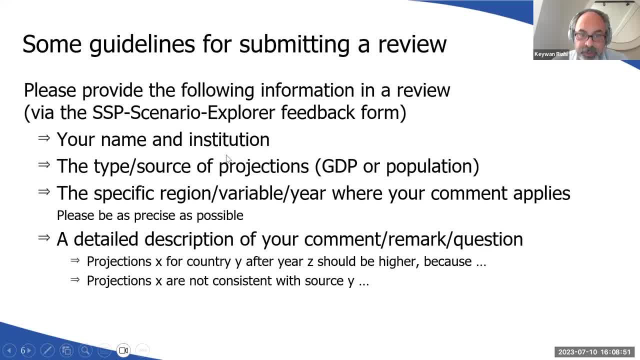 and also to provide information about which variables the comments are made on and which results. So if we were to say that you have a question in this region and here it is applied, it applies to, and then send us in the feedback place in the Scenario Explorer description. 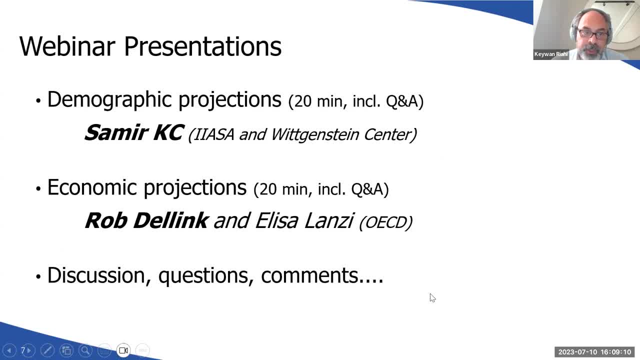 of the remark, question or comment that you might have. Already speaking, perhaps a little bit too long, I hope this was useful. We will revisit the link for where you can provide feedback at the end of the presentations and I suggest we starts with the first presentation. 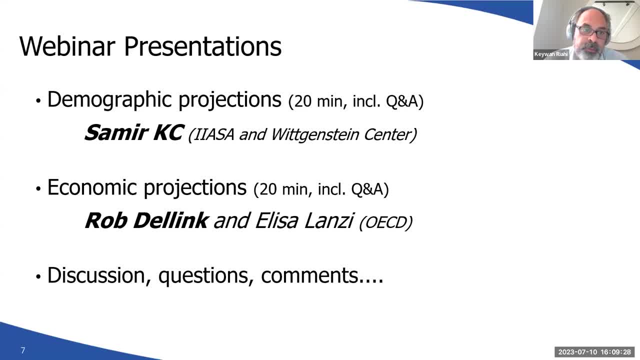 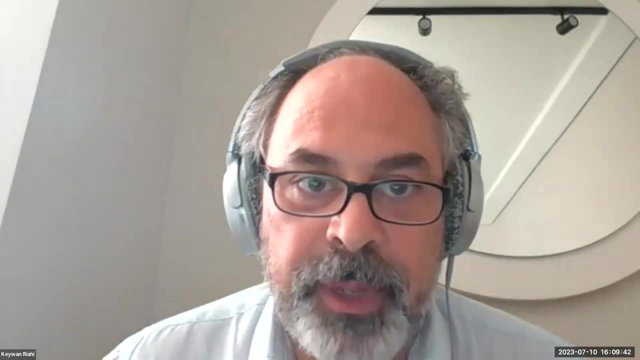 by Samir KC, who is leading the update of the demographic projections and who is at the Wittgenstein Center and IAZA. So I stop to share my slide and pass on to you, Samir. Thank you, Siobhan. 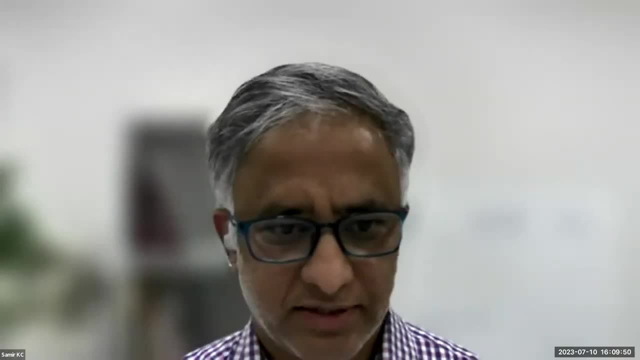 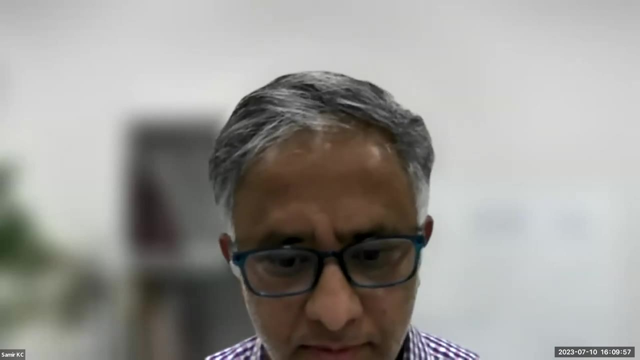 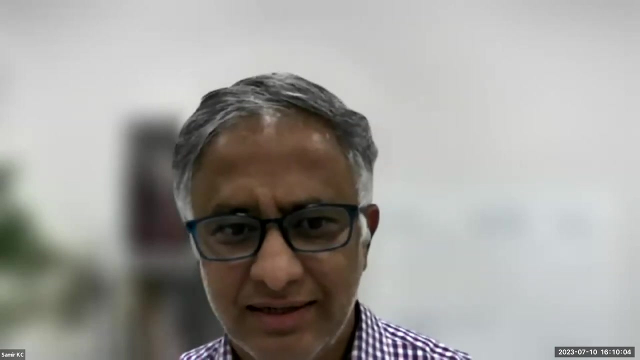 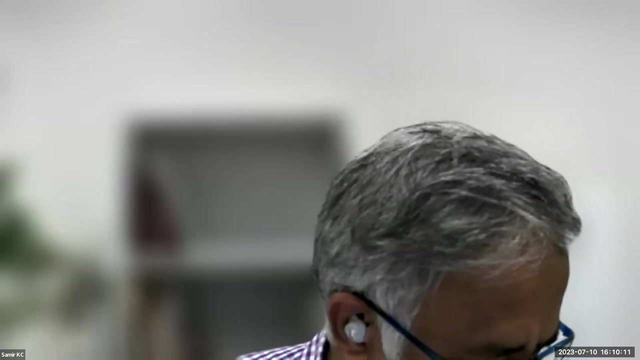 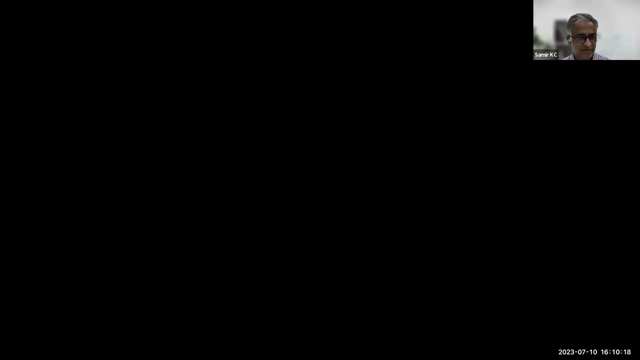 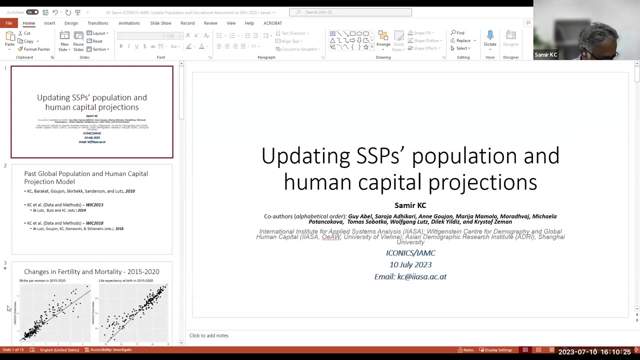 I hope you can hear me good. OK, Just a bit lost with my screen. just a second to take a side. share the screen and yes, So You see the notes. right, We can see. right now it's not the presenter mode. 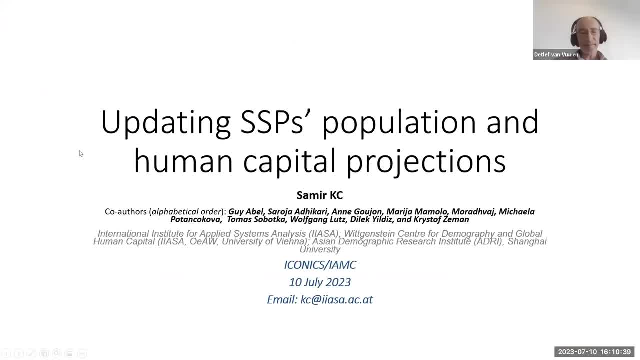 it's the other mode. I think you have to skip now. Now it's perfect, Now it's good. OK, Thank you. So, thank you very much. I just have to be looking at a different screen, so looking at the main screen. 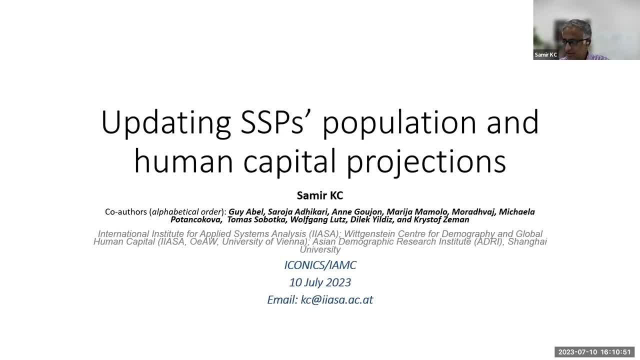 So this is a work: the updating of SSPs that look almost right now. It's not the main screen, it's the main screen. So this is a work: the updating of SSPs that look almost right now. So this is a really great work. 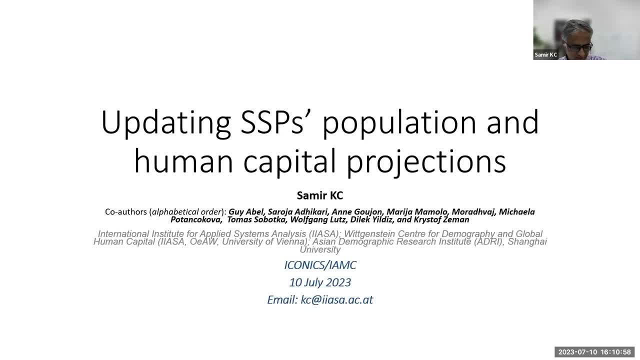 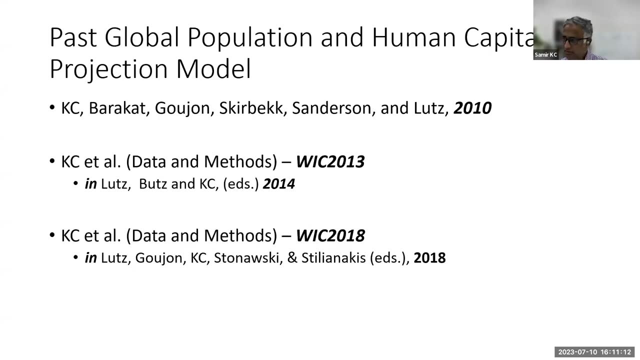 So many of these issues can be referred to whoever you work with. So if we look at the online delivery of SSPs, the amount available is not only fallible at one time, but also early in a future As of a. So we haven't talked in detail about the 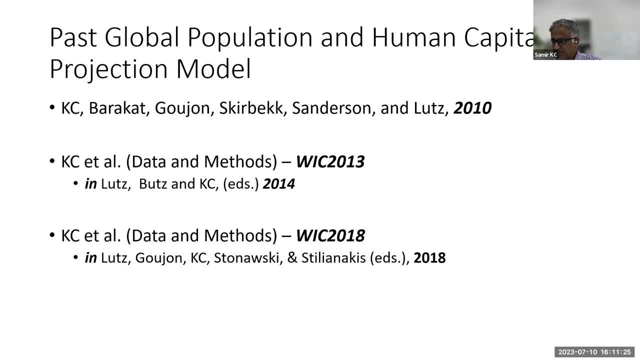 sem Preferences project at the ALGC and as a whole. we haven't talked about that kind of stuff yet, Obviously. But I think that's OK. Sorry, I will stop talking for a second. OK, All right. Bye was in 2010, and in 2013 we were doing a big project on defining the global projections. 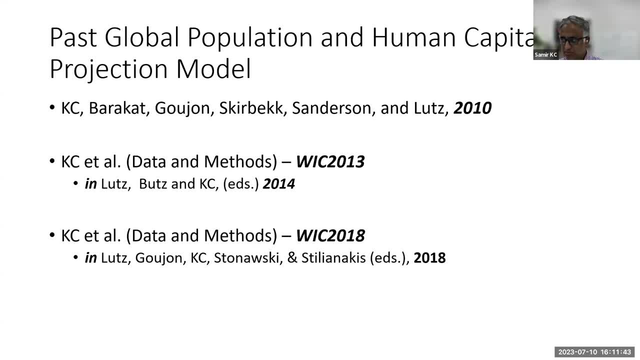 by ourselves, meaning that in 2010 we were taking lots of information from the UN about the future, but in this 2013-14, we were developing our own future demographic scenarios and during this time where we produced SSPs, and so we call it WIC 2013. so for us, for our 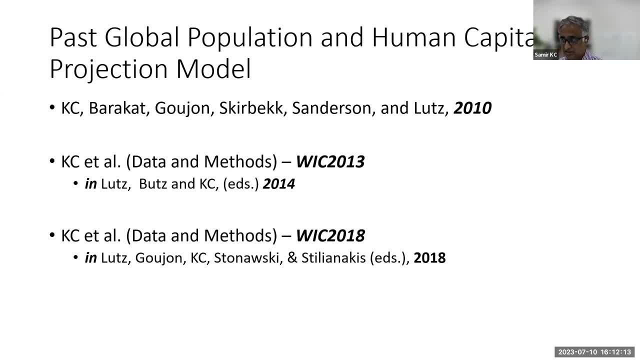 internal kind of labeling, we call it, which is time centers, 2014 projections, which is basically the first SSPs. so, while those SSPs were shared to the SSP database, we were also, you know, updating our projections: the course, reputation and human capital. and in 2018 we did update because five years for us would be quite, you know, like a significant. 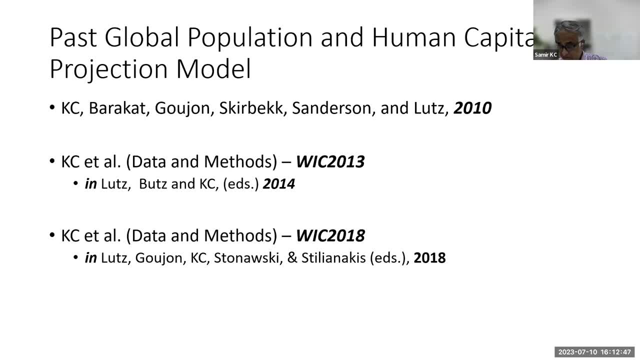 amount of time for the for this demographic changes, so we did this update in 2018. however, this was not yet brought into the SSP database, but I know that a few of the colleagues who needed SSPs they were also using this one. so now in 2013, with again the- you know from the SSP community asking us to revise it. 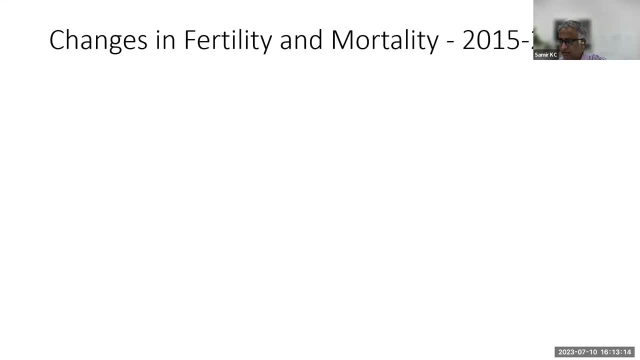 after that 10 years, we did, and we have some examples to show like what has changed since what we were thinking 10 years ago and now. so I have a few graphs. the first one: this is about the births for women as a fertility rate right. so in the x-axis you will see what we were assuming when we were projecting in 2013 or 12-13. 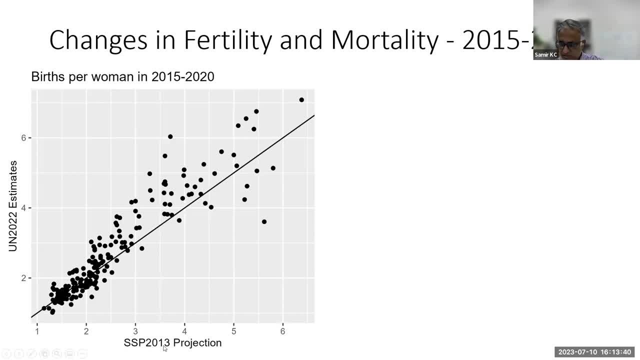 around that time, what we were thinking about what might happen in the next 10 years or so. so this is what we were thinking about in the next 10 years or so. so this is what we were thinking about in the next 10 years or so. 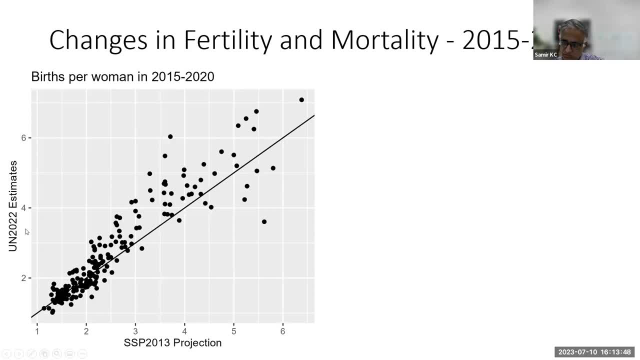 about what might happen in 2015-20. right and in the y-axis you will see the estimates from the UN. so UN kind of updates its projections every three years and what you see here is that in many areas of the world we have values are not, you know, lining up to this portfolio. 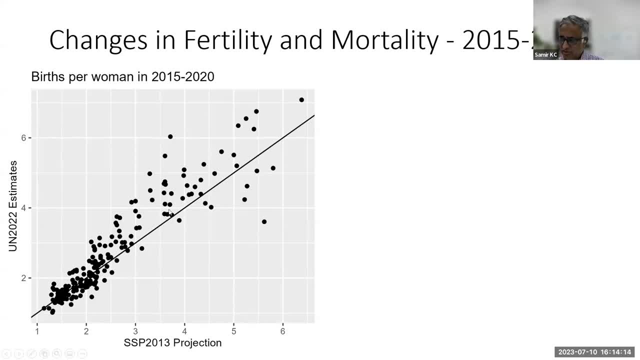 slope line. so definitely we see that in many countries. so these high fertility countries, what we were expecting. so the fertility rate didn't decline as much as we were expecting. So this is just about how things were different with what we are projecting and in the reality. And then for the life expectancy. these are the 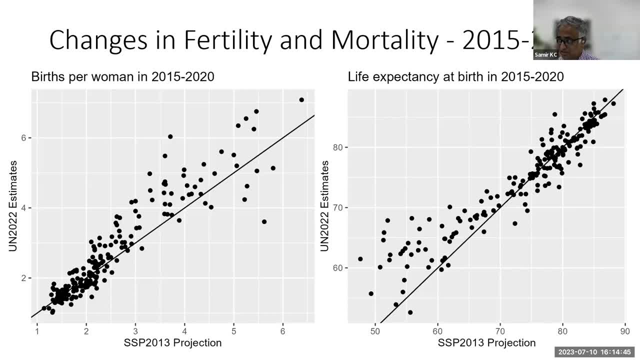 two main sources of components of population change. So life expectancy had bought in 2015-20.. So when you look at it, so here you see actually lots of positive things happening, meaning that in 2013, we were expecting certain increase in life expectancy. so there was always a positive. 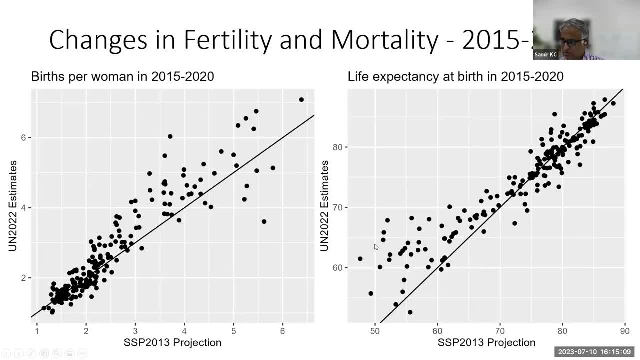 foresight there, But we found that many countries actually gained a lot of life expectancy. you know like the mortality situation became much better for many countries, especially those countries which are, you know, which have the level of life very low. We also see some of the changes here, but it's going on both. 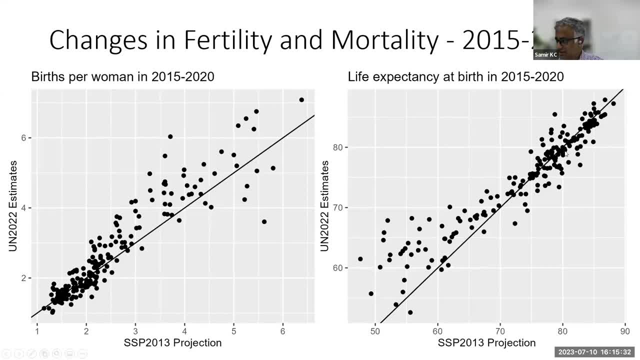 directions. So let's say, on Everest, things were fine over here on Everest, but in this part of the world- I have just put one new graph here, so I also split it into male and female- this became the gaining, like I mean the life. 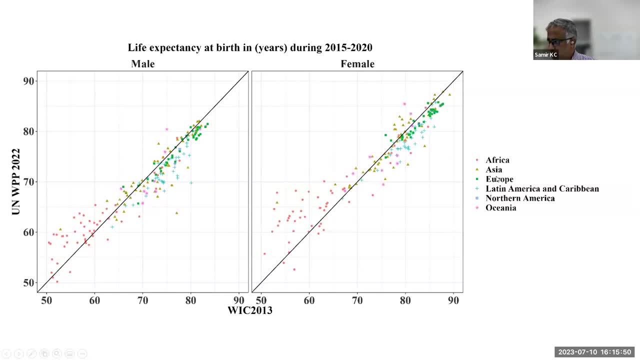 expectancy at birth and then also divided by- you know, leveled by the country- other continents, You will see that most of these countries are from Africa. and then here the positive news is like gaining the better job you know in saving children but at the same time saving 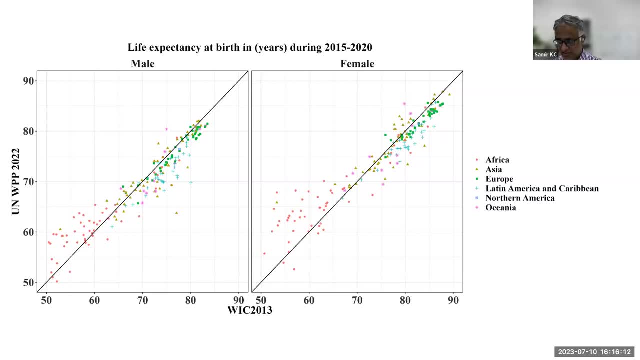 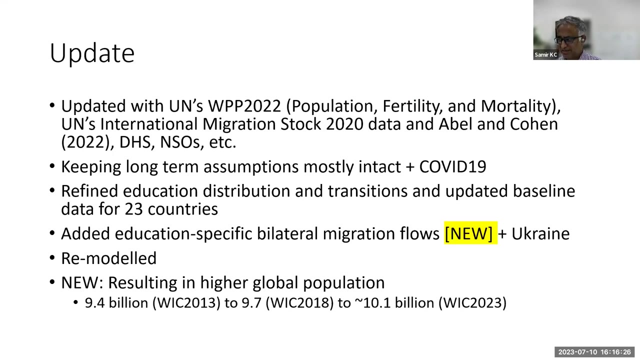 the HIV related mortality. So, basically, you see that these are very important changes, that we see significant ones, so we have to update our section. So, apart from that, just to quickly go through our main, let's say, highlight of this version, we have: 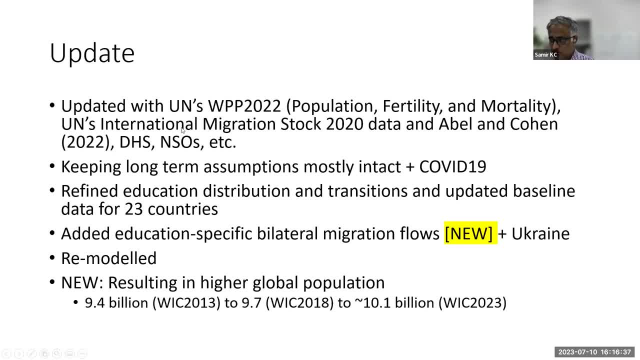 done a lot of work this time to improve our migration assumption, So we have basically used the information from the UN migration stock data, which provides you for a given country. it tells you, like, how many people are there, by age, sex and by country of birth. 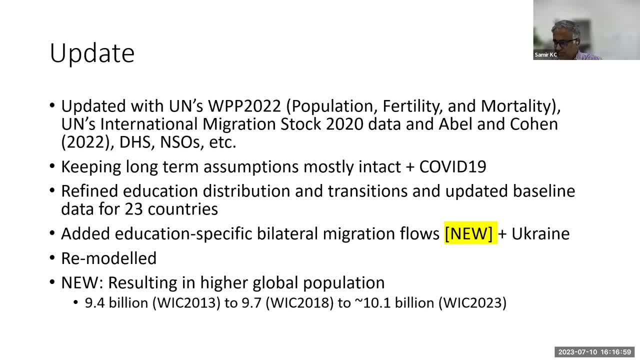 Other citizens. it says There was a confusion there. So anyway, we will know it like from where people, we will know the people's population's origin, And those data are kind of used like every five years, I think they get the population and then we can also use it here. So 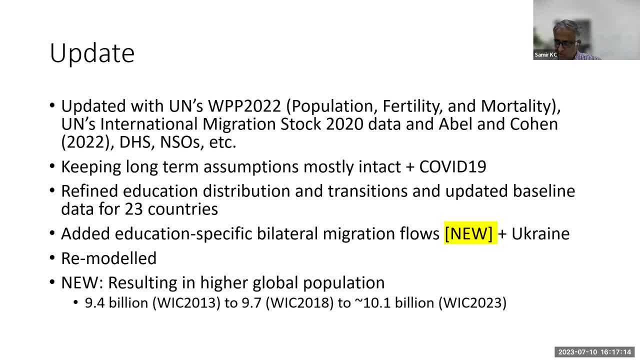 I think they provide every five-year time step, and we used to calculate the migration rates in the last five years, So we do five-year step prediction. So, and then for the mortality, with increased value, of the change in the value of life expectancy at birth. 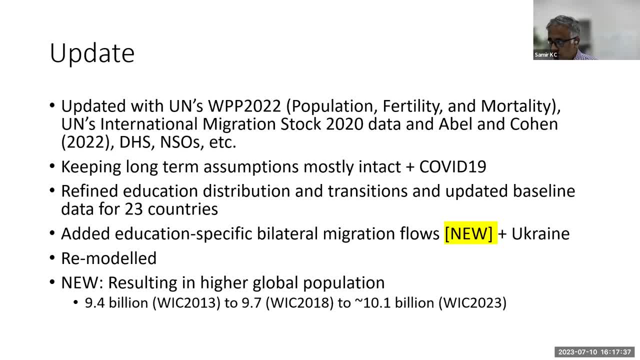 we go into the future And then we also have to bring the COVID-19 impact, which was mostly impacting the 2020-2025 deaths, Since it's our season, but as UN does it by age and sex, we do it by age, sex and level of education. 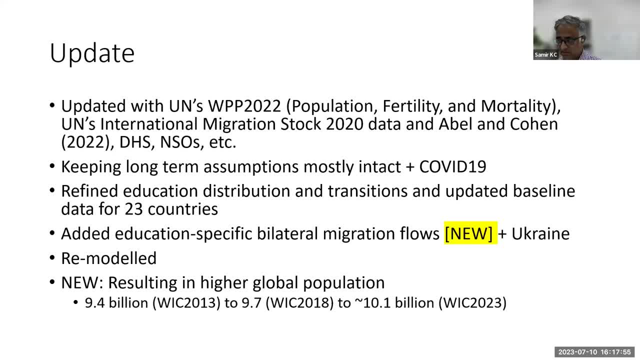 So we were also updating our base structure by age, sex and education. So there were lots of checks. I think in 2021 round of census we provide us more data in the future, So maybe, yeah, in the next another five years. 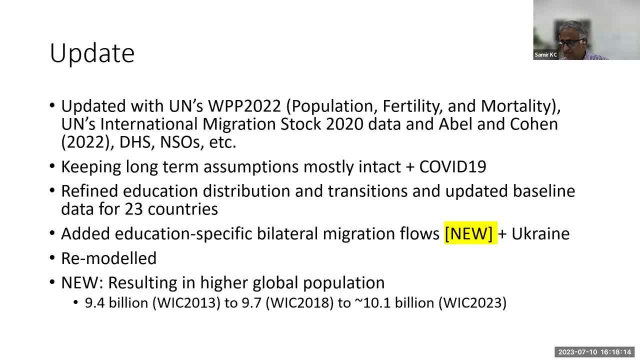 if we do, we will have much better data of the education distribution, But still like this is much better than what we had in the past. And then our, basically the highlight over here is this: education specific bilateral migration flows. So previously we were, our migration flows were, let's say, 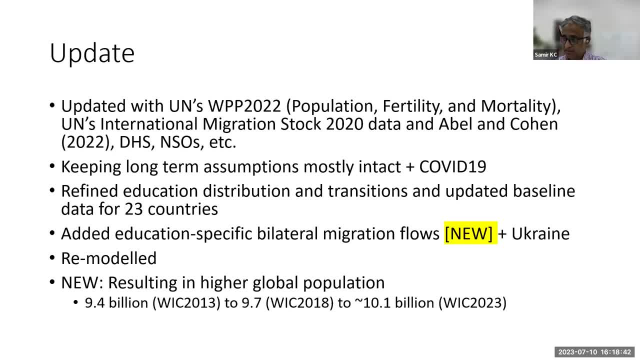 education specific. It was more than gender specific assumption, but this time we have worked a lot with several, particularly our work and how this education specific migration flows were estimated And then we brought it into our position. So this is a new and there are smaller things happening. 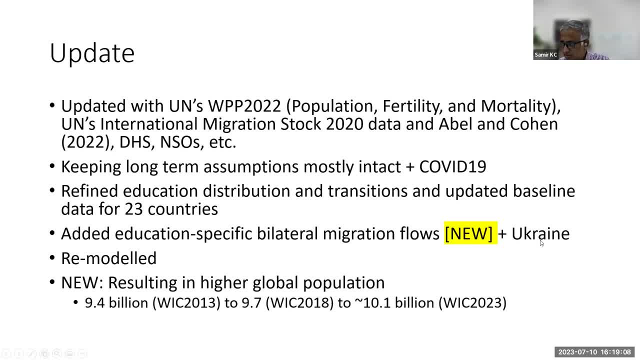 And definitely couldn't ignore Ukraine, migration, the refugees flows from Ukraine, and how we also work, that we affect a number of countries for which we have been working with the GRC in Europe, the Joint Research Commission of European Union. So we had a joint paper there and we are using there what we have produced in there. 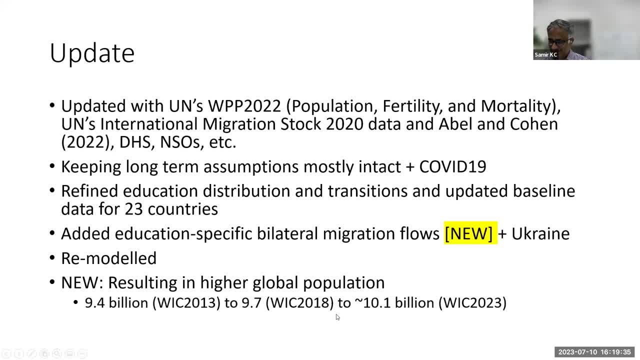 So, basically, the big results I will say is that in WIC 2013, our first SSPs, we had 9.4 billion as our projection was showing that war would peak at 9.4 billion, which now will be peaking at 10.1 billion. And we are now, you know, trying to, we are writing a paper. 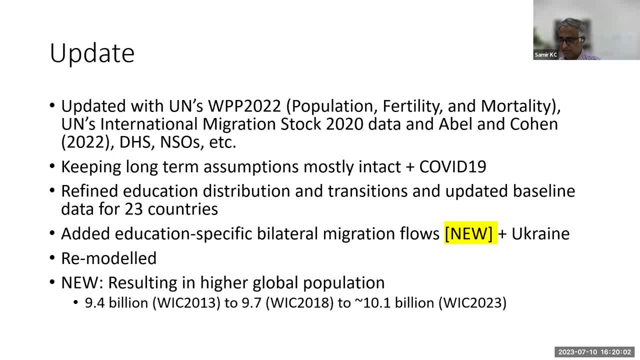 just a working paper to explain exactly why this happened, But we know it's mostly because the children, the children were saved. a lot of children were saved and you know, like when they go further they would be mothers, and you know there is. 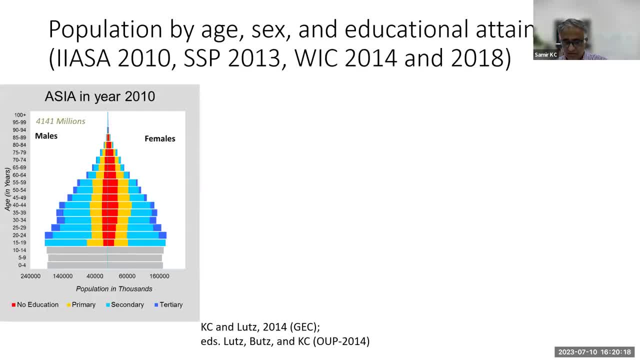 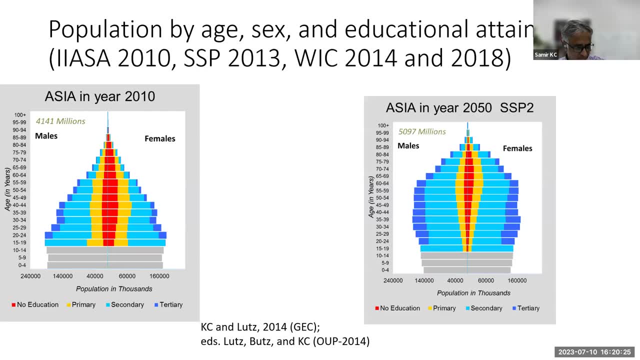 an impact, many impact of that. I don't know how much time I have, but let's quickly go through a few results now. And you know, our approach is always about, you know, like we have this population and we look at the population not only by age. 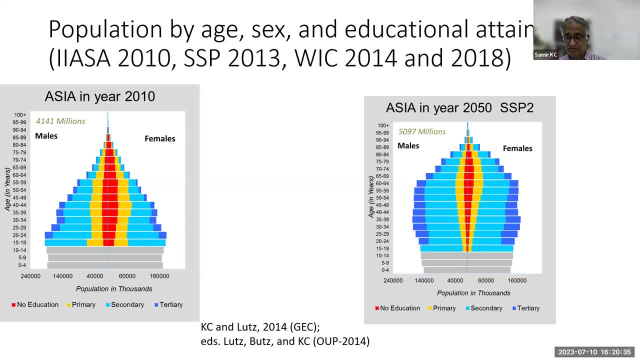 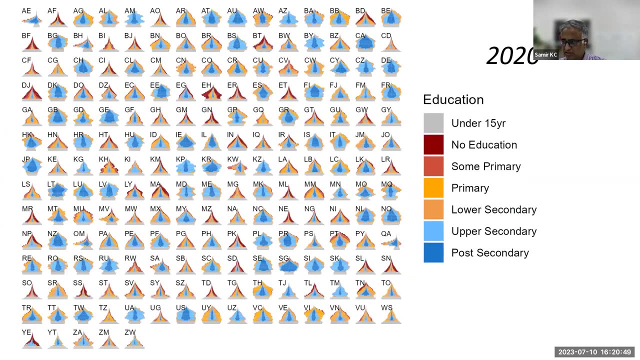 sex. This is a traditionally done by this pyramid, you know, but we put colors to it So it can also give a kind of quality of population. And yeah, so this is like 2020, so just to make it like 200 countries of the world here by age, sex and level of education. 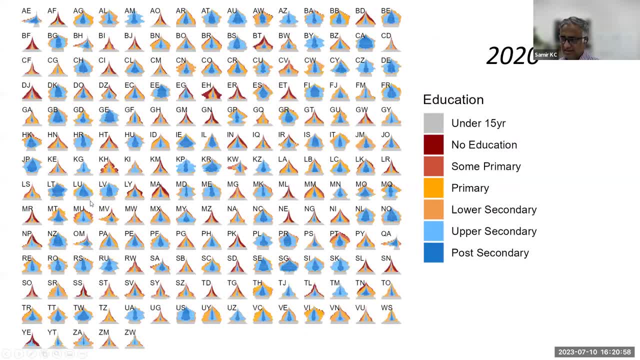 basically this kind of pyramid here over here, And this is what we project into the future. So you see that there are different shapes of the countries. there are lots of colors, more blue colors showing that this country is good in terms of human capital, but there are countries like 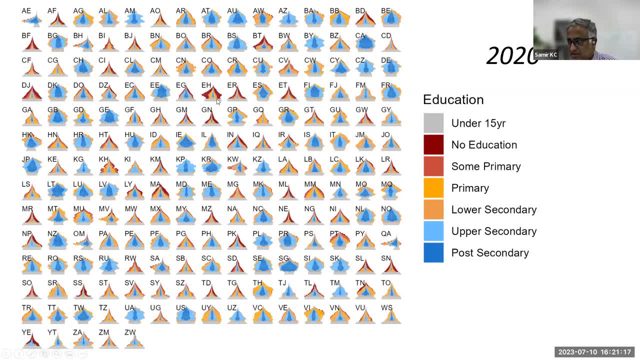 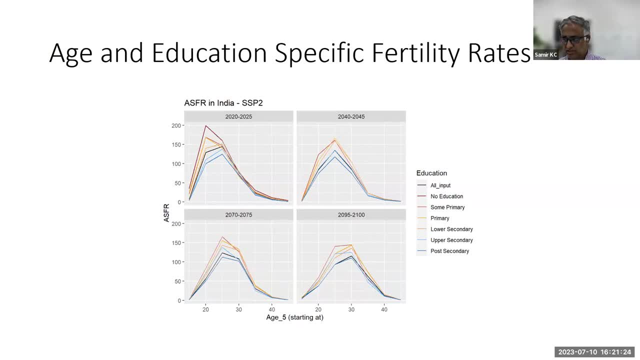 here where you see lots of weight, which kind of represents that the education level is quite low. and then I have few slides just to show, like what goes in our predictions, that we have to calculate the age-specific fertility rates. then we have the age and sex and education. 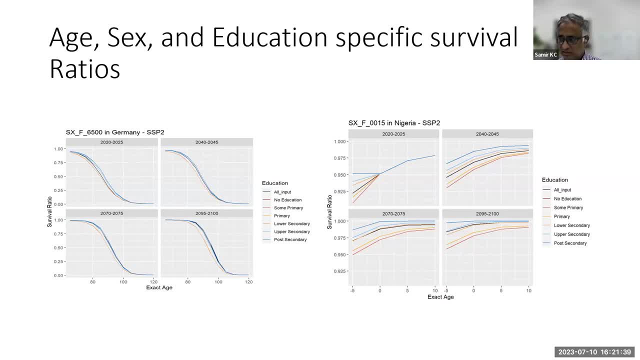 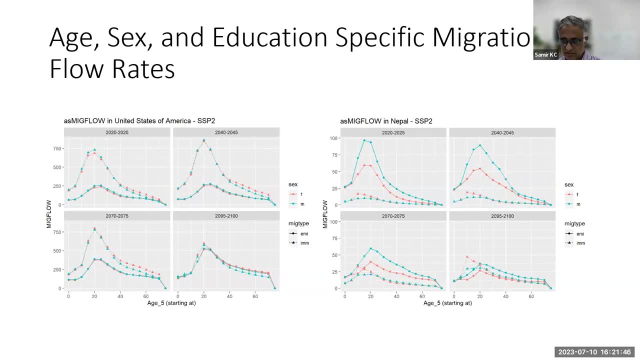 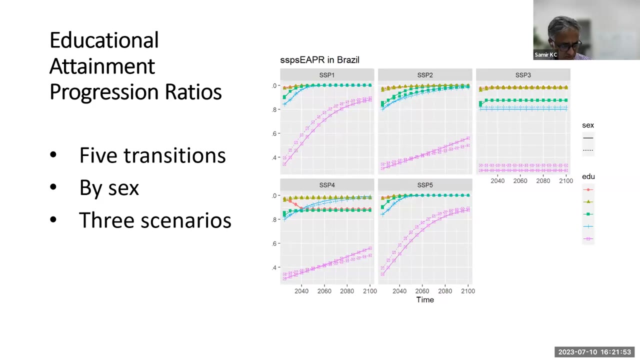 specific survival ratios. so that is the mortality part. and then we have the age, sex, education, specific migration, close rates. so these are from estimates, and then we have to do the projection and then finally the educational attainment progression ratios. So there are basically 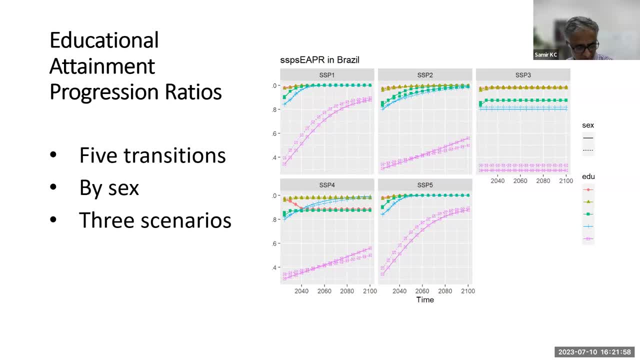 four sets of levels, The transitions, or you know, like actions happening in our model, the dynamics, and for different SSPs, then we have to define different. you know, the narratives of the SSPs are quantified. so when you quantify them, and for example in this educational one, 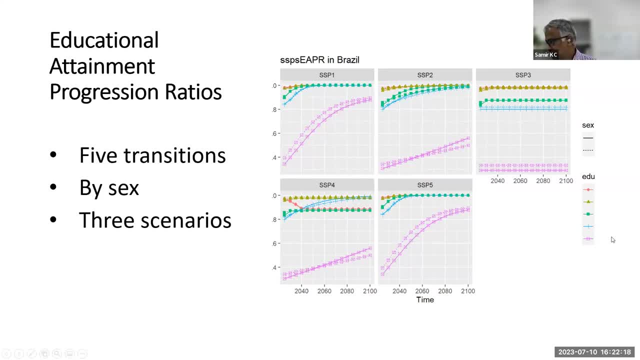 you will see that SSP one. so this is for the sorry, this part is missing. but this one, these blue ones, are for the post-secondary transitions and in the SSP two, which is our medium time, the medium scenario we have, like this kind of like. 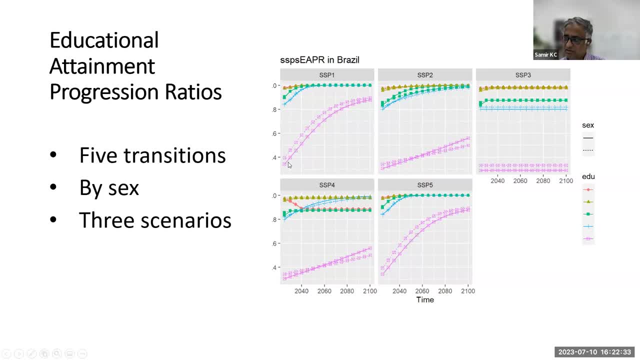 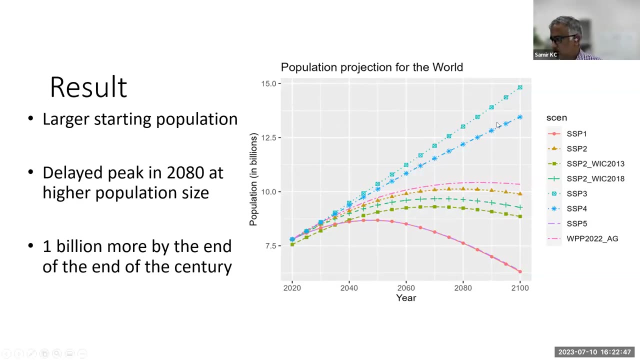 how the post-secondary transition would continue, whereas in our SSP one this would be quite faster. So this is how we. you know just a glimpse of what is there, what we have So, and as a result, so almost to find a slide here. so I have put lots of data. 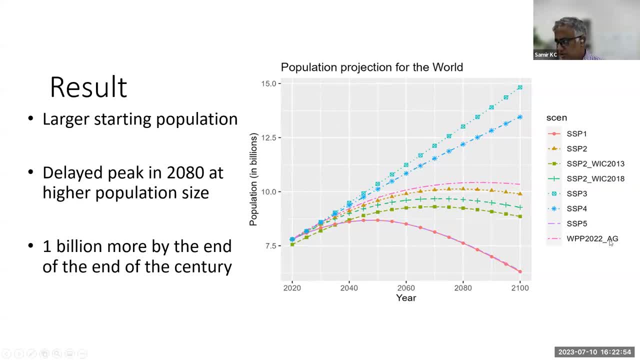 lines here. but basically there is this WPP 2022, this is the UN prediction. over here They are peaking around 10.5 billion by 2085 or so. They used to go to 11 billion and even more than that in the past in some of them, but now they are also coming down. 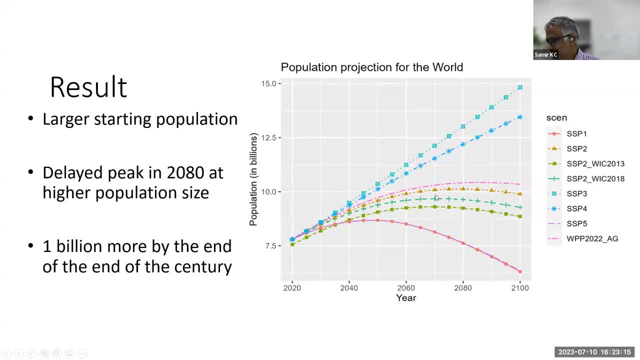 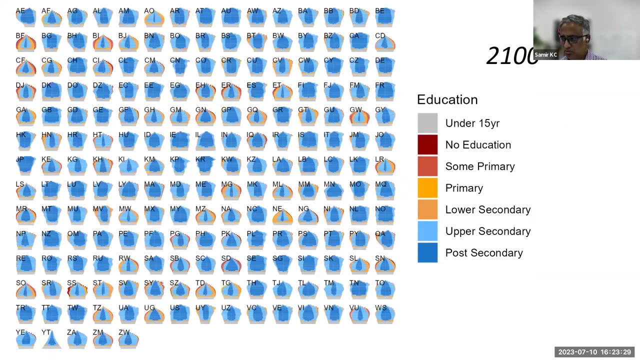 And ours were going up there. So this is our new SSP2 at the moment and I have put a few other SSPs from our past year. So basically, we are going, going up and then we have a different, other SSP scenario And this is our result for 2100 SSP2.. So it was trying to impress. 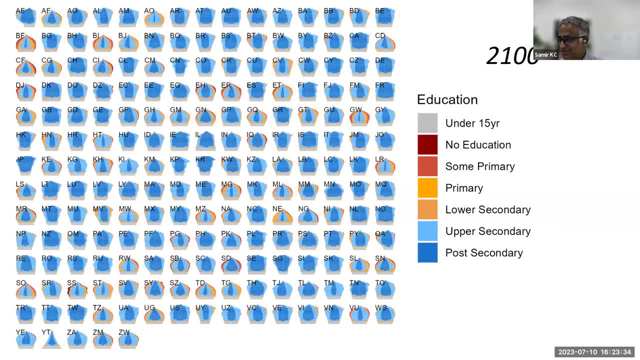 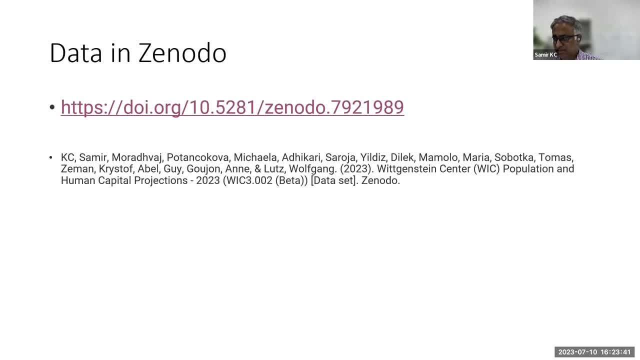 like how much beautiful it is our work here. And then all this data at the moment are shared with Zenodo, So at the moment we haven't made it public, but anybody can request for sharing the data. And finally, if I add this, So this is, this is our Zenodo, and so far we already see more. 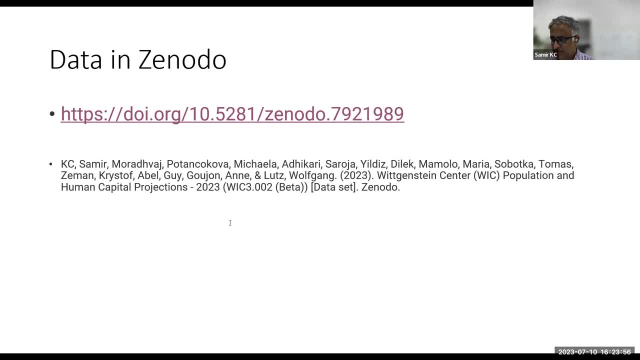 than one thousand downloads there, But again, as Jaywan said, so this, this data, I mean you have lots of like excel files and also you will see lots of these graphics that you know for the baby. I don't know you can go beyond what we will be providing you for the validation of reviewing. 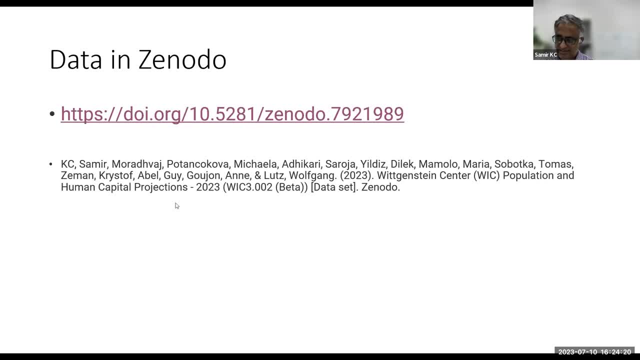 There could be lots of this kind of graphs, that you have a lot of detailed graphs to see. Yeah, and just say like, if you are not satisfied with you, want to review in depth, feel free to come here to do that as well. So I'll stop here, Jaywan. Yeah, thank you. thank you, Samir, particularly. 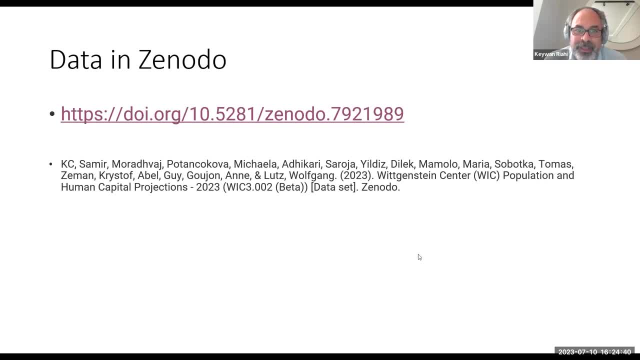 also for staying so well in time, Just for clarity and also for because this data is available in two different sites. So if you, if you want, if you're interested in really all the details of the data, this Zenodo link is the way to go, and, and, and, so basically to download a lot of additional and. 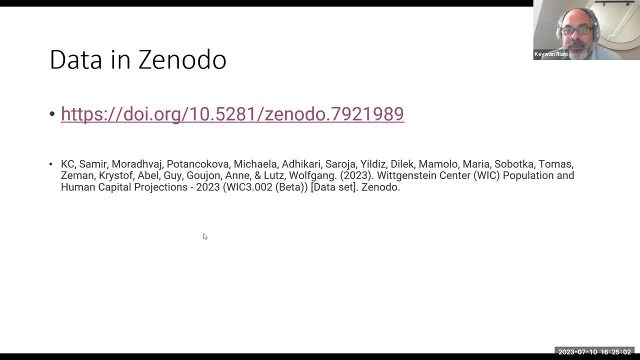 detailed information. The site where the, which is open for review and where we would collect your feedback, is the one that I showed at the beginning and will be the same data that is available on both sides, But but the review site is slightly different. So for the current 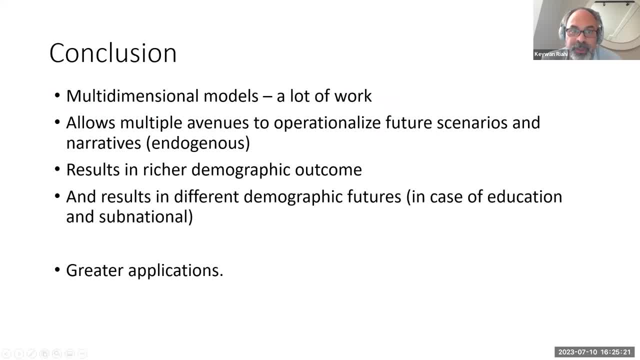 moderation. I will pass on to Detlef. Detlef von Buren for PBL. Detlef, please take over. Thank you very much. Thank you very much, And we still have five minutes because you were so nicely in time. So there's one first question for you, Samir. 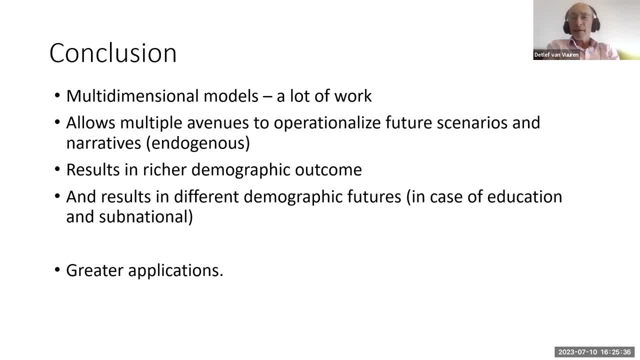 from Karen Meeseman- I think I can read it out, which is: can you please provide the reference used for the migration and refugees flows? Yeah, sure I will. later I will put that reference in the chat. It's actually from the JRC. 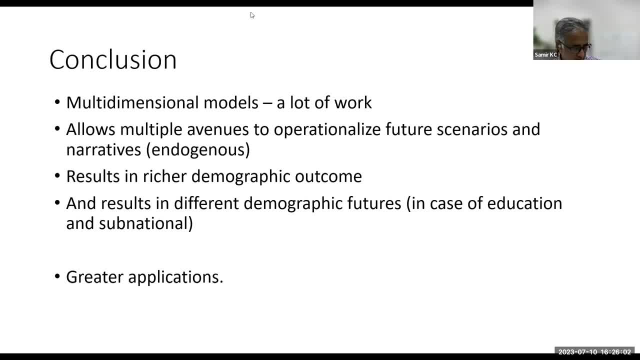 report. I will, I will do that, yeah, And and we would like to have clarifying questions at the moment. So, for people that have clarifying questions for Samir, feel free to raise your hand or type them into the Q&A. In the meanwhile, there is one clarifying question for you, Kaywan. 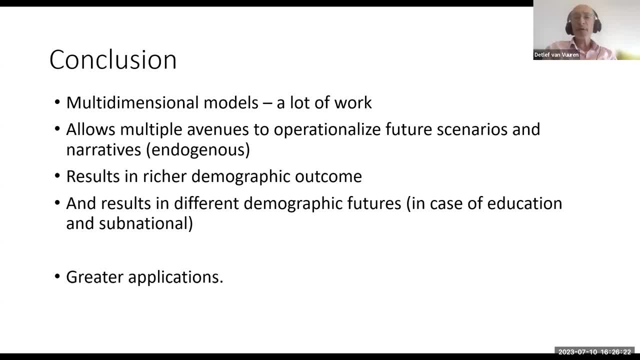 which is from Jonathan Doolman. Will it be possible in the Scenario Explorer to compare the updated SCP data with the older data? Yeah, this is a very good idea. So far we did not. we wanted to display particularly, of course, the new projections. 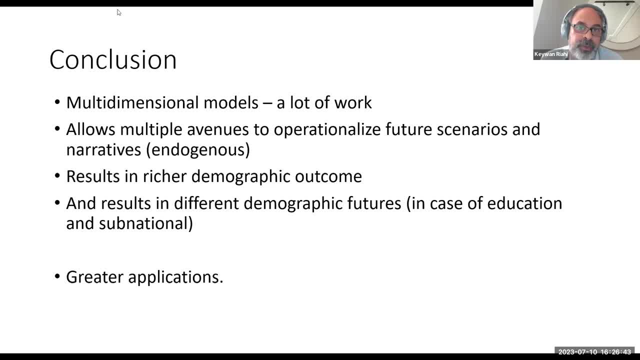 So let us discuss this internally. Perhaps we will add it so that you have a reference point and also, visually, can see whether perhaps the updates have resulted in the biggest, biggest changes. I think that's an that's, that would that's. uh, we will make an effort to provide both data, but in a way that you don't. 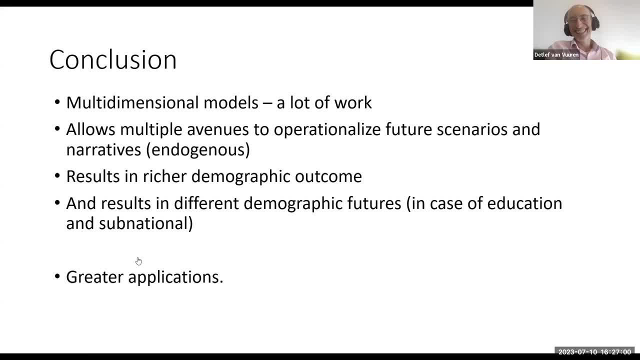 comment accidentally on the old data. so we really we need, we need to find a way that that that you can clearly distinguish between old and new. but we should. that should be possible, great friends. any questions still for somebody? let's see that marian has. is there no difference between ssp1? 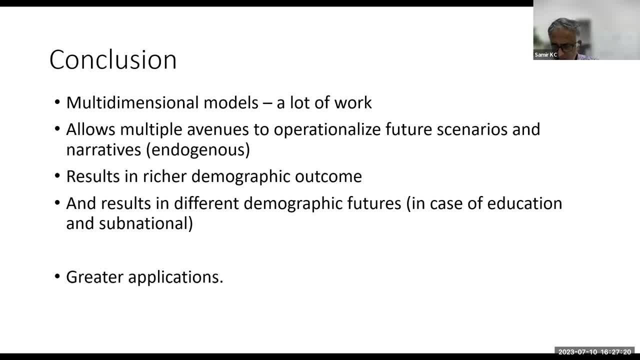 and ss 35. so my answer is that when you put it at the global level, there is not much difference, but when you look at the country levels, uh, there there are difference, especially, uh, i think uh, in developed countries. yeah, because migration, migration is one of the key component there. so, whatever, there is a big migration flows happening. 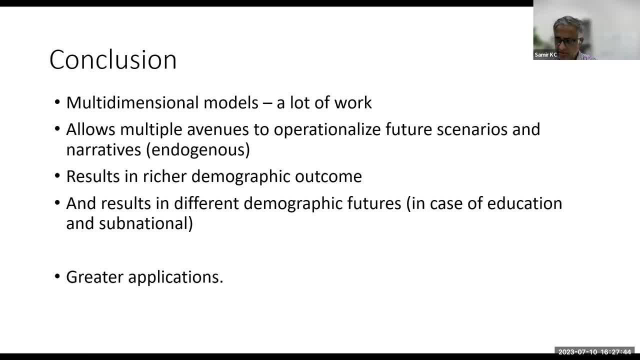 versus p1 and ssp 5 will have differences. and then again you can see this: uh all the data crabSorry is guest club. that horse evolved- put it on to some of the narcissistic languagebrushes of the test- is larger, but there is this big migrationğ that horse workflows happening. the ss p1 and ss p5 will have differences, and then again you can see this: uh all. 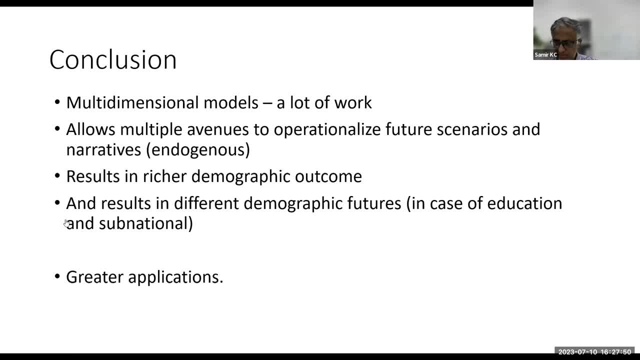 these changes in this, this pop, like in the gennado, have created. this file is called pop and for every sub reasons you will find, you will find something like this. if my screen is still shared, you will see that in canada, how the different ssp1 and ssp, even ssp5. 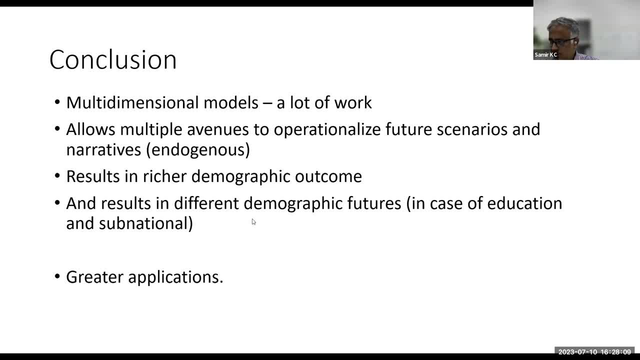 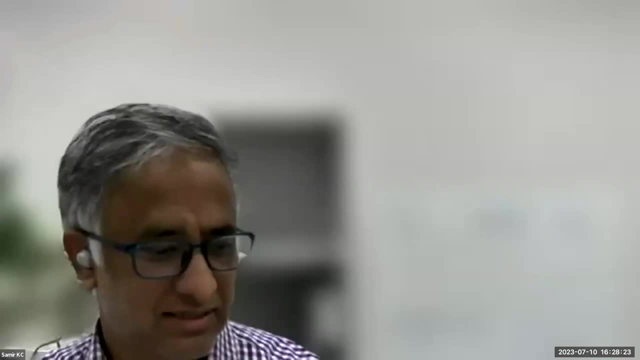 and ssp1 will have a different population and it's mostly driven by the migration. so somehow we're still on your conclusion slide, i think. oh sorry, but uh, no, but you could we if? if that's possible, it would be great if you can also share your slides, samir. yeah, for people, and there's one. 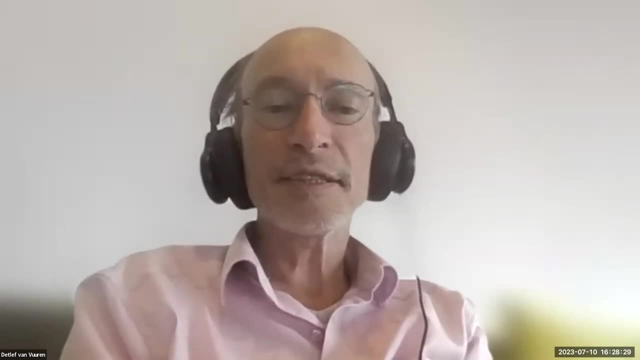 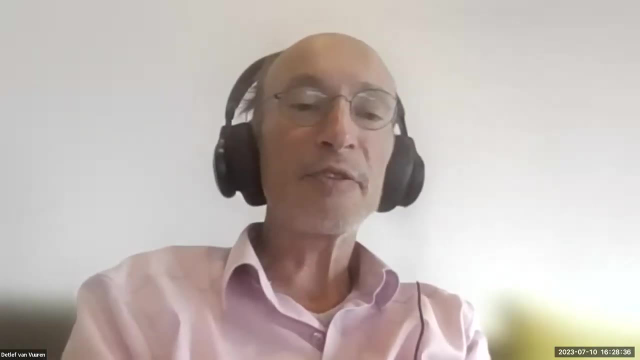 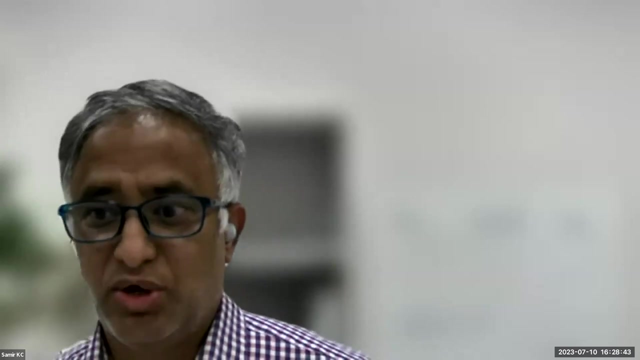 last question, and then i propose to go to rob's uh presentation, which from uh mohammed irfan, and you can see it yourself. i think, samir, i can read it out. yeah, yeah, you know, i say i can read. so this is like: does the utfc data cover the entire world for bilateral migration? like that? no, no. 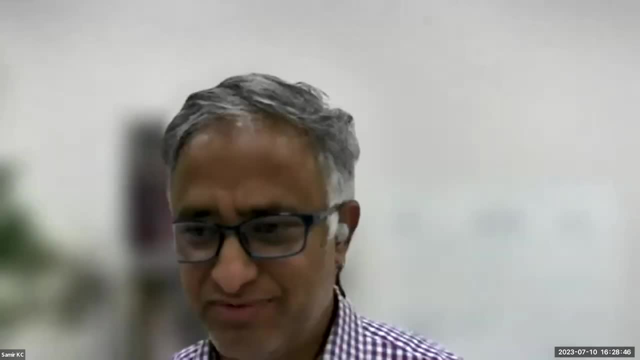 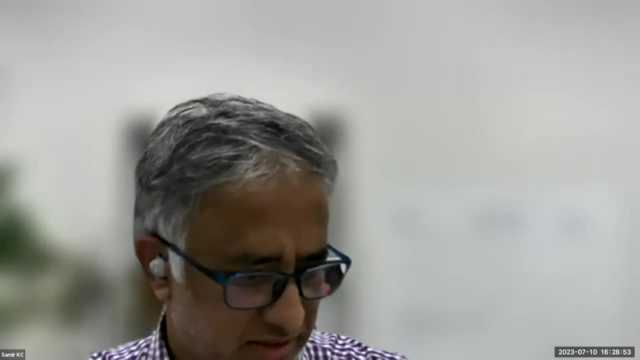 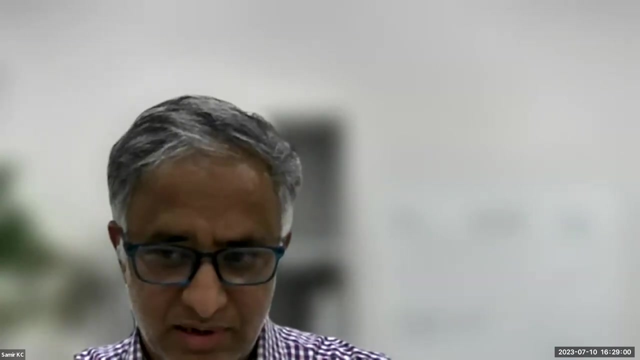 that educational attainment is ours, so it's not coming from the jrc, so jrc data is only for the ukraine. uh migration, okay, like refugee migration, uh, but this uh, uh, uh educational attainment migration is from us, so we are actually will be uh coming uh, yeah, you will see all the results. 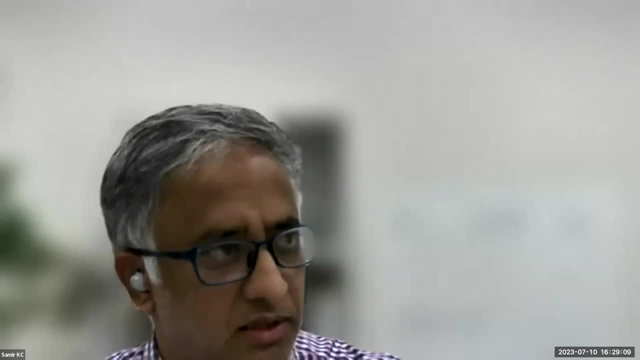 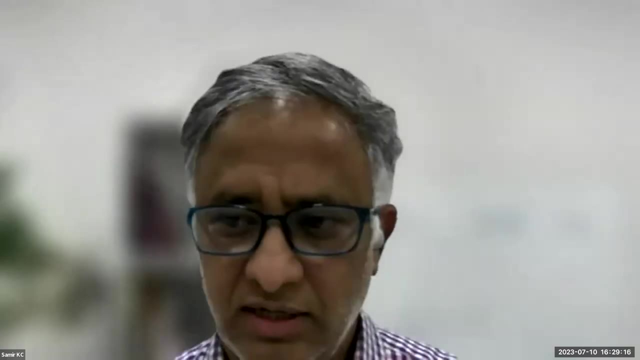 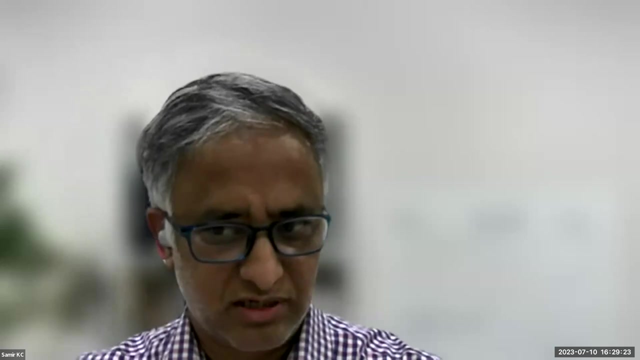 in the data, so the reference will be uh of that would be one of our colleague, rilek, who's going to have a working paper at yasa very soon, and then uh, and then in in the projection. so she provides the estimates of the past and then then i convert it into the future scenario. so 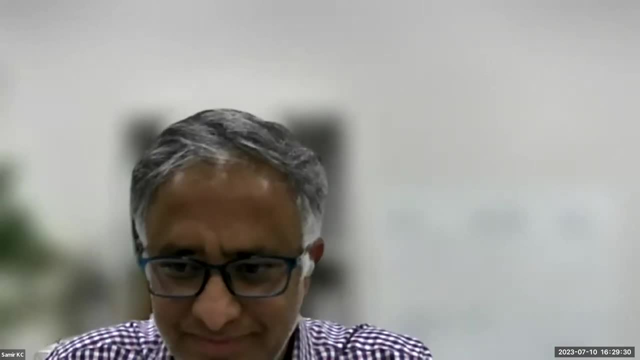 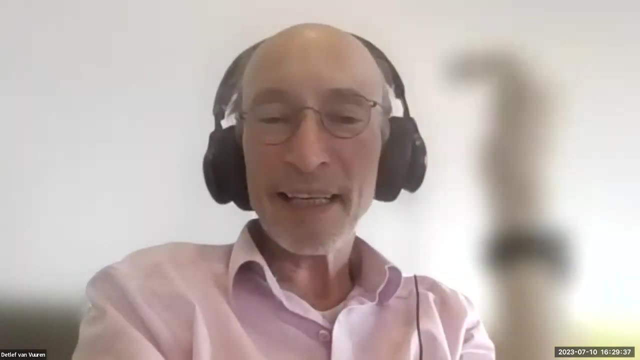 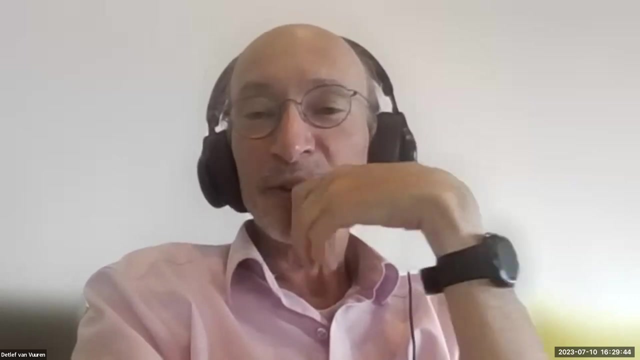 maybe in a few weeks you will have this thing. okay, perfect, yeah, so i would suppose that we now continue with the second presentation and we have this primary data, not only population data, but also economic data, and, uh, so we have the data and we have the project data that is coming from the ucd, and then 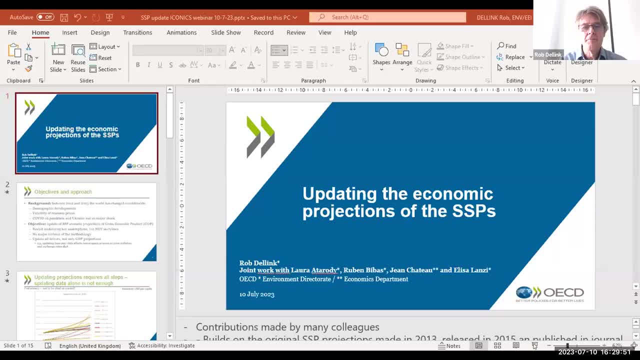 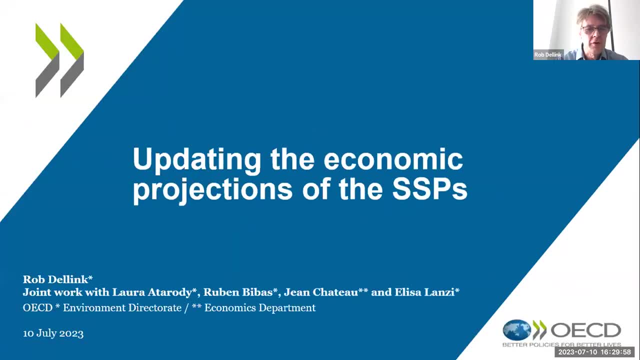 the data from the ucd and then the data directly comes to the government. so again, that's the ucd planning of the ocd will talk us through the new projections there. so the floor is yours. thank you, detlef. um, i'm trying to share my screen now. 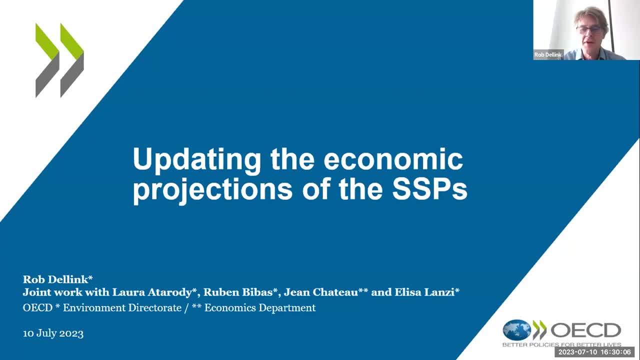 there we go. so this is joint work with a number of colleagues. let me clarify up front: these are projections by ocd staff using ocd tools. but these are not ocd projections. these are not is for us kind of a hobby project on the side. So don't blame our governments when we make mistakes. 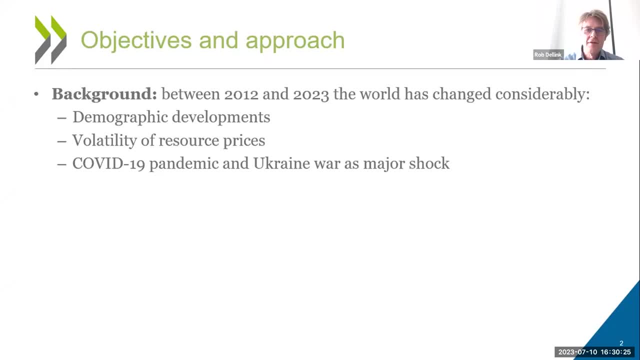 So the objectives are that when we did the original analysis, that was like more than 10 years ago. we've seen changes in demographic developments, as Samir already said. We also saw volatility in resource prices actually happening already in 2015-2016. that had a significant influence. 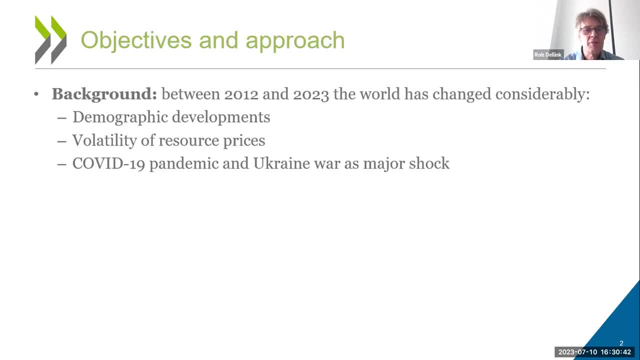 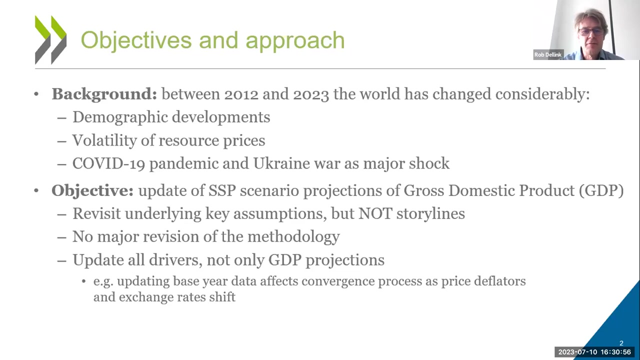 on GDP projections in Africa, for example, And of course there was the COVID-19 pandemic and the Ukraine war as a major shock in recent years that have also affected economic projections. So the objective of our work now is to update the SSP scenario projections in line with what Kaywan said. We revisit the underlying key assumptions. 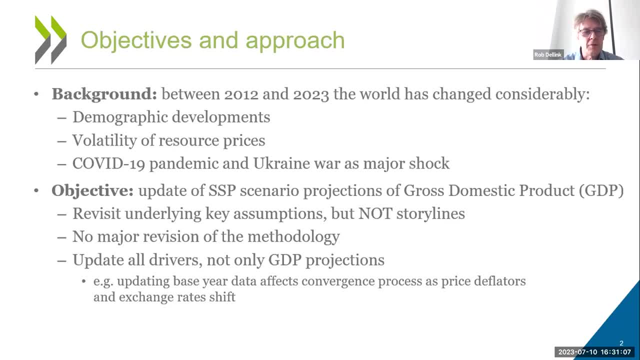 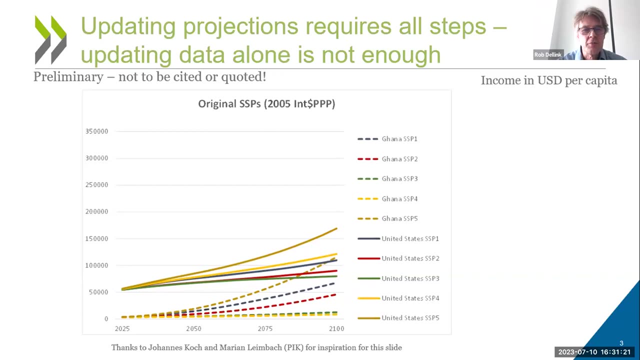 but not the storylines, and we don't make major revisions to the methodology. The thing is that we want that. what we're doing is we update all the drivers of the model and not only the GDP projections, and I can give you an example. These are projections, the original. 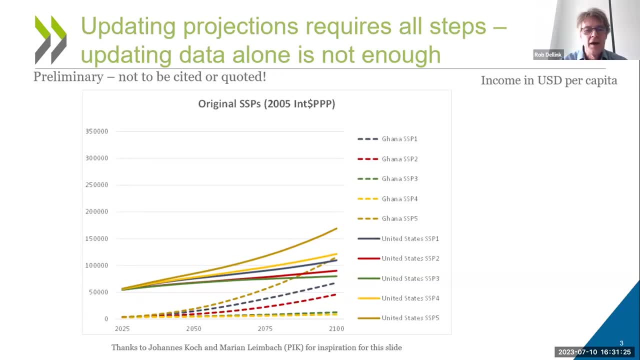 projections for the United States and Ghana. And then, when we started our updates, the first thing we did is we converted the SSPs to 2017 international PPP exchange rates, which is the latest one that's available from the International PPP Exchange Index. This is like a very basic 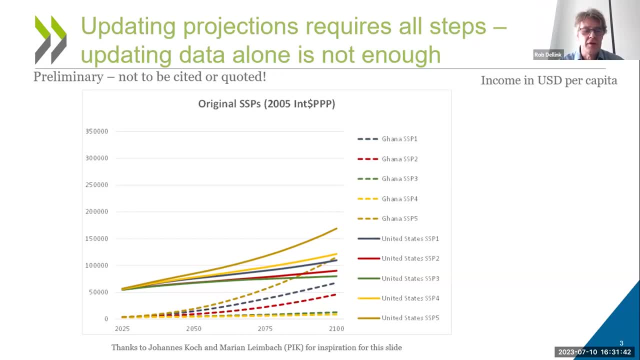 comparison exercise and if you and also national statistics have changed, the definition of gdp basically has been revised. they've included more categories of economic activities in gdp. so if you just update only the information that we have to new exchange rates and historical data for the 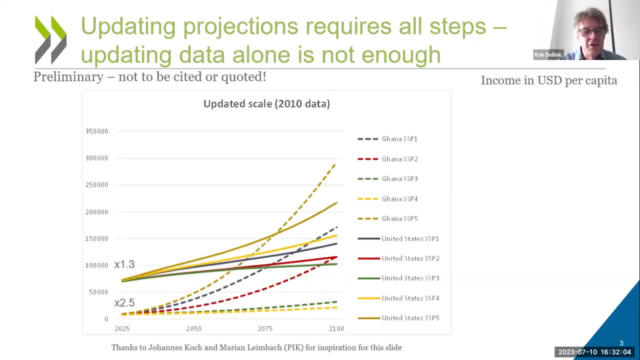 year 2010, you will see that that gives you a 2.5 times increase in the gdp level- gdp per capita level in ghana- and a 1.3 times increase in gdp per capita level in the us. so if you would, 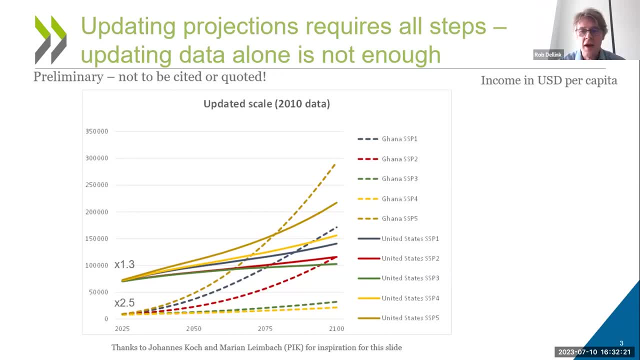 apply that to the original growth rates, as we had in the ssp projections, you would have a much smaller difference to start with between ghana and the us and then if you have a high growth scenario, such as ssp4 five, you could see in the brown lines that actually you end up in a situation where ghana 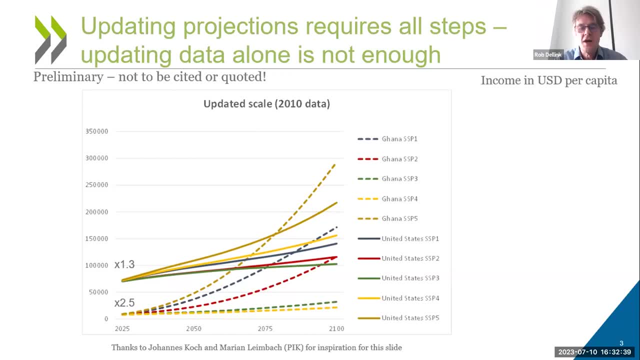 is richer than the us by the end of the century. so basically, just updating data and not updating any of the underlying drivers can lead to significant problems in your projections. so if you then include all the updated data to 2020, the idea is already. the difference is already. 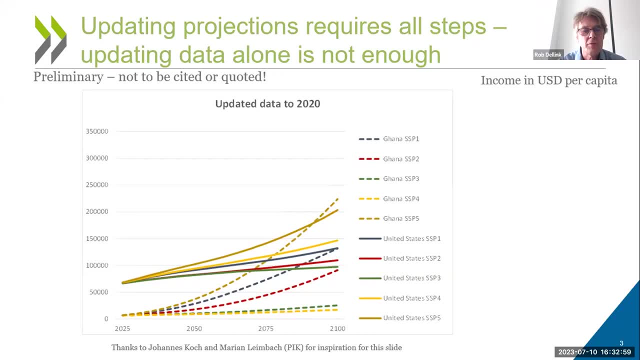 much smaller because growth in ghana has been lower than what we had projected and in the US had been roughly on target from what we projected. So you get something that is already closer. But if you do the whole new projections with all the drivers and look again at how far 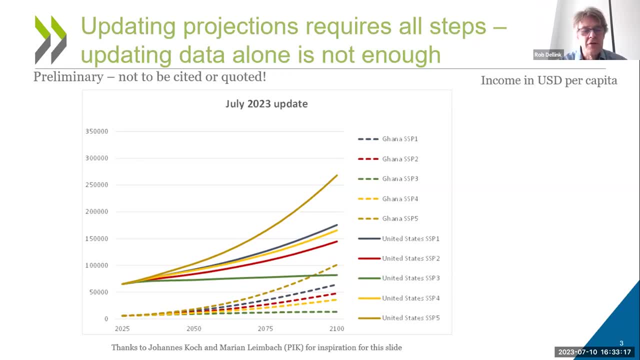 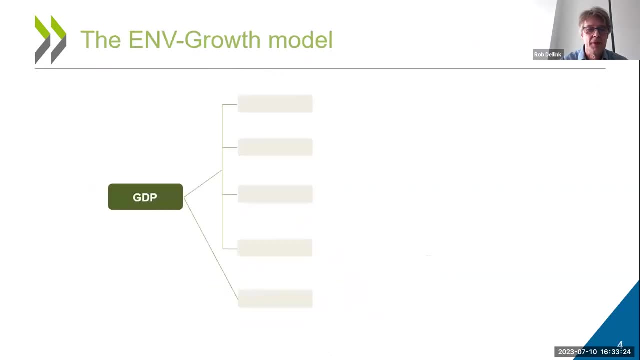 countries are from their frontier, et cetera. so you redo the whole analysis, you get the new results, which are much more in line with what we had originally. So the modeling tool that we use is called the ENV growth model and has a number of drivers. First one is total factor productivity. 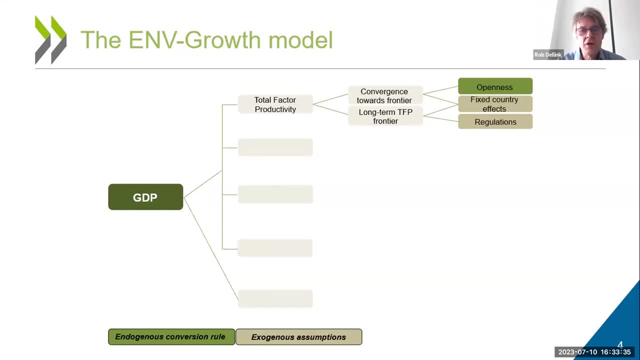 Basically, this is technology, as we call it, And there we distinguish between two different elements. One is: every country is converging towards its country-specific frontier of how good technology might be. You can think of this as countries looking at other countries and seeing. 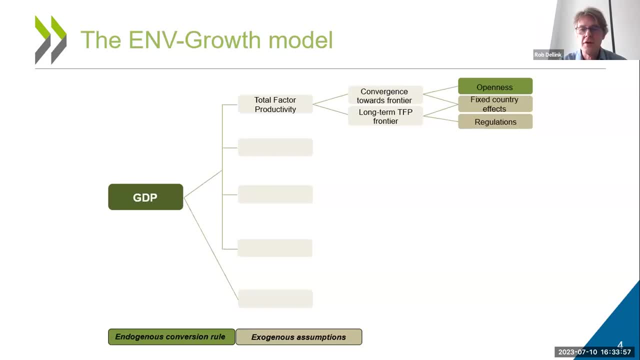 that other countries are better at programmed technology producing certain commodities, so they could also catch up and produce those commodities more efficiently. So this convergence towards the frontier depends on a number of things- fixed country effects among them, but also it depends on trade openness. Basically, if you're 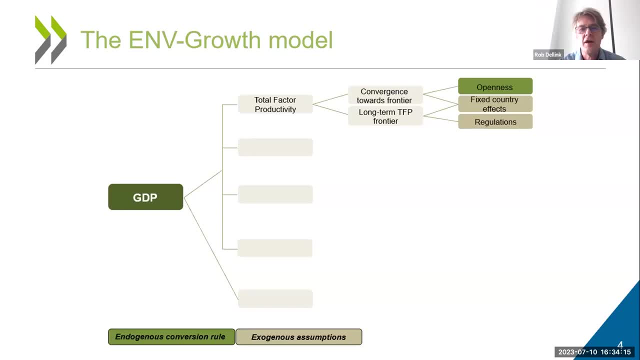 more closely connected to the international community with trade, you have better access to the technologies of other countries, and then that will speed up your convergence towards your frontier. But this frontier itself, this long-term TFP frontier, that itself is changing over time. 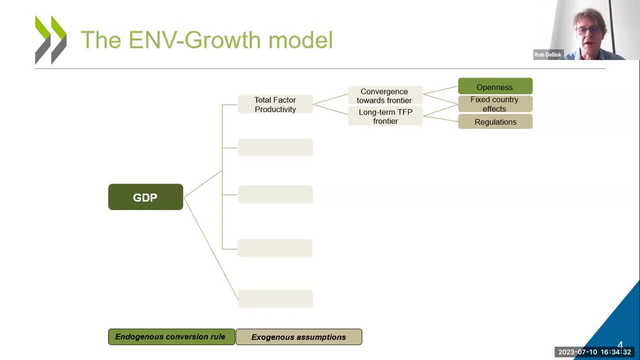 So it is country-specific, but it's also time-specific, And this depends on an econometric equation for most countries and some convergence assumptions for other countries, and it depends on how far countries are basically and how they move along, And this is also a key parameter. 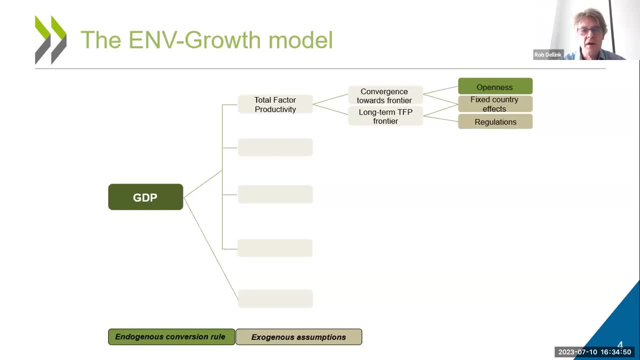 in our modeling to differentiate across the SSPs in how fast this long-term TFP frontier moves. So the second one is physical capital, which is basically investment increases your capital stock and then depreciation takes some of it away and physical capital grows. We start off. 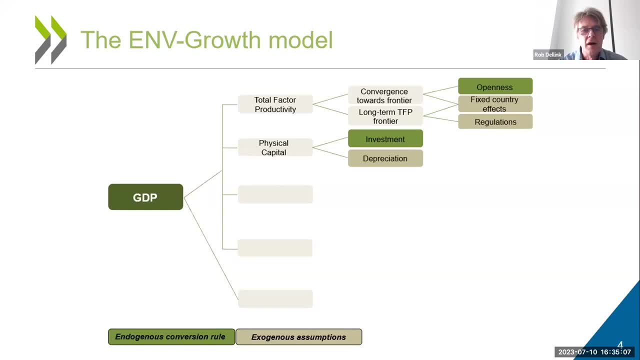 with a situation where physical capital is basically suboptimal. There's not enough physical capital used in most of our economies and therefore the physical capital stock grows over time and contributes to GDP per capita growth. Now for labor. we have two aspects. One is human. 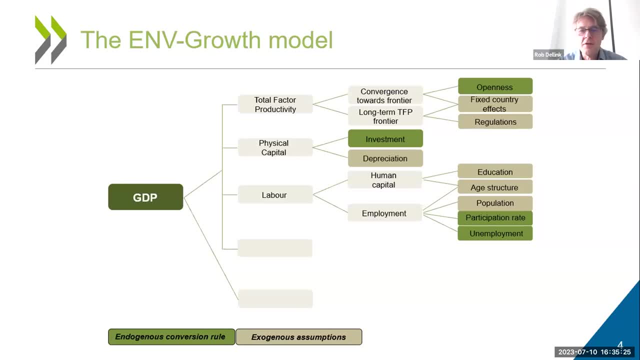 capital directly taken from Samir and his projections, so that includes the education and age structure and also the gender, in building a synthetic human capital indicator for us. And there is employment which depends on also the age structure and the gender and the population. 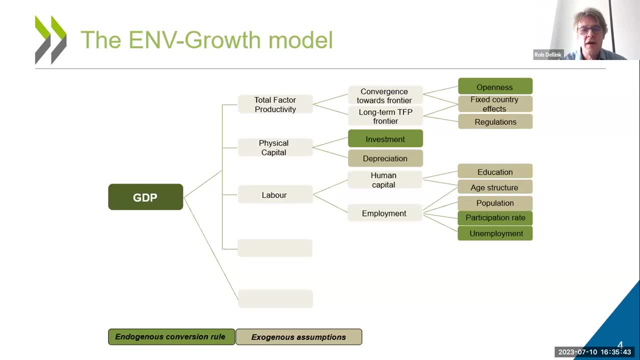 and also on participation rates and unemployment rates, And then together this employment, so the number of people working and human capital, basically how skilled the people are that are working- give us the labor input to GDP. Then there's a smaller thing, which is related to energy, which has energy efficiency. 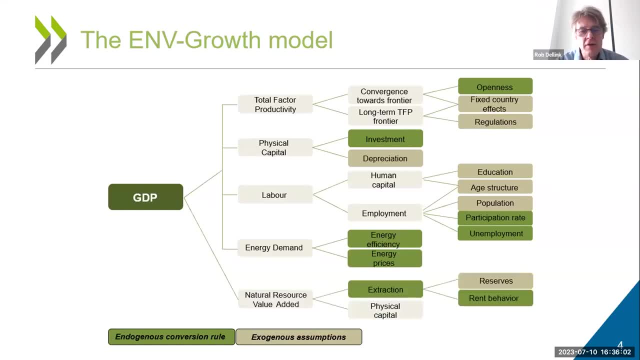 and energy prices. And then, finally, we have something called the natural resource value edits, which depends on the extraction of oil and gas by major economies, And the idea here is that, if you look at the evolution of GDP, for a country like Qatar or Saudi Arabia, it is definitely not. 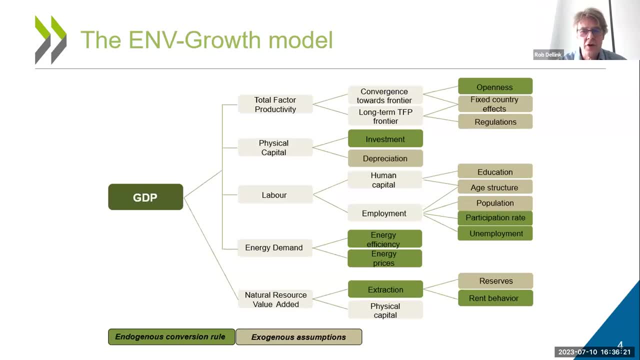 the labor productivity or the total factor productivity that determines the GDP rate. So, for example, if you look at the evolution of GDP for a country like Qatar or Saudi Arabia, it is definitely not the labor productivity or the total factor productivity that determines the GDP rate. 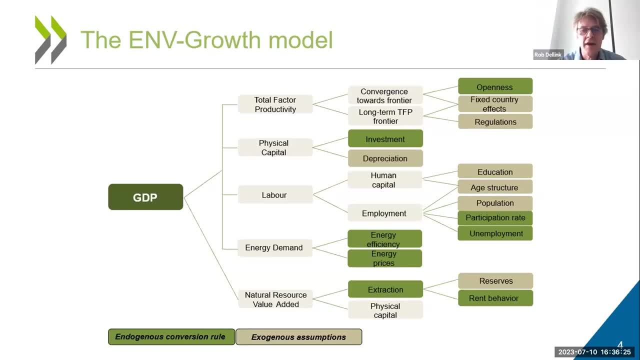 So, for example, if you look at the evolution of GDP for a country like Qatar or Saudi Arabia, it is definitely not the labor productivity or the total factor productivity that determines the GDP growth in these countries, but rather it's the rents that they get from exporting the fossil fuels. 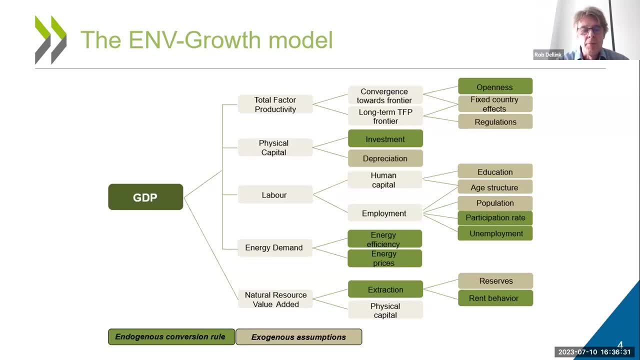 So we split the GDP into the part that is governed by natural resource exports and the part that is governed by basically production in the other sectors. So together that then gives us a GDP projection and a GDP per capita projection. So we incorporated a bunch of different. 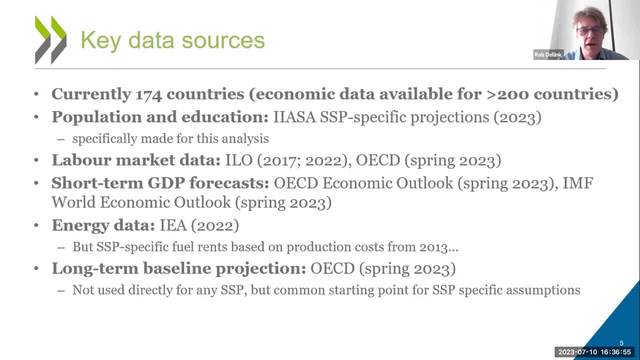 databases. So we have 170 countries, 74 countries which take up all the economic data as well as the population and demographic data that Samir provided. The economic model in itself is more than 200 countries, but there's a number of countries for which we don't have demographic data or for which there's only demographic data and no economic data. 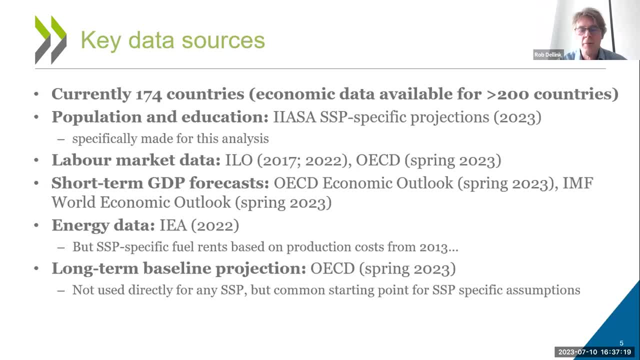 So still the 174 countries, I think, add up to more than 99% of the GDP. So the 174 countries, I think, add up to more than 99% of the GDP. So still the 174 countries, I think, add up to more than 99% of the GDP. 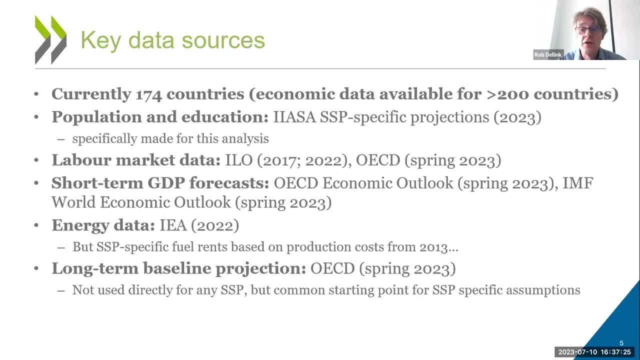 of the world. One major- I think the major country that we do not have in the database is Venezuela because, as people might know, Venezuela, the country's statistics are sorry, the country's statistics are no longer available, So we basically don't have any data. 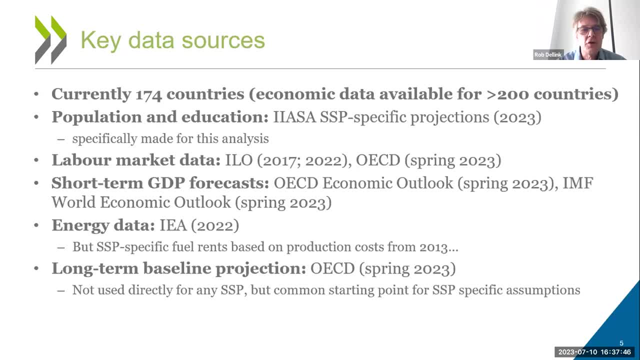 to make projections of economic activity in the future in Venezuela, So that country is out. We use short-term GDP forecasts that run until that are from this spring and that does include a number of the recent geopolitical events, And those are projections until 2025.. So what? the 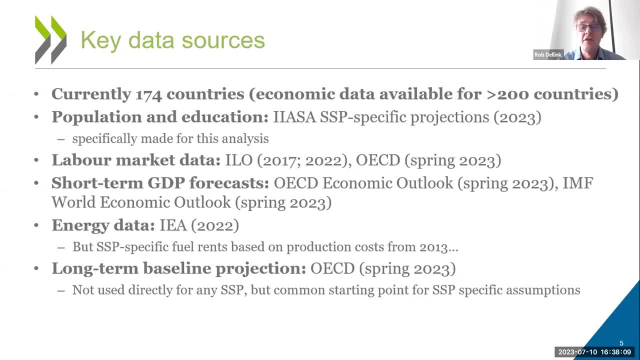 model actually does. it takes those short-term forecasts as if they're data and then makes projections from 2026 onwards using this GDP framework that I had in the previous slide. For the energy data, we use IEA data. but before people get too enthusiastic about looking at this, 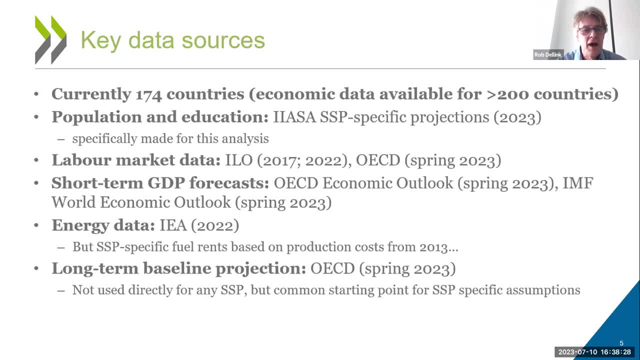 natural resource extraction rents that we have- actually the underlying rent data- is quite old and we don't have any specific new data for that. So unfortunately, this is mostly in terms of making sure that we have a good split between the natural resources part and the rest of GDP. 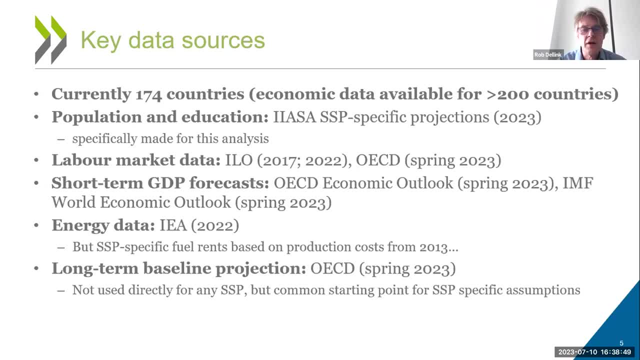 but there's no detailed energy projections And if people want that, I think they have to wait for the integrated assessment models to come up with updated projections of energy and emissions. And finally, the long-term projections that we use are also embedded, basically, on the long-term projections that the OECD is making. 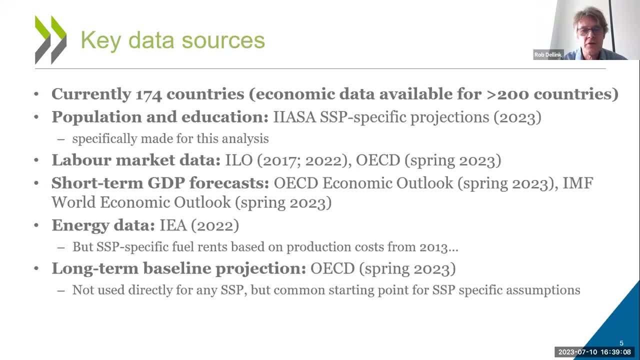 for a subset of countries only: OECD countries and the major G20 countries. These are not directly used in the SSPs, but they give us some starting point for identifying how has. how do economic projectors and economic forecasters, how do they see long-term economic? 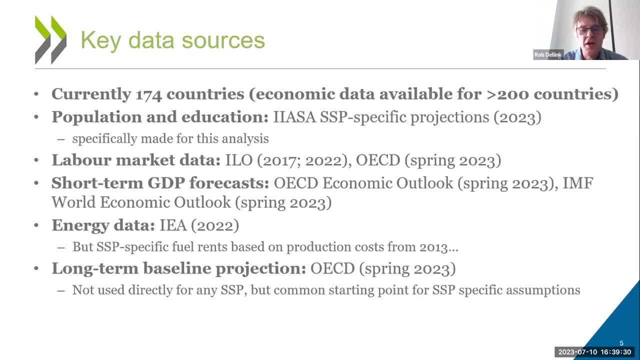 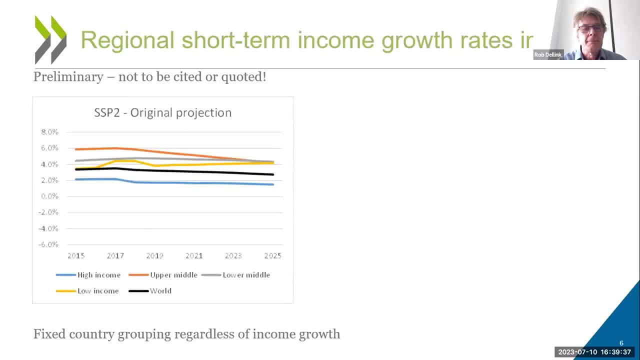 growth in the world And has that changed in the last 10 years? So we do that to basically scale a little bit our SSP projections. So how do we do in between 2015 and 2025 in terms of GDP per capita? 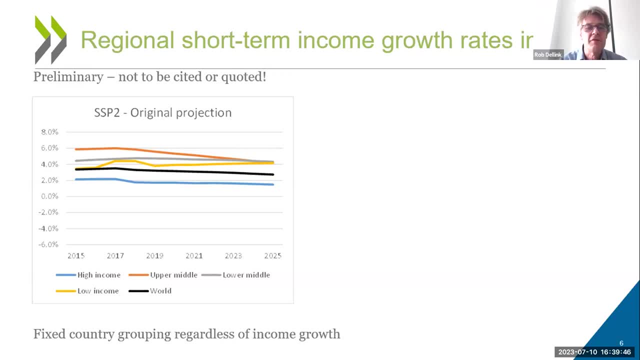 we forecasted something like a 3.5% growth rate in 2015, gradually declining to a little less than 3% by 2025 and at global level, and obviously reality was different. The big one is COVID and you can see that the big decline in 2020. 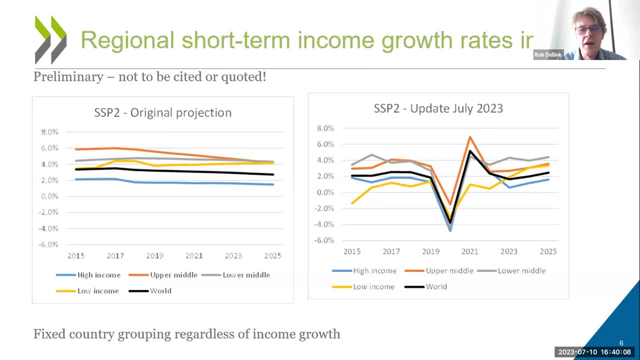 and some recovery in 2021.. But the other thing to look at here is the yellow line, which has the low-income countries, where you can see that already in 2015,, because of this commodity crisis, growth was much lower than what we had expected. Growth is picking. 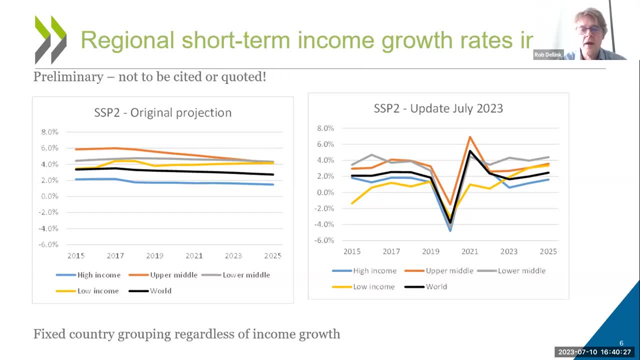 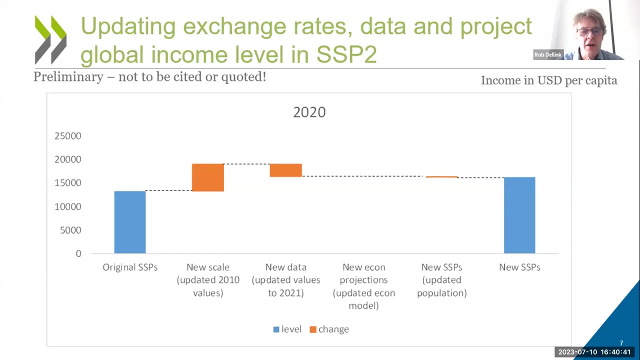 up, and the forecasts are that growth is continuing to pick up in low-income countries, But clearly we have had a decade that was less optimistic than what we had projected. So then, how do we get from the old projections to the new ones? The first one is what I already alluded to: the different definition of GDP and the revision to 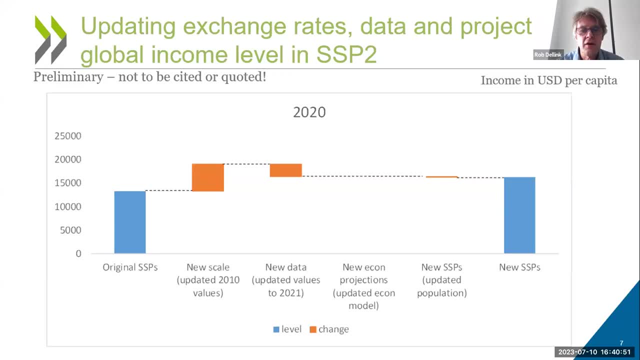 17 PPP exchange rates, which give them larger share in global GDP, to emerging economies mostly, And that gives us a significant increase in the global GDP per capita level. Then the data as I just showed. our economic forecasts were a little bit too optimistic. 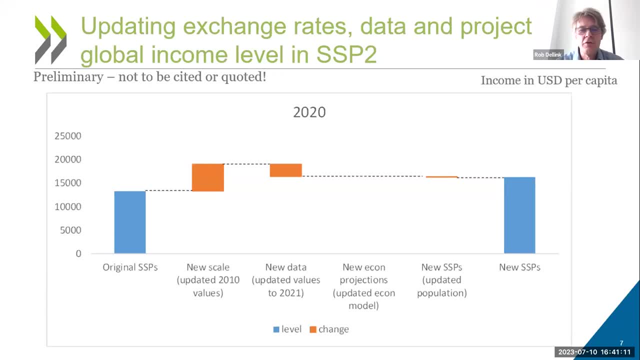 So actually, if you take into account all the latest data up to 2021, we have a little bit lower GDP per capita levels global level. Now, obviously, the new long-term projections don't influence the numbers in 2020, and the population projections are a little bit different, but not that much. 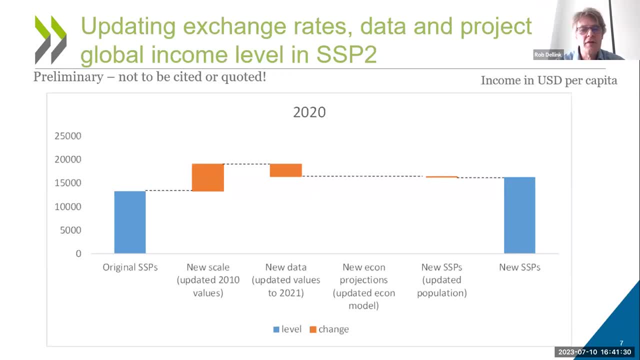 So the new GDP per capita global is quite substantially higher than it was in 2020,. for 2020, is higher than what we had foreseen in the original SSPs, even though 2020 is a relatively low year. But if we look at the longer run to 2100, we still have this scale effect. 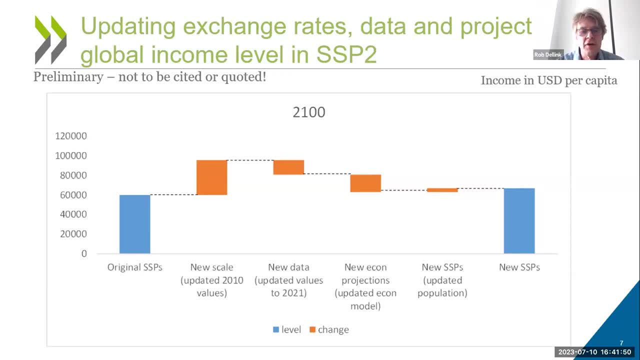 We have the effects of the historical data, we have the effect of the lower data, but now we all have an added effect and that is that we are slightly less optimistic on long-term economic growth And therefore in SSP 2, we have a lower GDP per capita projection at global level. 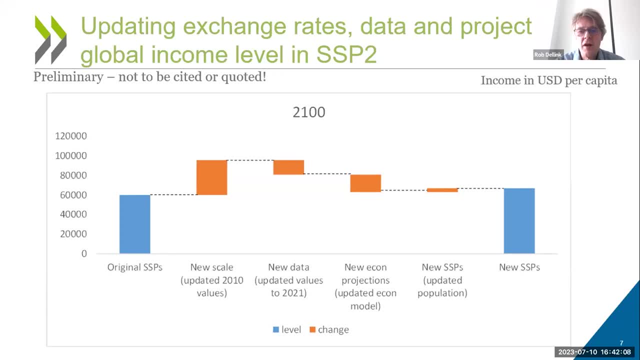 In this case the updated population have a little bit of a positive effect. so that's driven by a balance between GDP. So it's higher. sorry, between total population that's higher, but for us, for the GDP per capita, it's mostly working age population that determines the GDP per capita, as that leads to labor input into GDP. 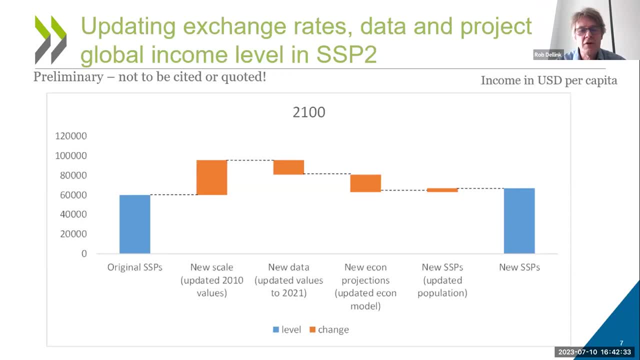 And the latest forecast, the latest projection that we have is for 2100- that that leads to a slightly higher GDP per capita. So in total, GDP per capita for SSP 2 is somewhat higher than in the original SSPs, but not actually as much as you would think from January. 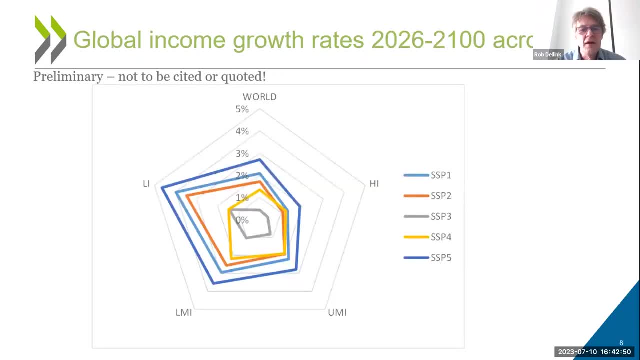 the rescaling of the data. So if we then look across the different income groups- high income, middle income, lower middle income, low income countries- and we compare across the SSPs, we see a very similar story to what we had 10 years ago, which is that SSP5 is the high growth. 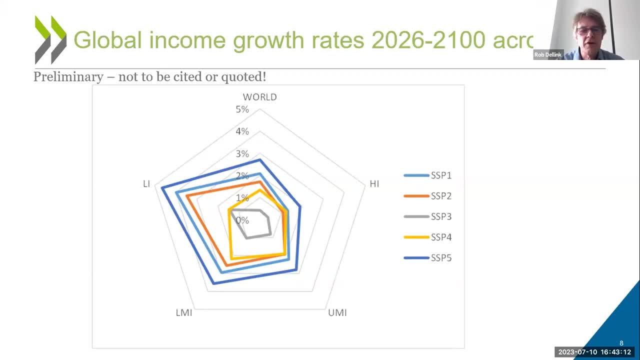 scenario. SSP2 is a kind of middle of the road scenario. SSP1 is also higher growth than what we have in SSP2, and SSP3 is the low growth scenario with very low growth rates, except potentially for low income countries which have some growth still. that is well above 1% for most of the century. 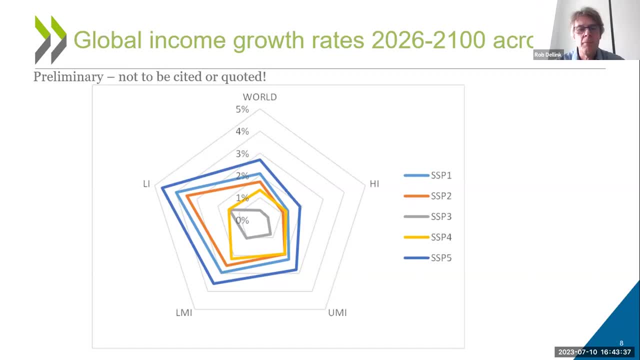 And then SSP4 is this combined scenario where basically the low income countries are more in SSP3 type of worlds whereas the high income countries are more in an SSP1 type of worlds, And so you get this shifted focus where growth is lower in low income countries and actually much more. 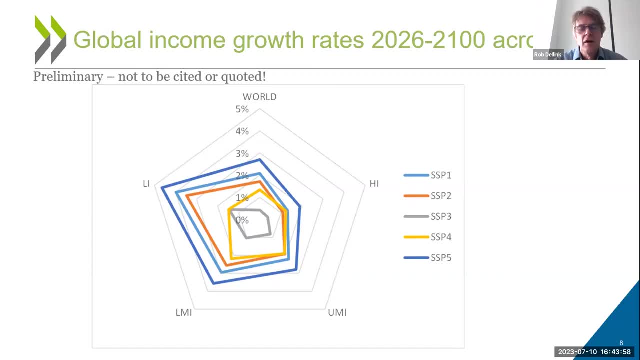 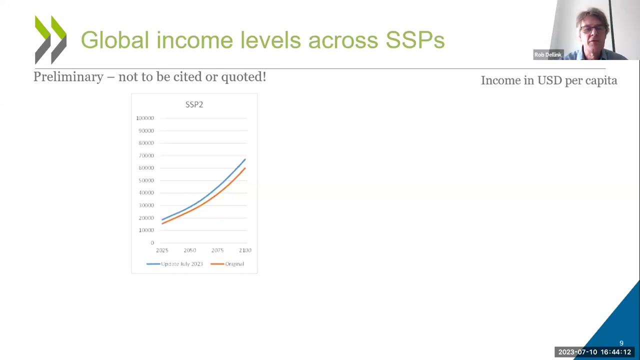 So you see upper middle income countries and lower middle income countries still catching up and converging in income levels, but actually high income countries and low income countries have much more moderate growth there. So how does this translate into GDP per capita levels? So we start. 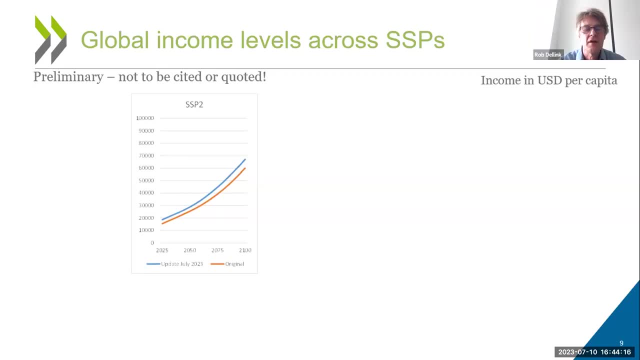 off at a higher base in 2025 because of the increase in GDP per capita, and then we start off at a higher base in 2025 because of the increase in GDP per capita. So you see higher base in 2025 because of the increase in GDP per capita and then we start. 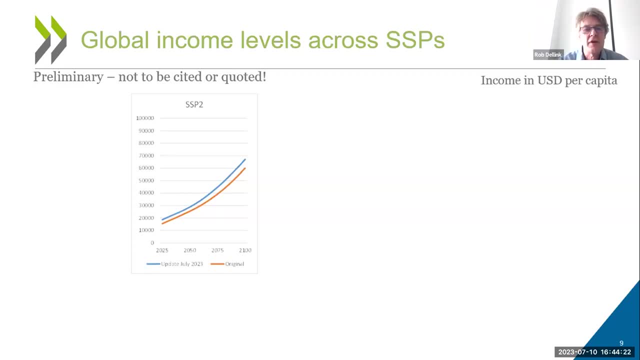 off at a higher base in 2050 because of the increase in GDP per capita. and then we start CB, as the 2.2 billion BR basis rate that was quite high last year in永 nella de Christ has gone up doubtless because of that. 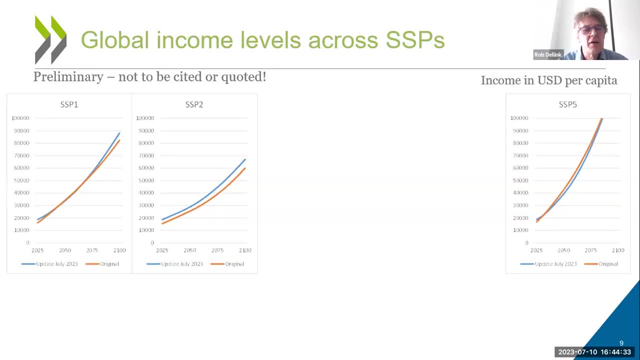 While with classe number 1, we have an out-of-ποld decision status. And then 35 billion model for accessory reality is at the back up to 6 billion, and they all kind of go here and they all grab. 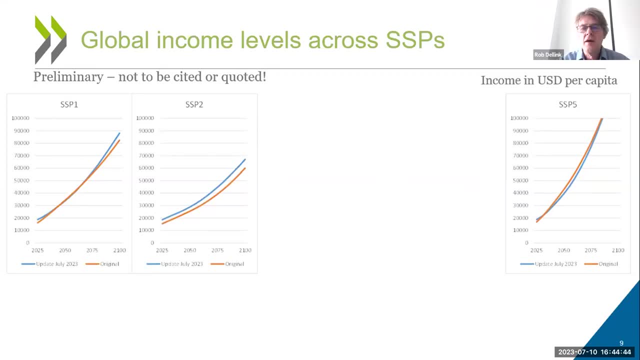 theirźniej. So this data is based on this and its valid構 자기 bottomness. perceiving the. we have somewhat higher growth, We start higher, but we have slightly more pessimistic growth rates and therefore this doesn't get sustainable. 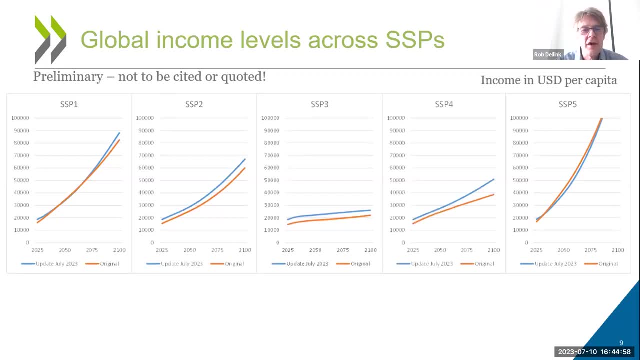 But in SSP3 and SSP4, and especially SSP3, this difference in the base year. if you have low growth rates, then the rescaling of course matters a lot for the level of GDP. So in SSP3 especially, we just basically the whole growth. 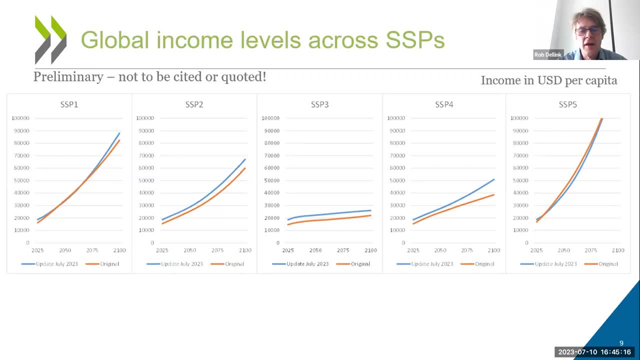 the whole line is scaled upwards. and then in SSP4, we see, because we have now a differentiation between upper middle income countries and lower middle income countries, we have differentiated growth rates for those in SSP4. that leads to somewhat higher growth at the end of the century. 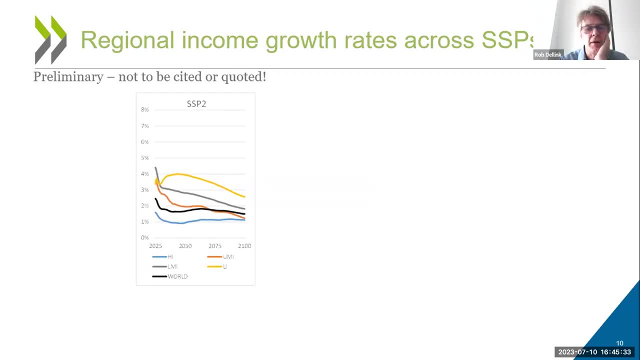 But perhaps more interesting is to look at this in terms of regional growth rates of GDP per capita. So SSP2, you see a small growth boost in lower income countries. This is actually a little bit lower We had in SSP2 10 years ago. 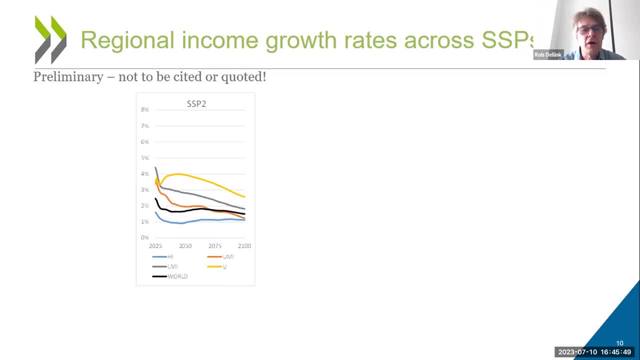 we expected a stronger boost in growth to up to 5% or so. We are now a little bit more pessimistic and think growth in low income countries will remain below something like 4% roughly, And then over time the growth rates across the different regions. 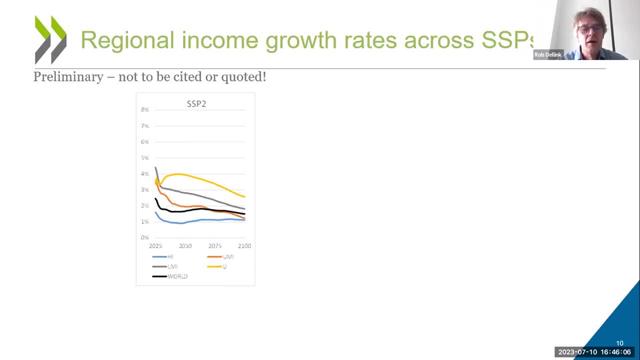 converge over time, but not exactly. But they converge basically because in high income countries they are closer to their frontier, So their only way of growth is coming from lower income countries, From the frontier movement itself, whereas in high income countries and lower middle income countries 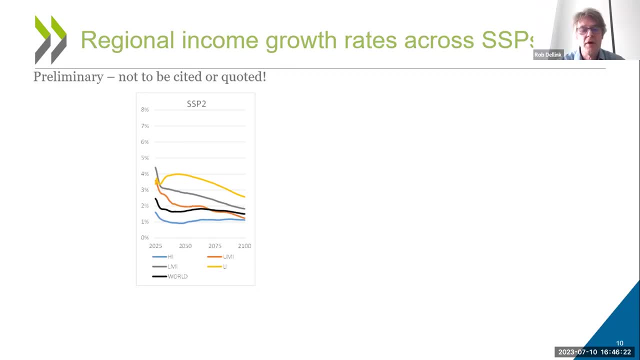 you have high growth rates in the beginning because they're catching up to the frontier more rapidly, And then over time that effect fades away and they have still region-specific growth rates. So there's no full convergence across countries, but they are closer to their frontier. 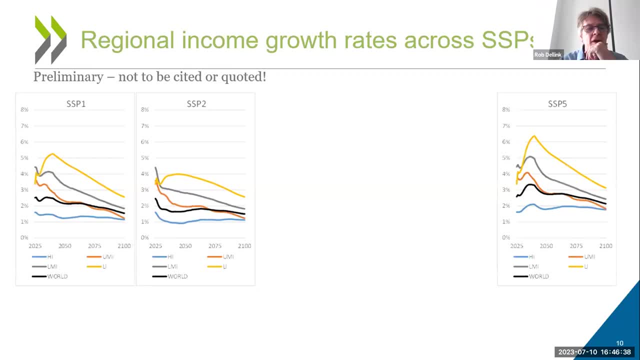 and therefore their growth rates decline. Similarly, SSP1 has a higher growth spurt in the beginning first half of the century, and SSP5 as well, Whereas in SSP3 and SSP4, these growth rates are declining much more rapidly, And you see, especially in SSP4,. 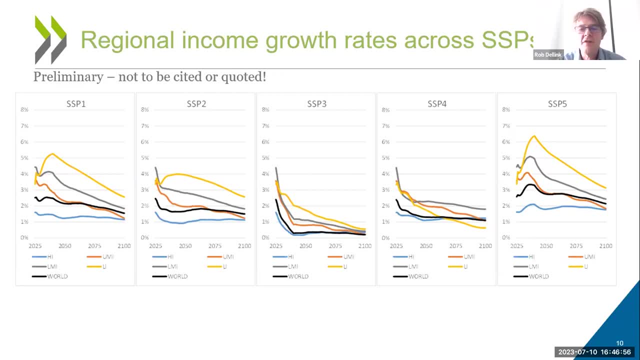 that the lower income countries actually have a very low growth rate- that's even below the high income growth rate, because they are basically to some extent excluded from the global economy- is in the storyline of that scenario. We also see that in SSP3,. 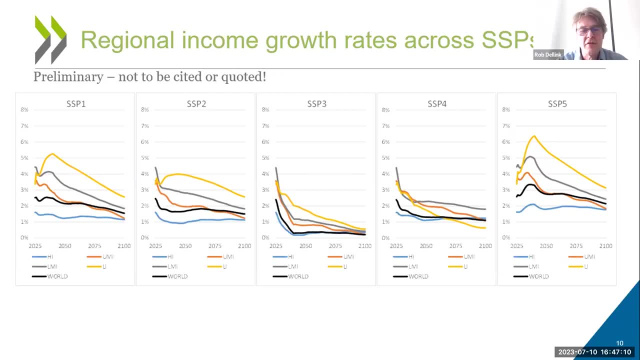 the global growth rate declines very rapidly to only something like 0.3 or 0.4%, And that is a very low growth rate that's then sustained throughout the century. So this is not a post-growth or a non-growth scenario. 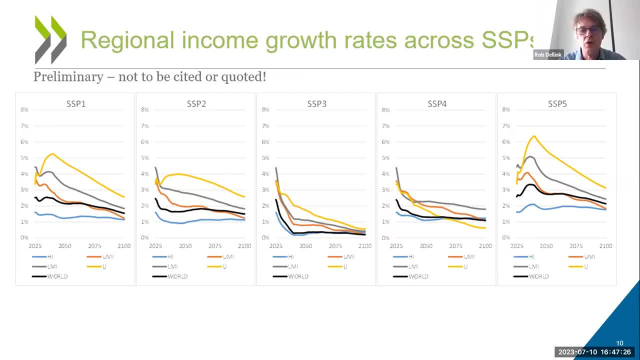 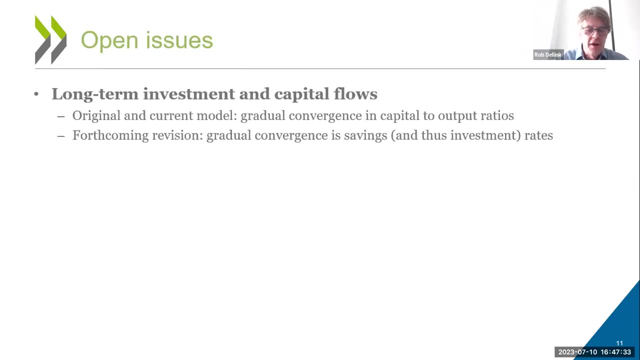 but it gets very close in terms of having very low technological progress in this scenario. Now, these are preliminary results. They do use the latest projections of Samir, but we have a number of issues that we would like to still look at. One important one is long-term. 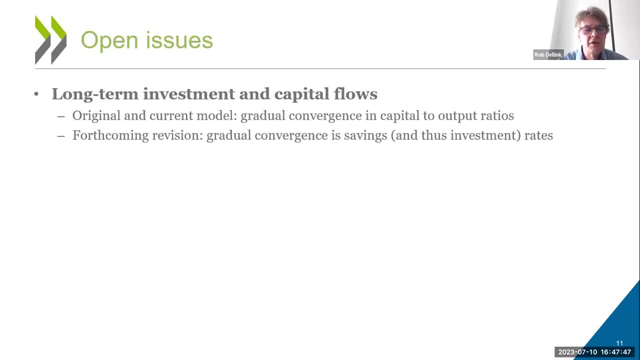 long-term investment in capital flows. What we're doing here- the results I presented today- is that we have gradual convergence in capital to output ratios across countries, And the idea being that, as countries grow over time, some countries have a very low capital input. 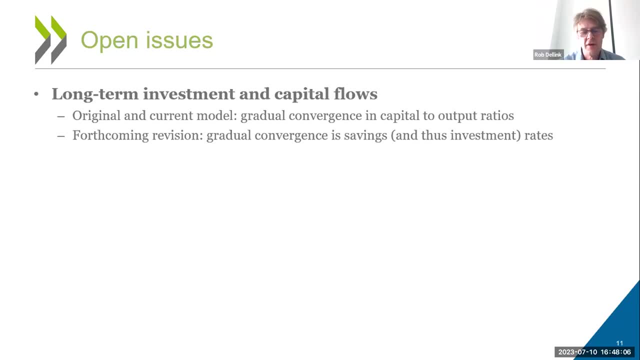 in their economies and these would grow more fast and would invest more and capital would flow there from other countries to increase their capital to output ratio. There's been an ongoing discussion and also our internal economics departments. There's no real empirical backing up for this assumption. 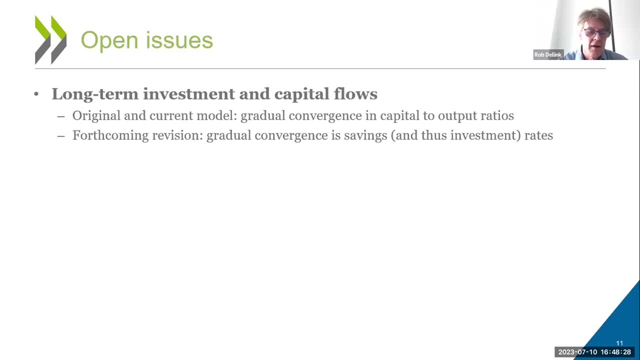 And it also the other downside to this assumption is that it does not allow for a different specialization of economy. So imagine an economy specializing really in industry versus another economy specializing in services. They would not have in the long run, they would not have the same capital to output ratio. 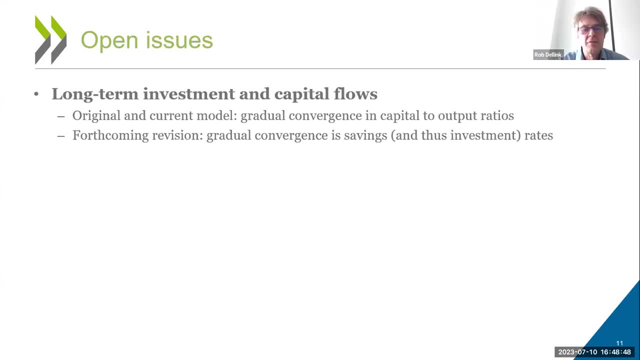 So this gradual convergence assumption is probably not the best to take. So what we want to work on in the coming months is to change this gradual convergence towards savings and thus investments. The other thing we're struggling with is labor force participation rates. We used to have fairly up-to-date projections. 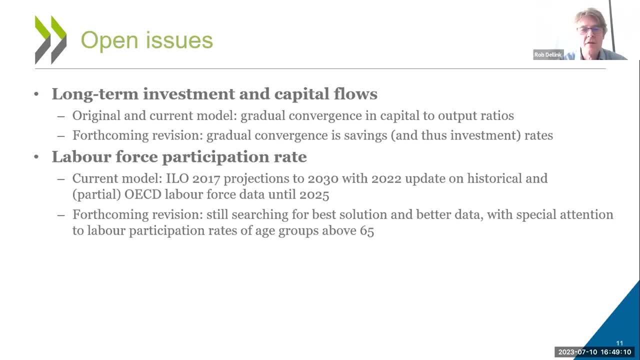 from the international labor organizations. They have not made any recent updates, except for a very early one, which is the labor force participation rates. We used to have fairly up-to-date projections from the international labor organizations. They have not made any recent updates, except for a very early one. 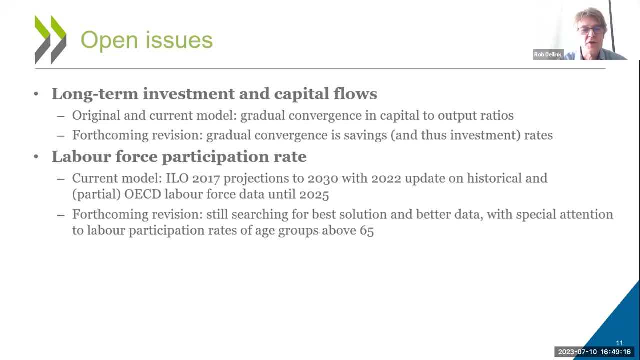 which is the labor force participation rates. We used to have fairly up-to-date projections from the international labor organization. We used to have fairly up-to-date projections from the international labor organization, very aggregated one in 2022, but that doesn't have long-term projections. 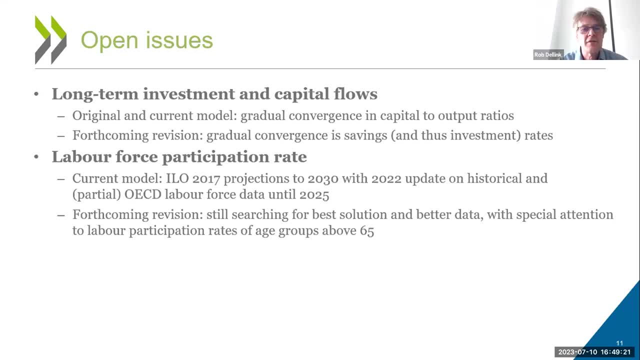 So we're really struggling with what to assume for the latest labor force participation rates in the long run, and especially as we see that population ages increase, so for labor force participation rates of age groups above 75 become more important to get right. so we're still looking into what are the best data. 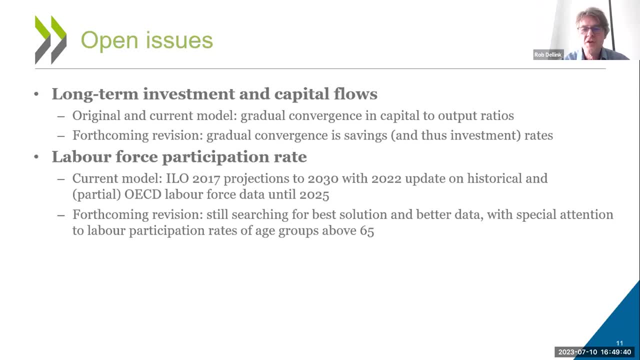 and the best solutions there, And I'm very happy to chat to people if they have ideas for this. and the first thing we want to do is do some careful internal review, of course, and also incorporate the feedbacks from the modeling groups, and we hope that you all spot the errors that we 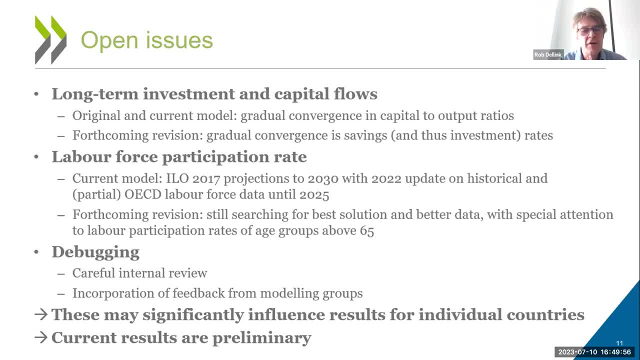 make or implausible some implausible assumptions or implausible results from our assumptions. um, i think the global storylines will not change, because that's the idea. we use the same storylines, so the global gdp per capita might still be roughly the same, but especially, i think, the 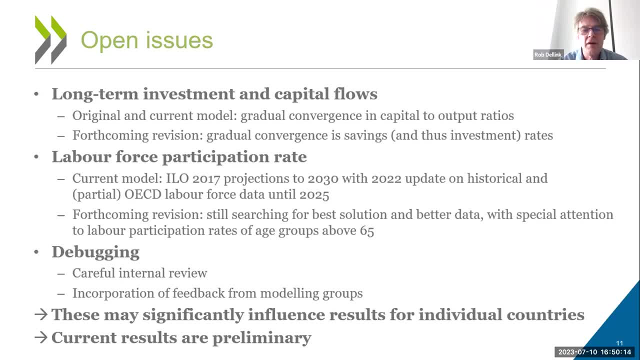 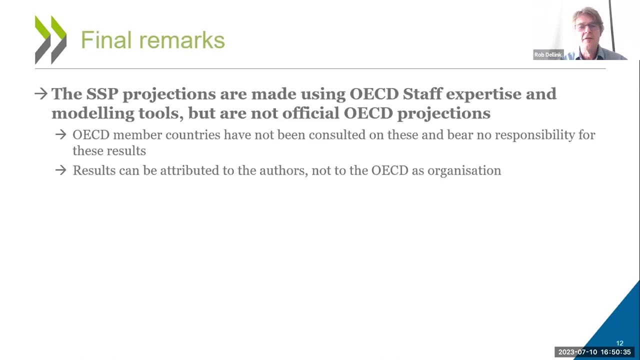 upper middle income countries, for example. these results might be significantly influenced by these assumptions we have on capital flows and labor force participation rates. so country results will be different. we cannot predict how much different they will be, but that's to say that the current results are really preliminary. so they are my personal and and my colleagues. 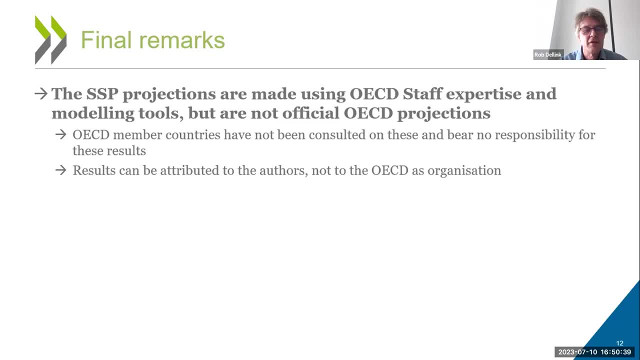 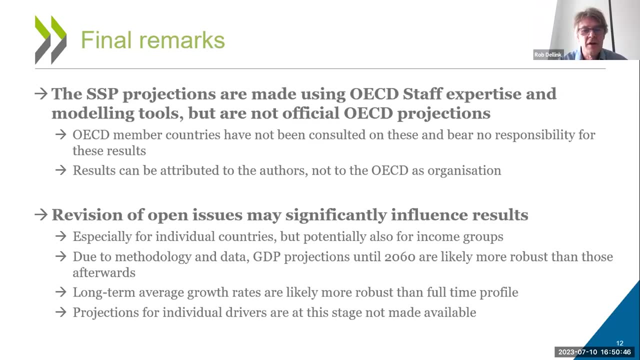 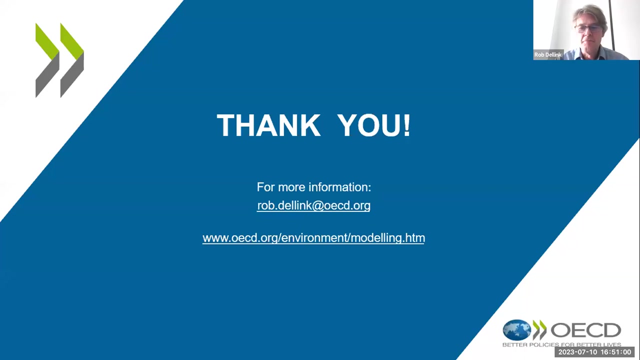 our projections, not official osd projections. i cannot emphasize this enough. you and we do have this revision that might influence results. um, so be careful when you do the updates to these preliminary results. they're more for testing than to update your model and then think you don't have to do anything anymore for 10 years again with that. i thank you, thank you. 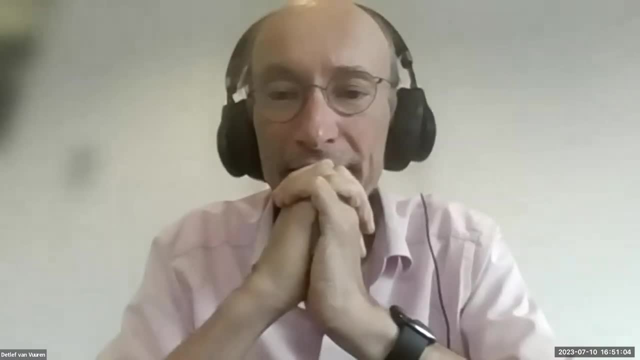 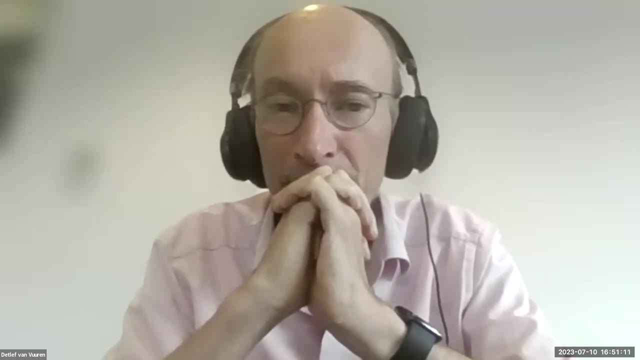 yeah, so indeed, the the numbers are released not only for testing, but above all, also for comments and um. so, based on comments from the gdp per capita and the gdp per capita and the gdp per capita, we can expect that some of these numbers will change. so be really, really careful. they're not 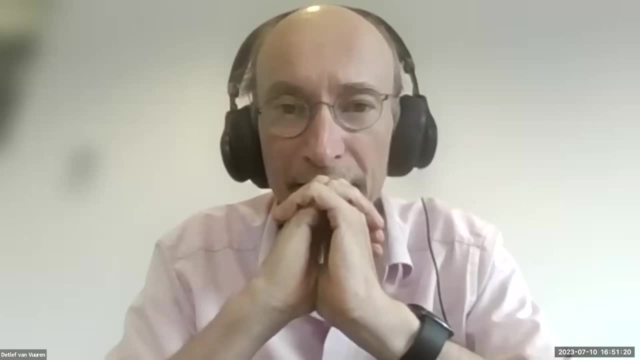 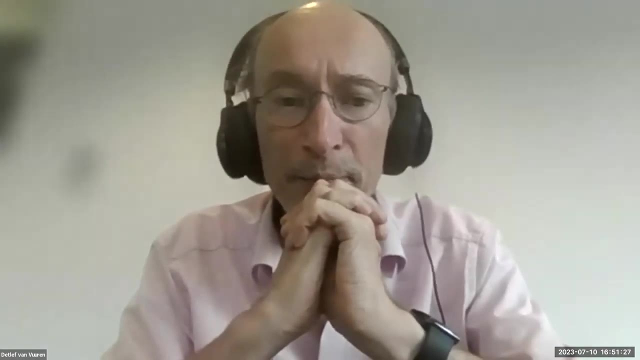 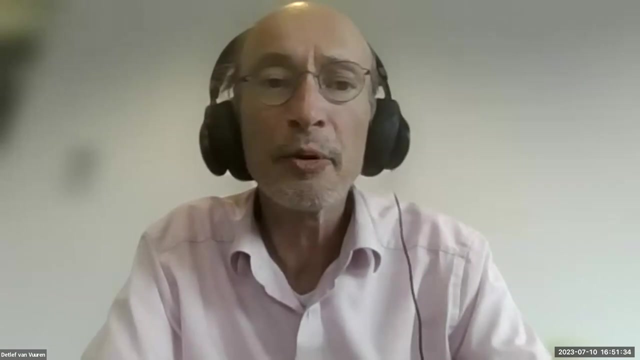 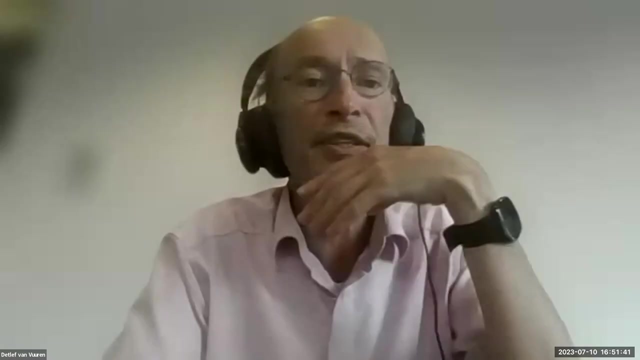 meant to be used already and referred to. they are really simply preliminary results. um, yeah, thanks, so, uh, we. there are some questions in the q a. maybe we can pick up two first and then go to more to the more general questions. um, so, one the word, several questions related to the, the unit of dollars that you're using, and 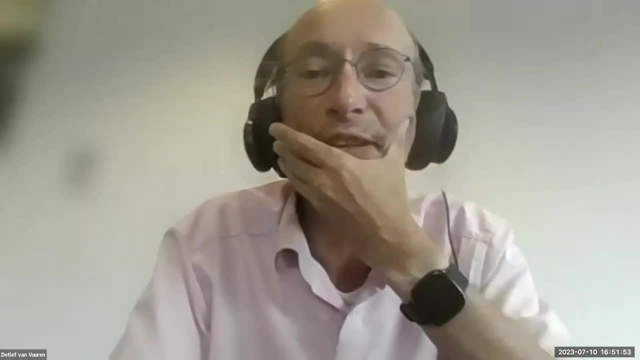 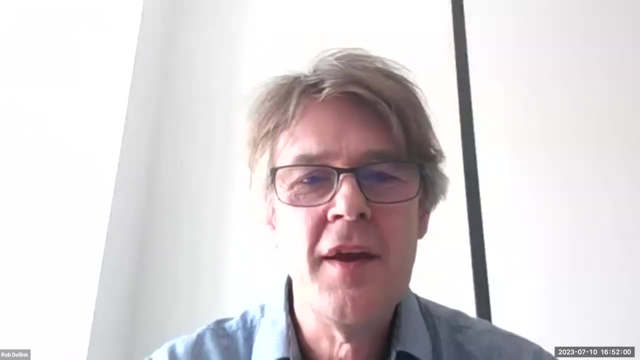 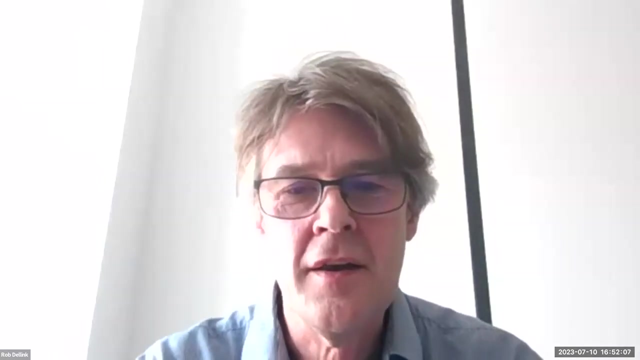 that people have might have used 2005 dollars instead of 2017 dollars and things like that. any recommendation? recommendation there? um well, i would urge people to update to more recent uh exchange rates, for the simple reason that, if you just look at the share of china in in global, 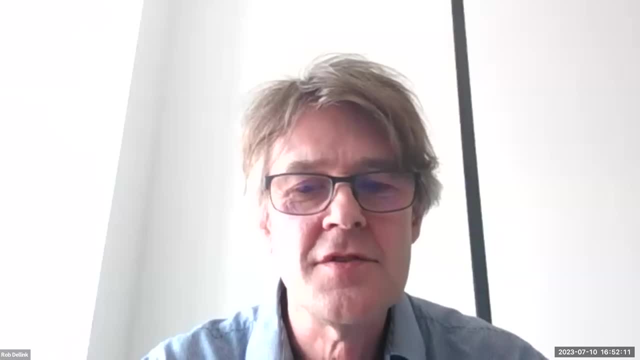 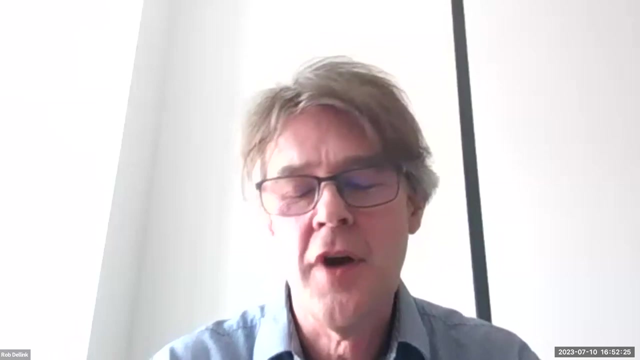 in the global economy that has changed so much in the last 10 years that if you use these very old ppp exchange rates, you're really making- um, you're making- a wrong assumption of the growth of the global economy, basically. so if you do this for at a country level, you do individual country analysis. 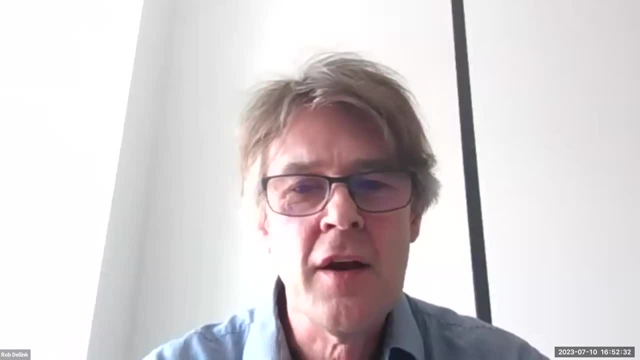 and you use individual country energy data to then come up with energy individual country emissions projections, there's not a big problem. you can use whatever exchange rate you need because basically you're doing the thing at the individual country level. but the moment you start aggregating across regions into regional grouping, these things really matter and they really matter. 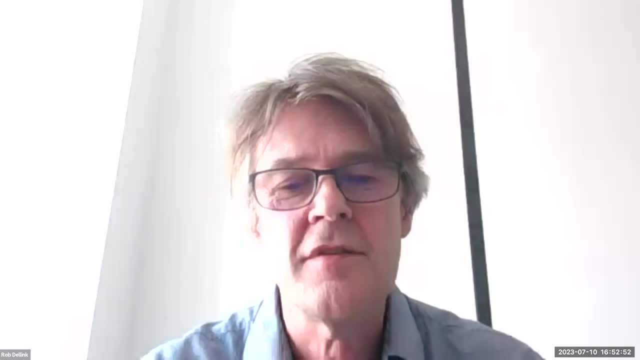 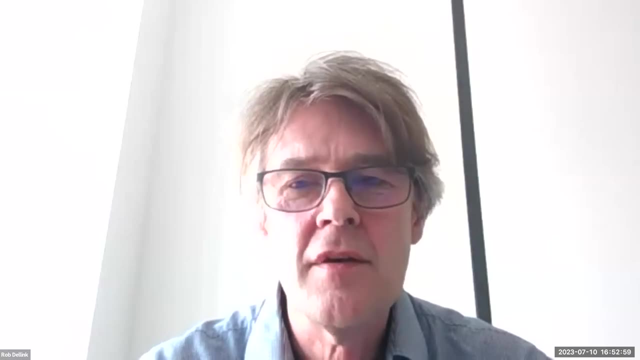 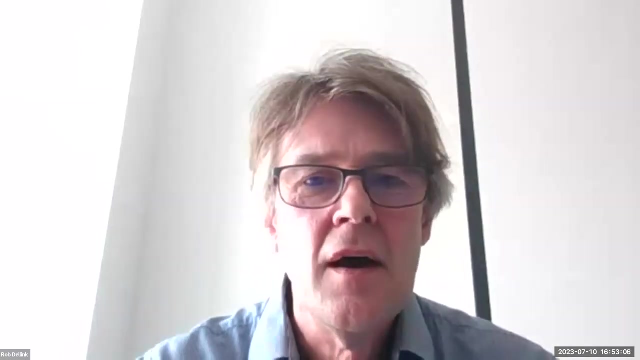 also for for the, the qualitative insights from your modeling. um. what we can do at some stage- not in a very short run, but a bit later- is to come up and provide a database with ppp convergence rates. um we also want to release in the final revision. we couldn't do it for this revision, but in the final revision we also want to do. 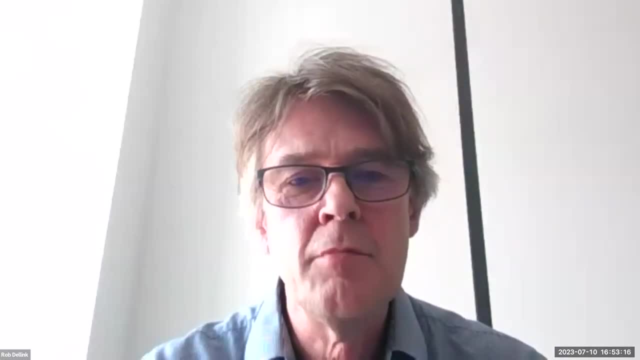 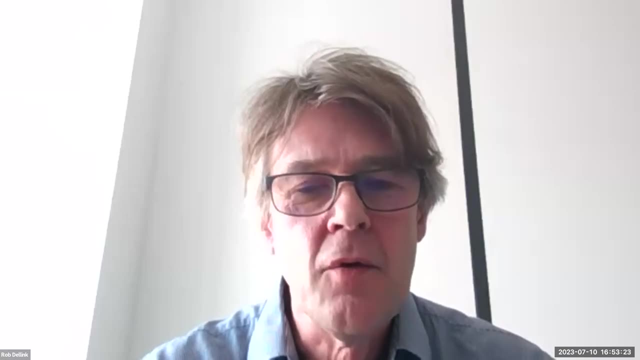 market exchange rates, gdp in market exchange rates rather than in ppp exchange rates, and we can have a convergence table for that as well. um, for people that really want to do this, this type of convergence, in the short run, i would advise you to go to the icp. they have ppp exchange. rates for individual countries across the different years. the only thing to really keep in mind that this convergence also takes into account inflation rates in the country that is the that is the basis for your exchange rates. um, so you would need not only to change your ppp exchange rates, but also change 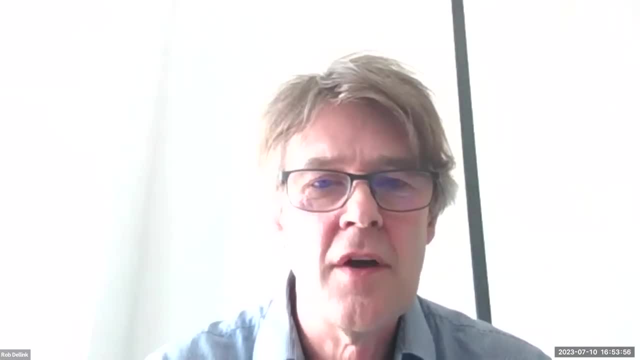 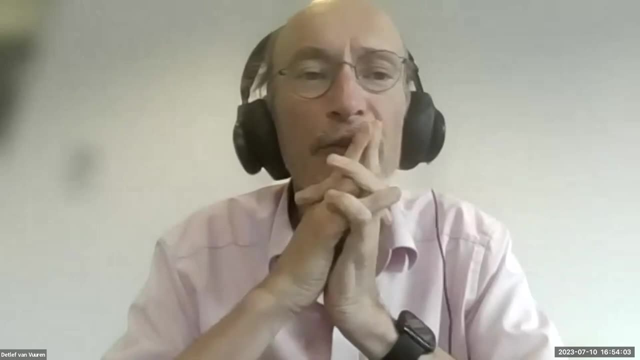 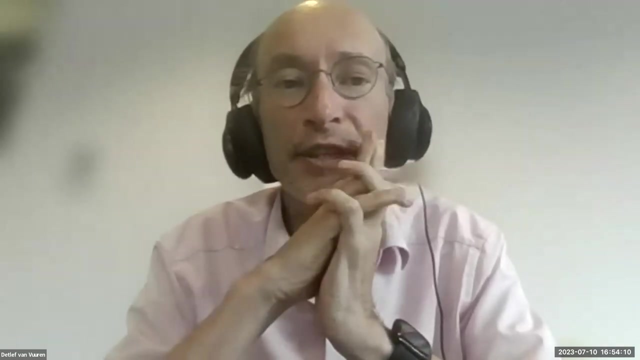 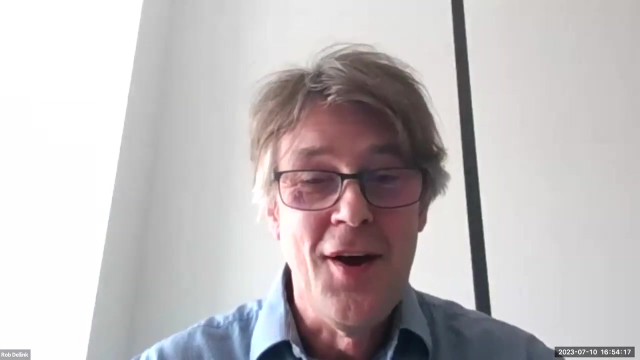 the, the price level in your target country, say the us. so a second question: you are using all kinds of some assumptions and, um, you're using all kinds of assumptions, um, but are you really willing to share any of your data on that, on the underlying drivers, like labor? are you willing to share those? 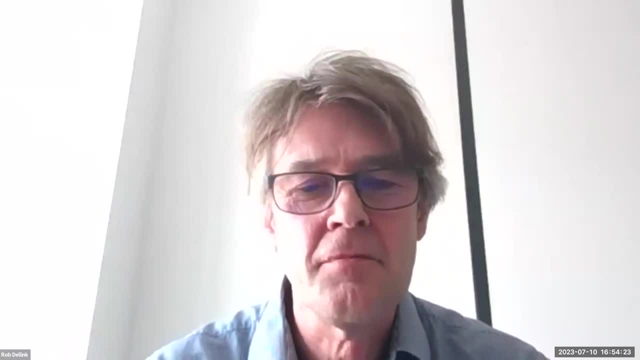 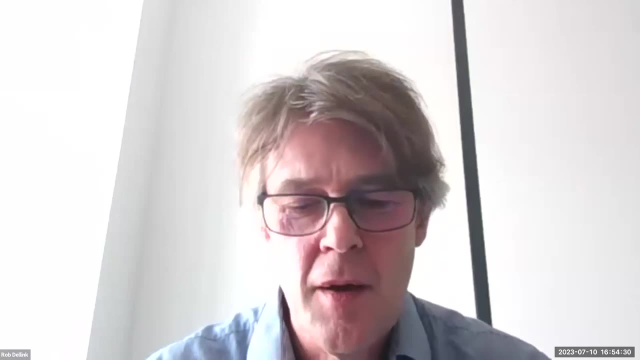 that's a good question and we have received that a lot in the last 10 years and i'm always hesitant. so first of all, we'll not do this um for this preliminary round because especially also the drivers will change when we make changes to labor force participation, participation rates. 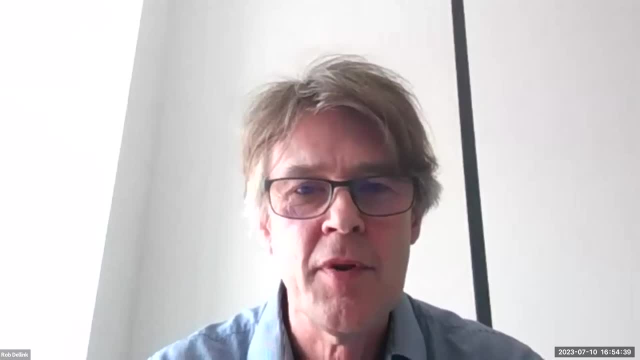 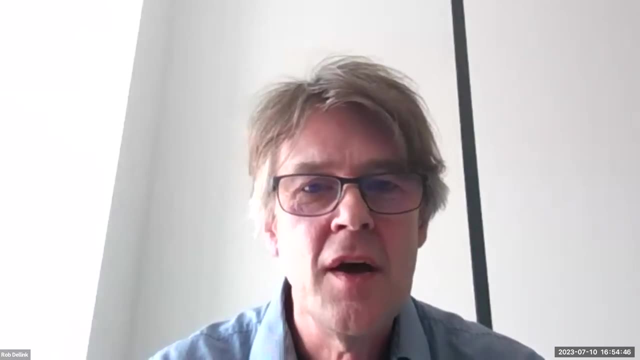 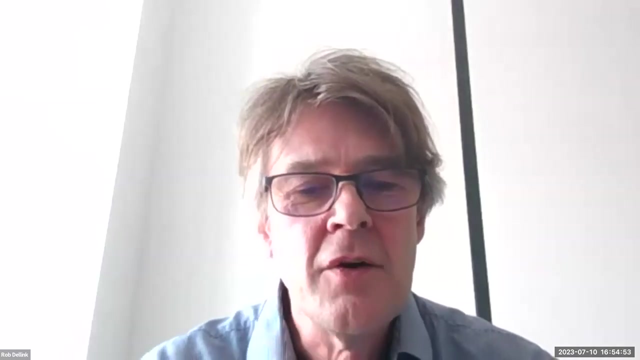 etc. rates that come from a model with human capital as a specific, separate driver of GDP and you plug that into a model that doesn't have human capital, you have a really serious misunderstanding of the total change in labor productivity, So the shares of the different inputs in your GDP. 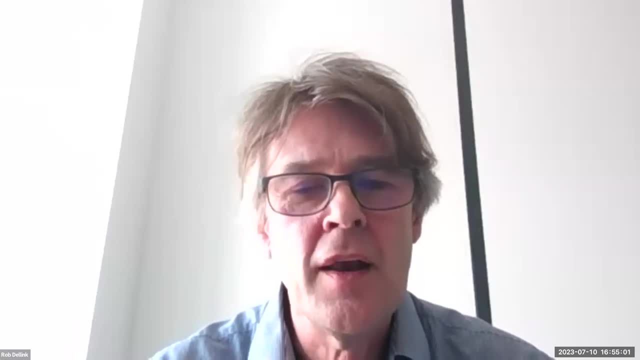 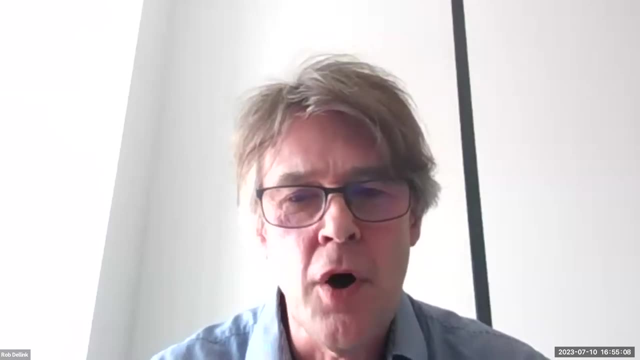 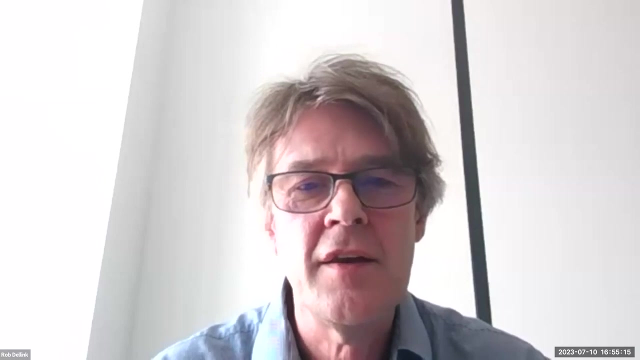 depend crucially on how you specify your model, and it becomes very tricky to use the growth rates for individual drivers if you use a different model than ours. So if you're using exactly the same model as ours, I think you can use our drivers as well, but the moment you deviate. 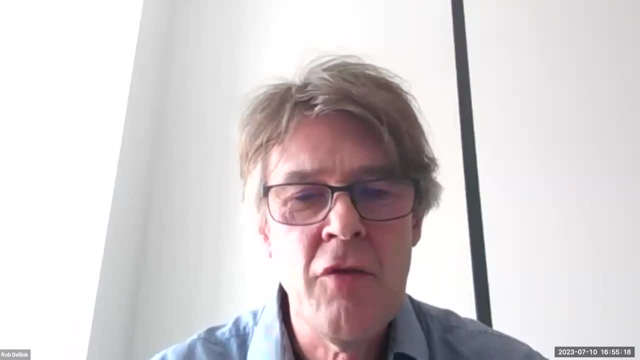 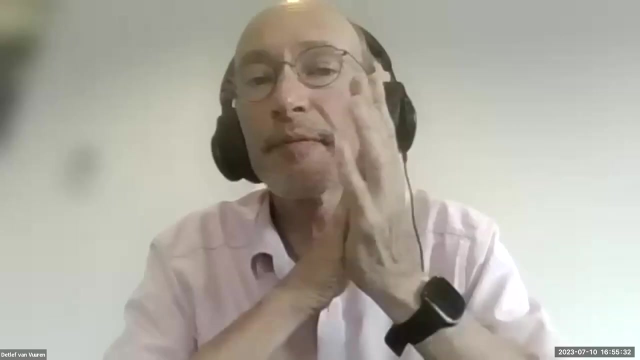 in your drivers, it becomes very tricky. We have worked with individual groups in the past to look at comparison between their model and our model, but it becomes really a tailored approach for individual models that we don't really share with everybody. Yeah, great thanks I. 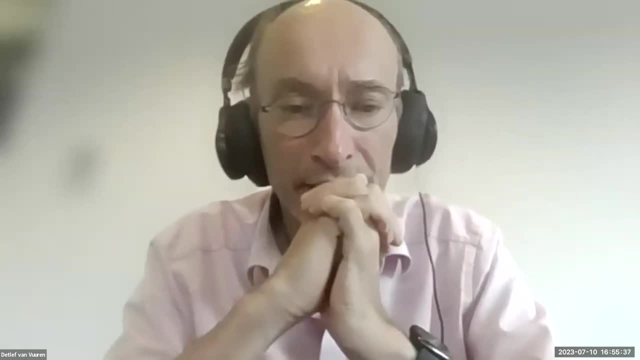 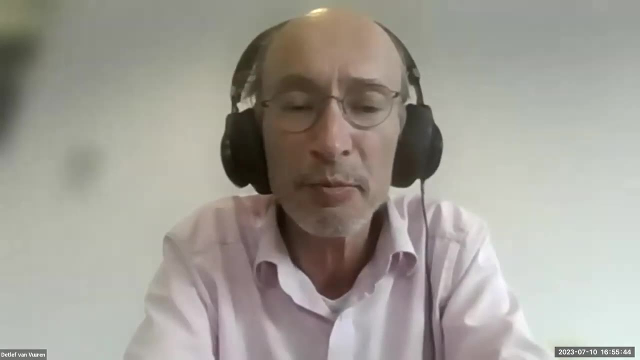 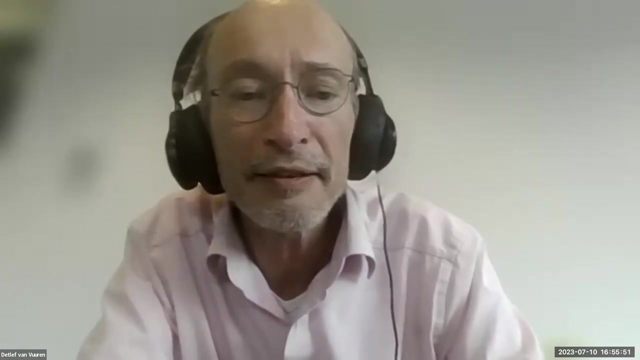 would like also the floor to be open for more general questions. so feel free to type those also into the Q&A, not only those specifically on the economic projections. But in the meanwhile people might think of the more general questions they would like to ask. Let's continue with one. 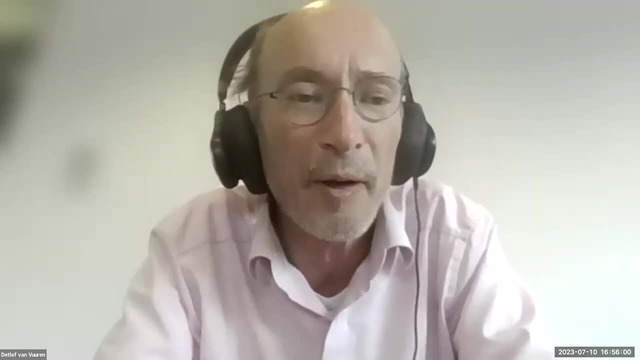 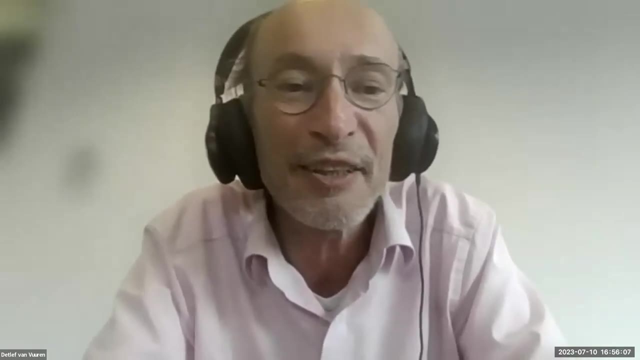 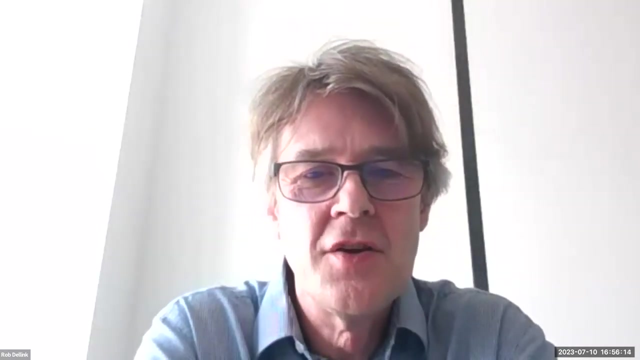 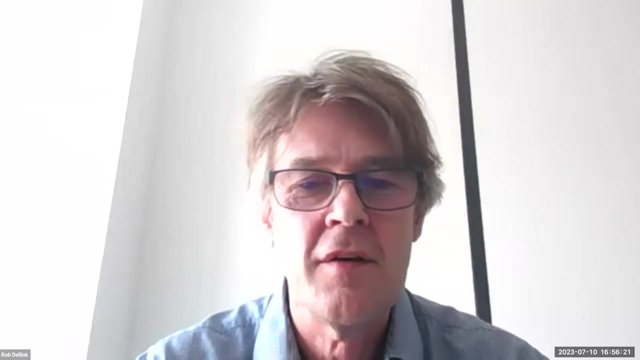 more GDP-related question. Now picking up the one of Chris Smith: is any of the factors GDP climate dependent and are you taking that into account? So they are not. We have not included any feedbacks from climate change on any of the drivers. We do have data and projections. We have made several studies ourselves and we, of course, 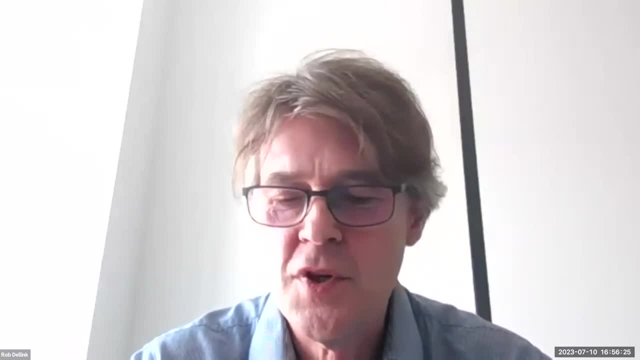 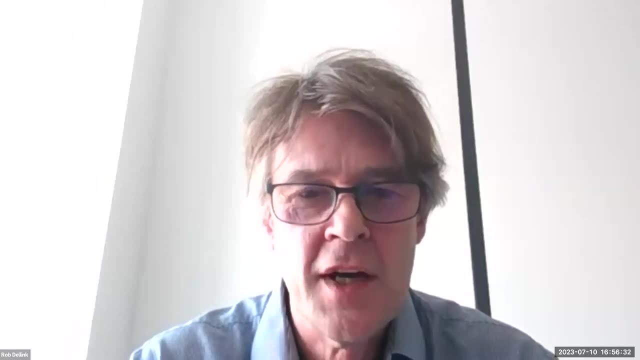 all the integrated assessment models have been using these to project damages from climate change And we deliberately do not put these in, because one of the objectives of these SSP GDP climate dependent factors is to make sure that we have a good data base for GDP climate dependent factors And we have made several studies ourselves and we of course all the integrated 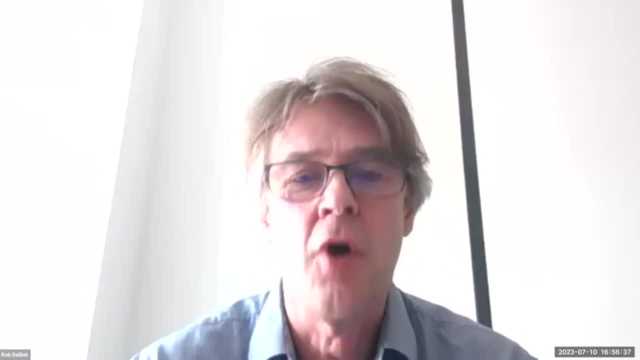 assessment models have been using these to project damages from climate change And we, of course, all the integrated assessment models- have been using these to project damages from climate change projections. is that people can use this to make their own projections of the impacts of climate? 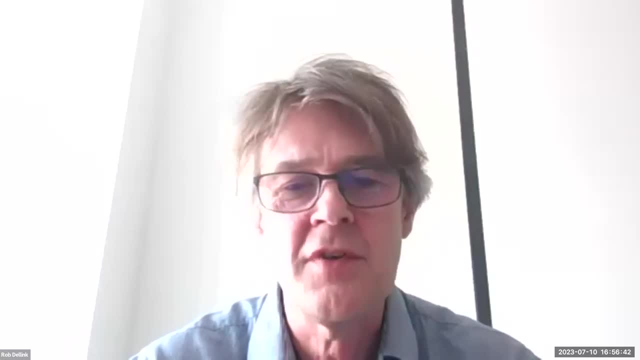 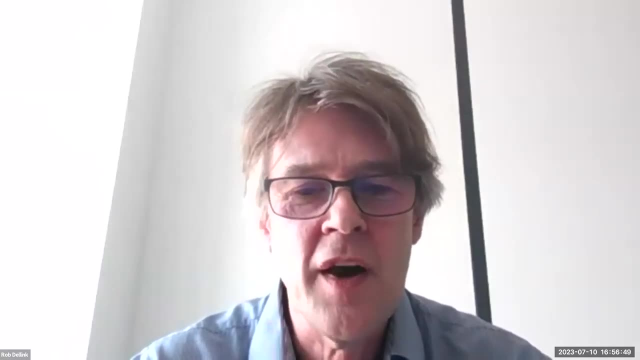 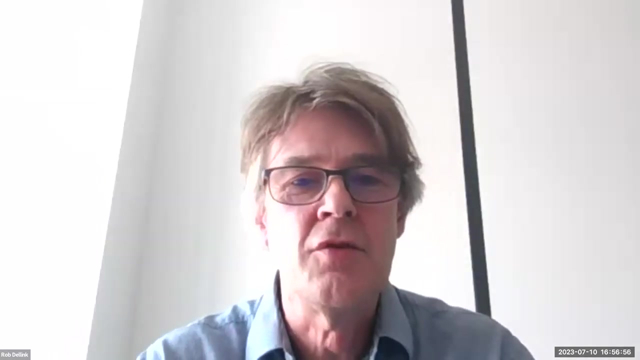 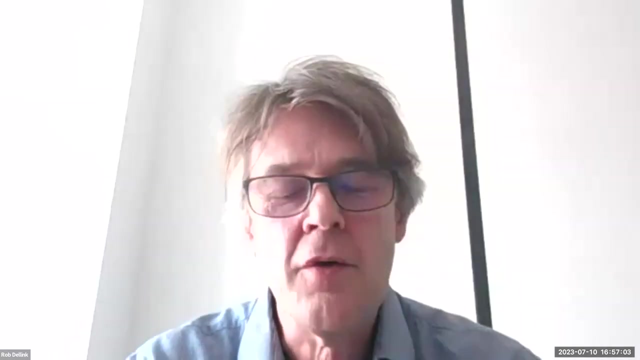 change. So if I would already have, say, a 2% labor productivity loss from climate change in these projections of GDP and then somebody wants to study what happens to labor in a specific country using these SSP projections, they would first then have to know what I assumed in that. 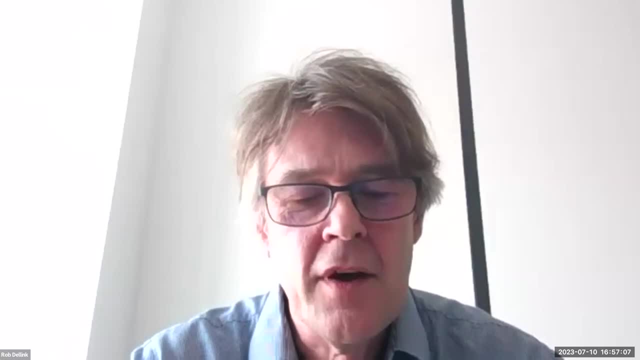 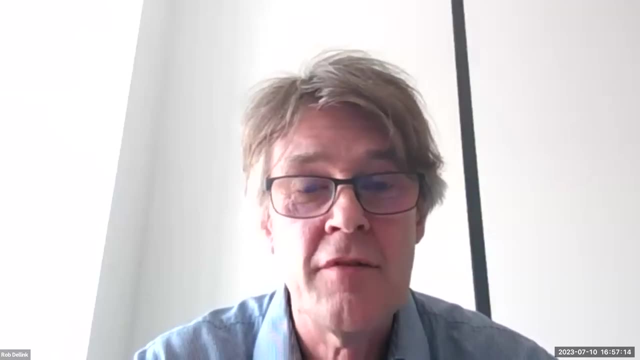 situation, And then they would have to do their analysis. The second reason to not do it is that there is a big discussion in the economics terrain on the scale of damages from climate change by the end of the century, with some people saying it's in the order of magnitude of a few percent of GDP. 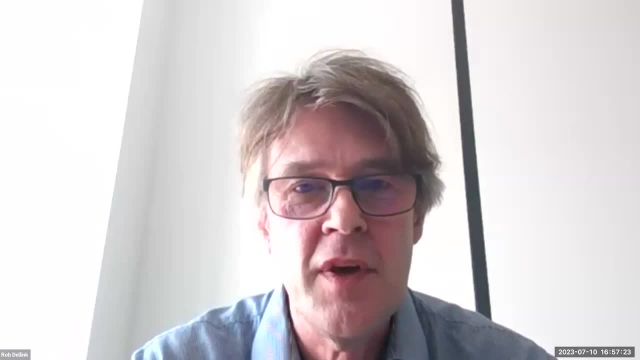 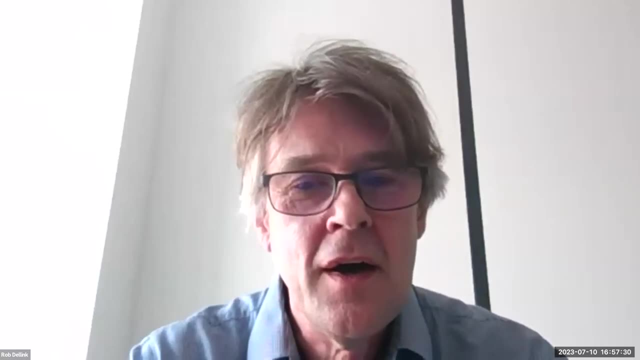 and others saying it could be well above 25% of GDP in terms of the macro damages from GDP. I have a view on that, a personal view, but that's not an interesting one. You might have a personal view on that, but that's not an interesting one. You might have a personal view on the. 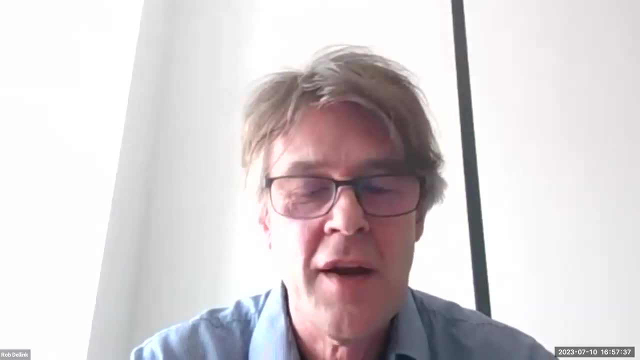 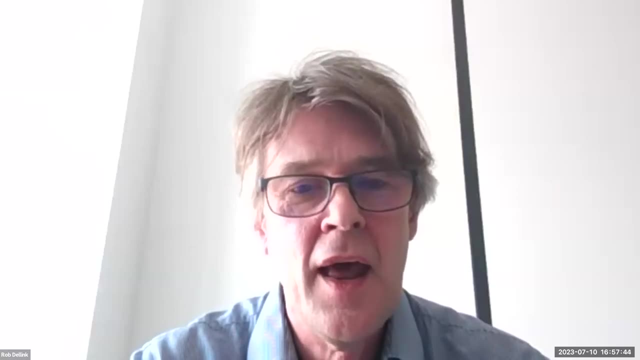 on that. So if you want that, you can always correct these GDP projections with your own view on what the macroeconomic damages from climate change should be and then add that, but just don't attribute that to the GDP projections that we deliver. Yeah, so this is really a catch-22. 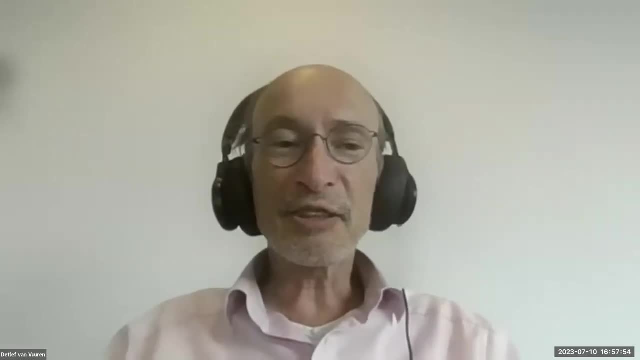 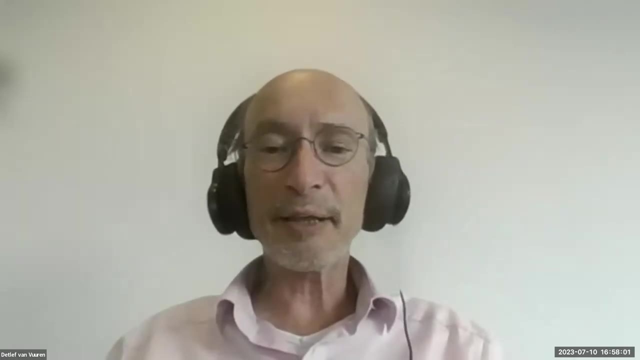 situation for us. So we believe that climate is important and so somehow we want to include it into the drive. that's why we do this exercise. But if we include them, this complicates the analysis, And so far we have always said: let's not include them and let's then the impact. 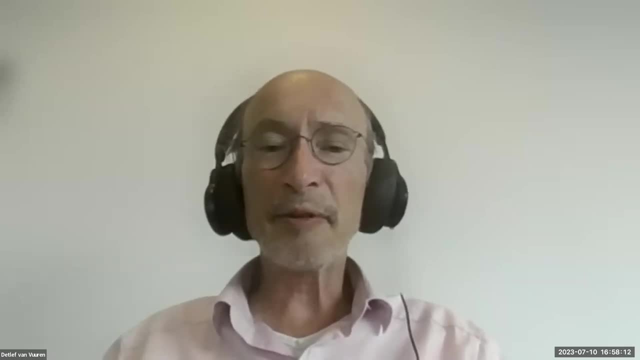 modelers have them included. We'll keep with that philosophy, but at some point this becomes unholdable, and so there might be, at some point, updates where we include climate impacts, and maybe those sets can be made available as well. Kevin, you raised your hand on this particular. 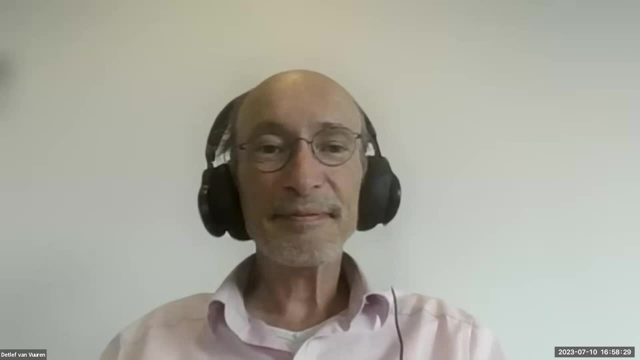 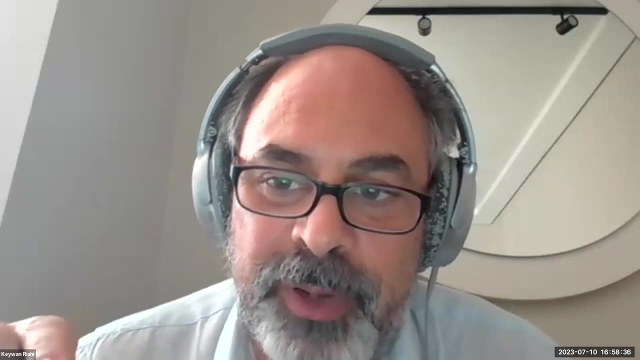 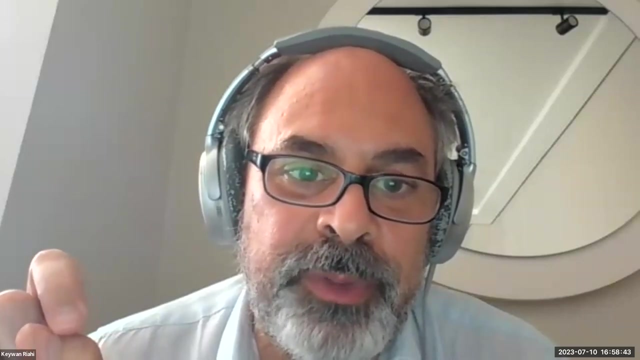 topic as well. I think That was actually not on a particular topic, but since there were a few questions asking about to which extent we provide input assumptions of the GDP projections, Rob, I was wondering whether you would like to say a little bit, whether the data set would include only GDP. 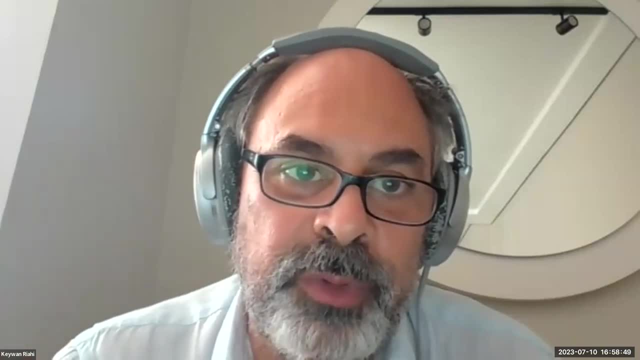 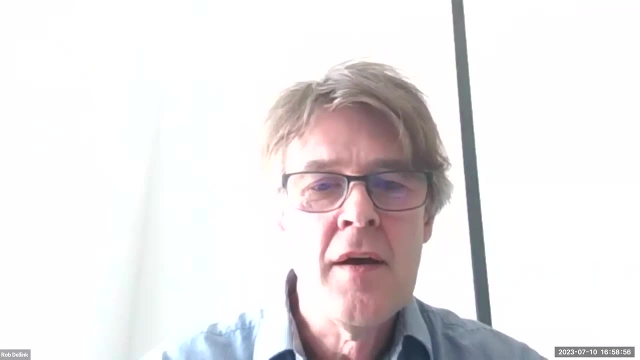 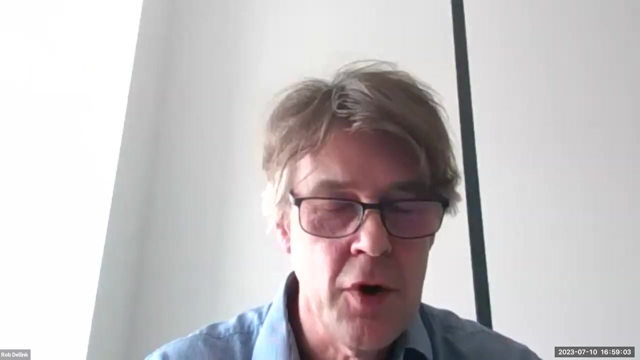 projections and which sort of underlying assumptions we would post. I think that would be useful. Yeah, so at the moment we just do GDP in PPP terms, so people can calculate income per capita by using some population data, because those are fully consistent. We. 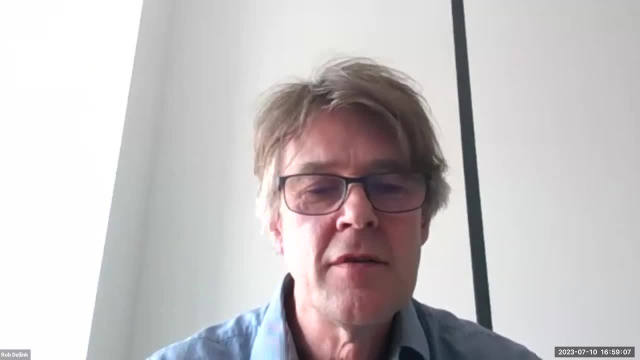 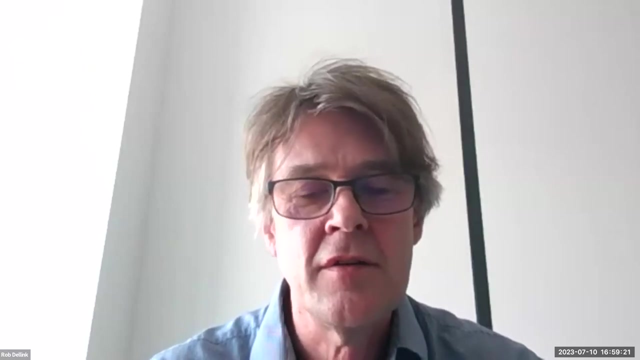 have harmonized fully with Samir's database. We're not planning at the moment to release any of the underlying drivers. We can reconsider this. We might also provide a more detailed database on the site, like Samir has been doing in his Zenodo, but we are definitely not doing that before we have. 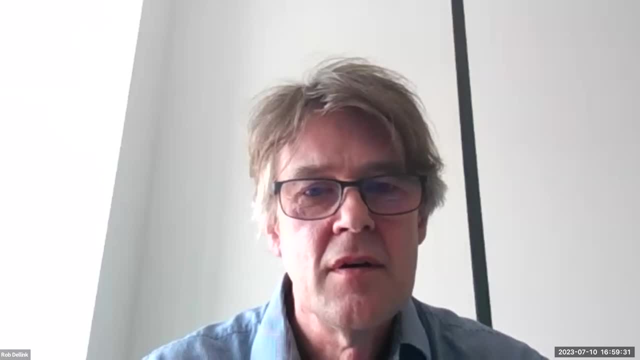 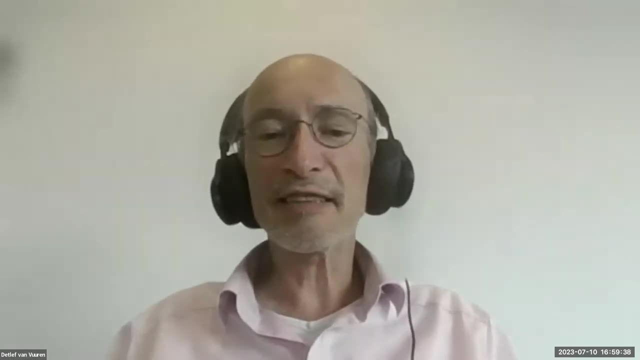 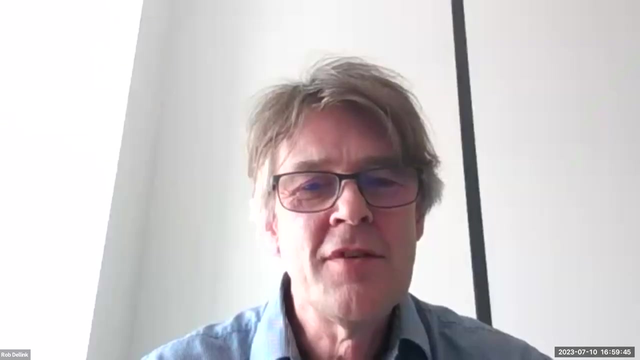 finalized our projections. Okay, I see mostly the questions related to economics, except if people have more general questions, please post them as well. I also promise, Detlef, I also promise to stay around for another five or ten minutes to answer some of these. 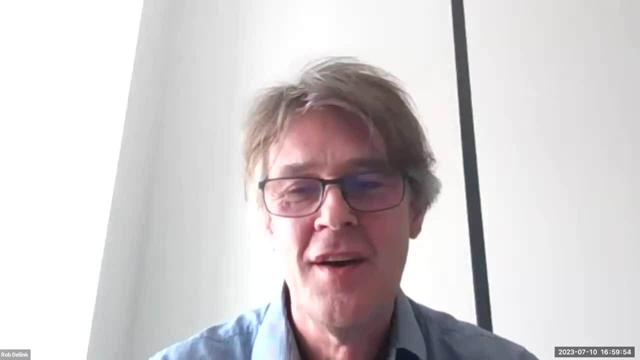 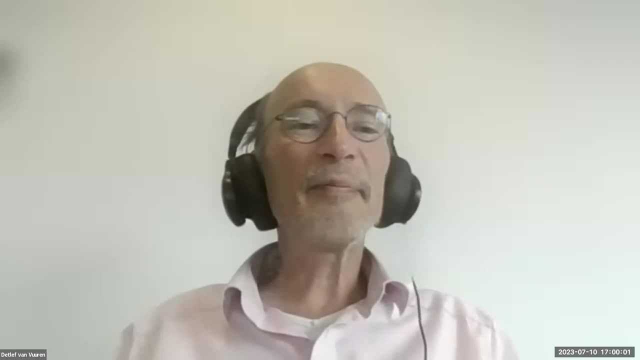 questions. So if your question is not answered yet by the end of this seminar, as long as the seminar is open, I'll try to answer some more questions. Yes, So maybe take the one of Nico, specifically on Russia and the former Soviet Union countries. 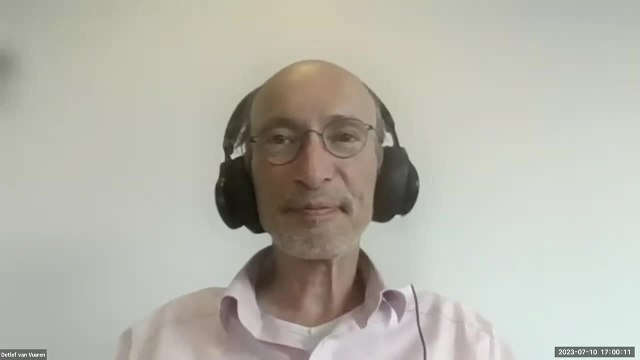 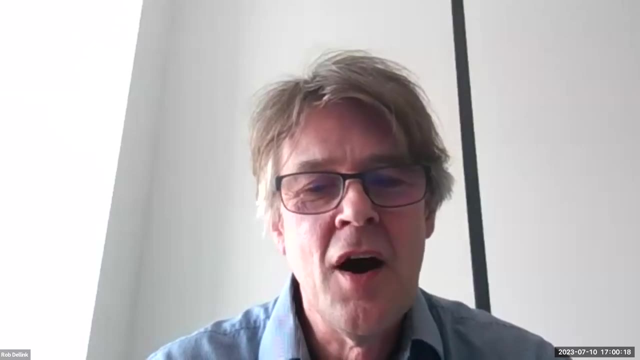 Can you say something about the GDP projections of those countries? Yes, So this is a very difficult one, because our projections stem from, basically, February, March 2023.. That's the short-term forecast that we have On Russia. these are projections made by the OECD. 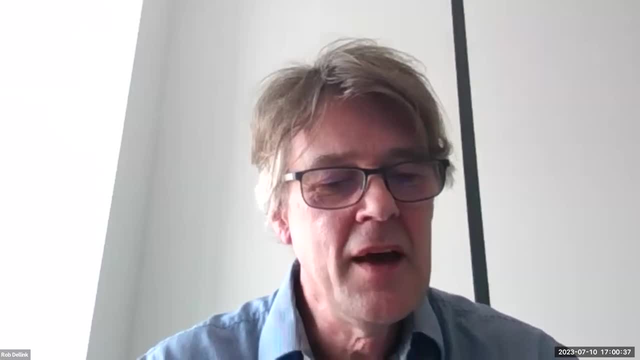 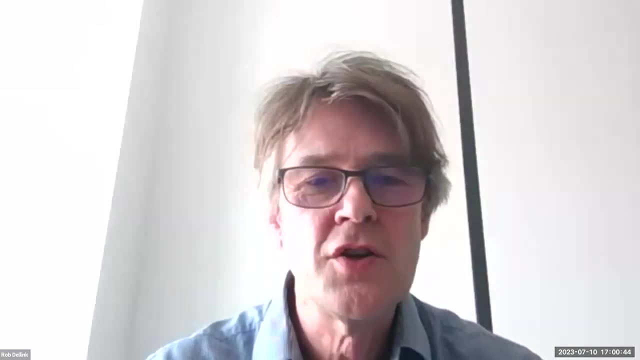 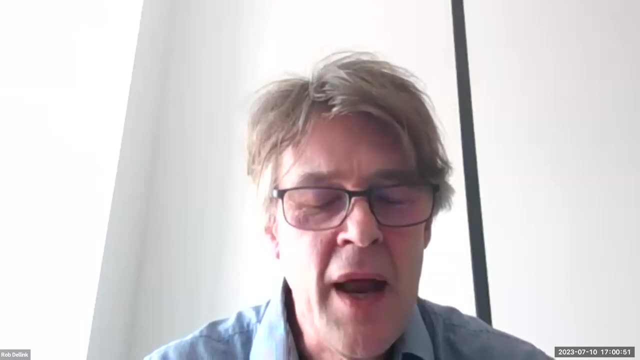 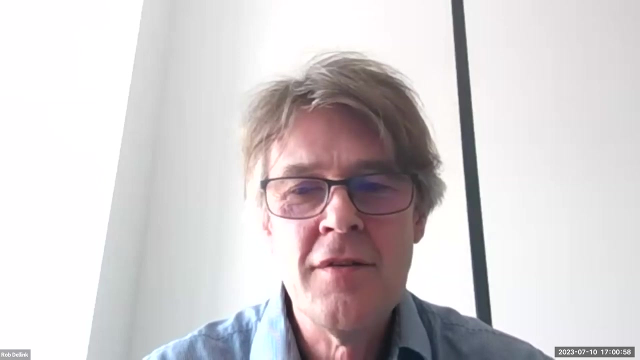 And they are recent, but they are trying to not preclude too much about an outcome of the war in the coming years. So they are in that sense they're embedding the start of the war, but they're not predicting any outcome of the war. 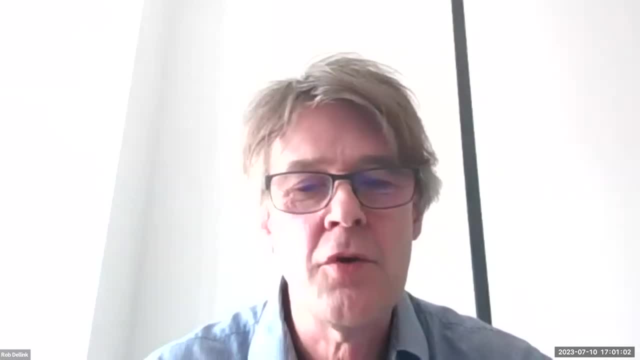 So you have to be very careful also with Ukraine And very recently. I would also be extremely careful when you look at data for Sudan, because currently the situation in Sudan has worsened quite a bit since our last projections. This is always the case. 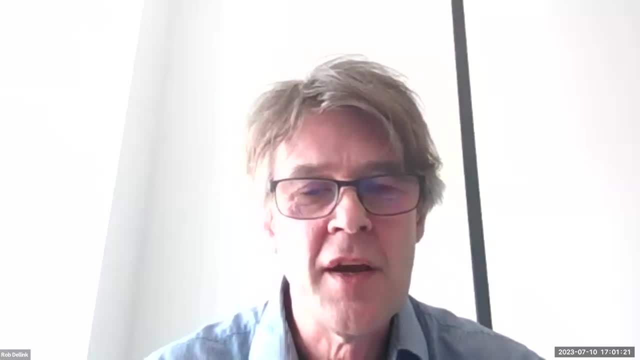 At some point we have a cutoff point. These are the geoeconomic and geopolitical circumstance that we can take into account, And everything after that is basically excluded from these projections. At the same time, we don't want to be too specific on what. would happen, And, for example, with Russia or with Ukraine, because the idea is that these scenarios would again take maybe 10 years before they get an update. Maybe we'll do an update earlier, but they should have some longevity, So we don't want to have too bold assumptions. 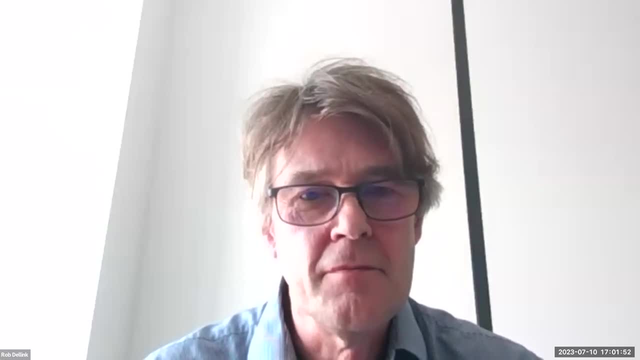 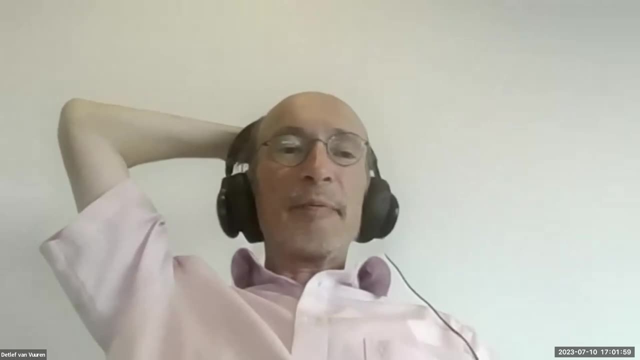 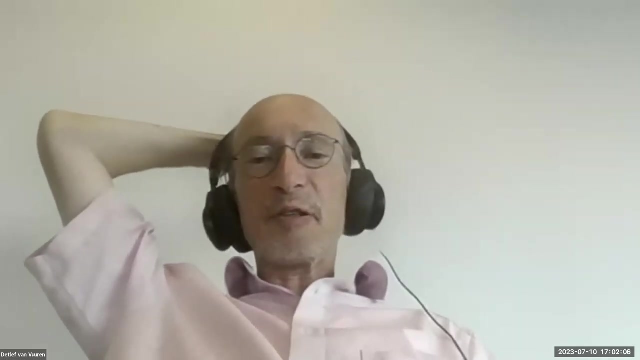 on the outcome of geopolitical circumstances. So you are using Samir's projections for labor, And how do you map France's educational education? And how would you wait for that to be accurate up to the end, With this quick analysis and this blame against labor, Jesus? 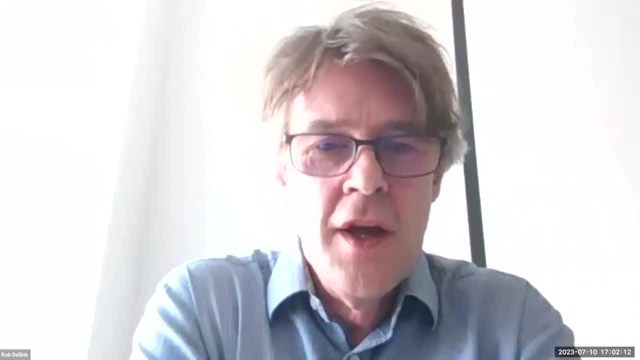 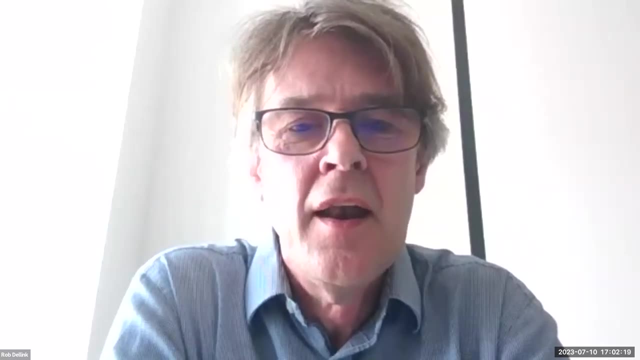 what are our expectations? How do you make those look consistent For the może? enough, you know what I'm saying, You know what I'm trying to say. We take the mean years of schooling that Samir provides for the age groups and for their gender. 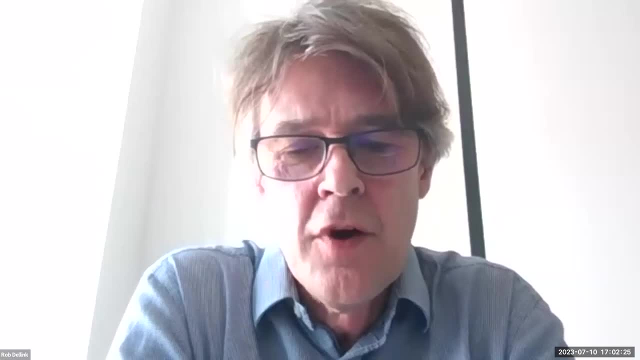 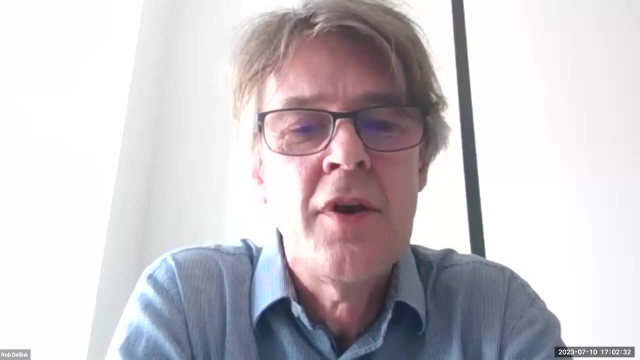 Again it's about хорошо for Samir. Again it's about heckle for Adam. Canada etwasni growth IRA. Adam Molingова vemês- misunderstood. How do you make those look consistent? We take the mean years of schooling that Samir provides. 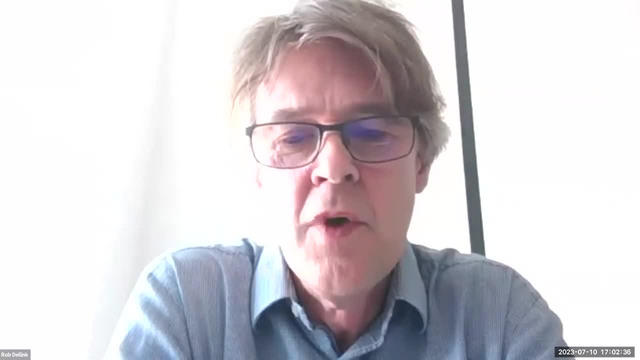 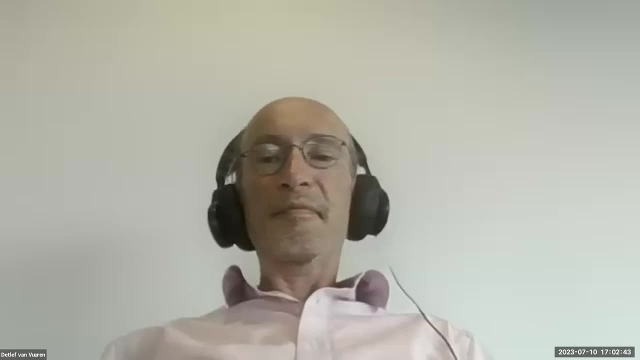 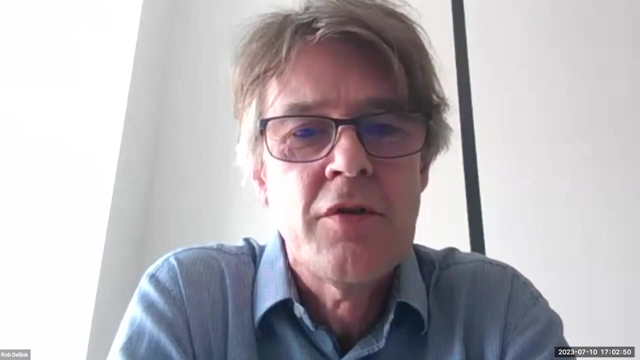 labor force by age group and gender and we multiply that, we use that as weights for then aggregating the mean years of schooling to the educational attainments, uh, to over the age groups and gender, and that comes up with a total labor force human capital indicator that we then put. 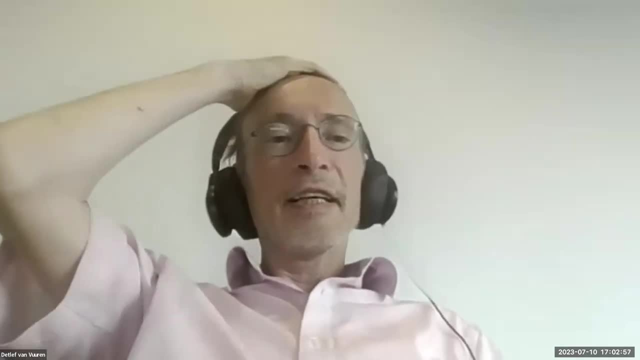 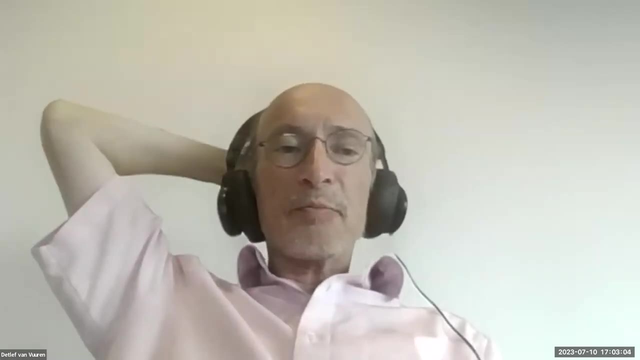 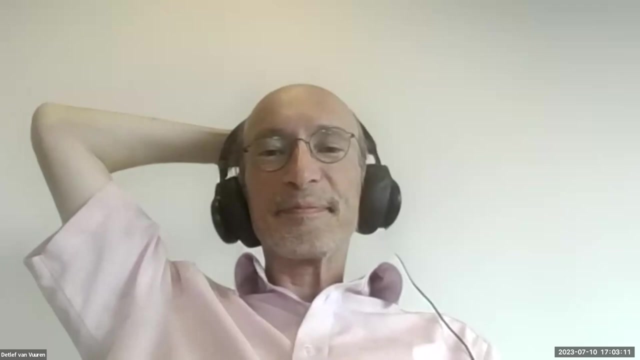 into the model. okay, great um. so for marina, the question would be: um, how do you make your assumptions for labor force projections for 2030 and how this is related to the lfpr? yes, so the labor force participation rates? um is really the thing that we have been struggling with. 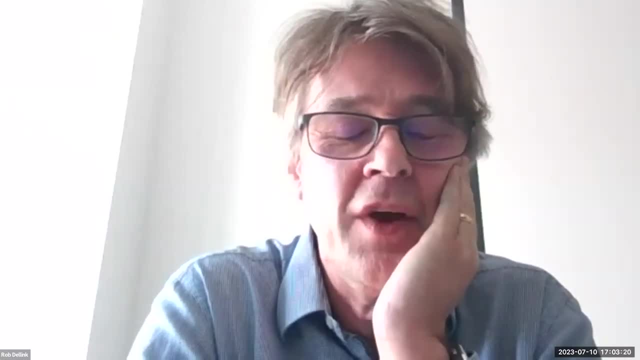 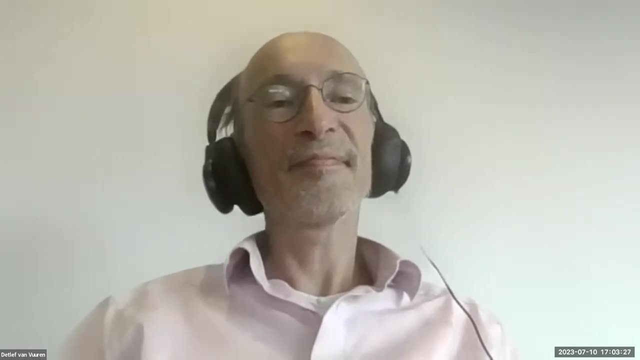 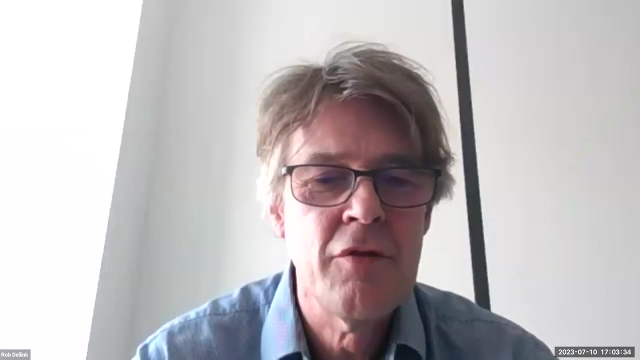 recently the most, because there are no. we can't find any very good uh database. we have some information on labor force from our economics department, but that's for a subset of countries. so what we're doing is we're actually using the detailed data from ilo in 2018 combined. 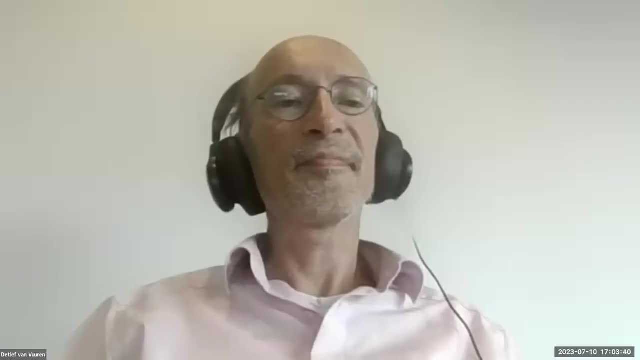 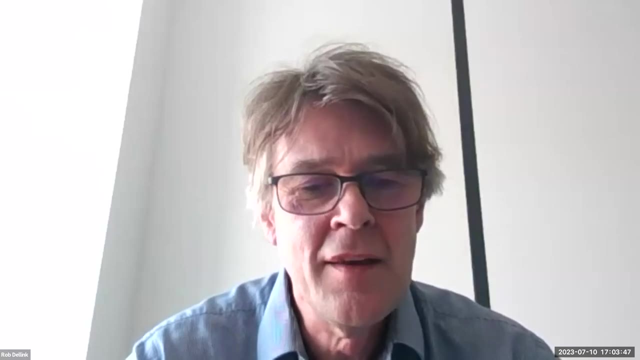 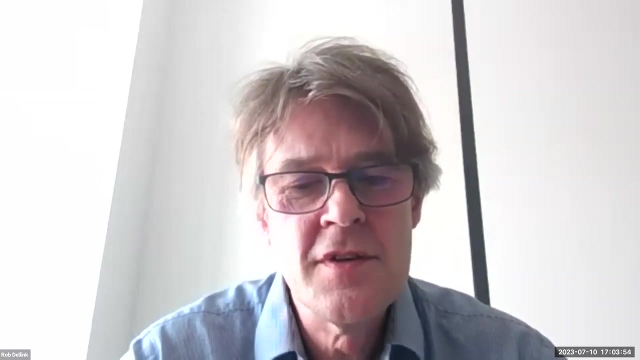 that, with some short-term revisions, that ilo did for total labor force, uh, age 15 and plus, so not for the age groups. uh, we combine that um, but it is not really satisfactory and the projections after 20- 30 use the same methodology that we use for basically everything else, also after. 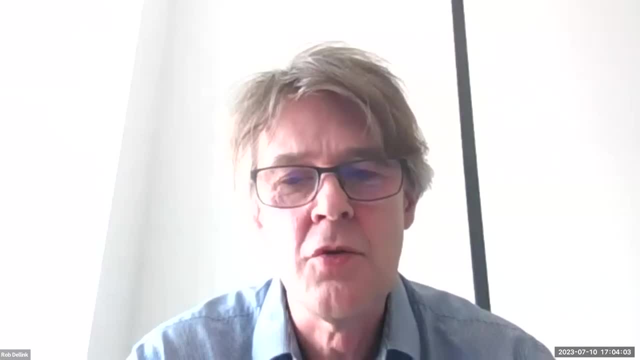 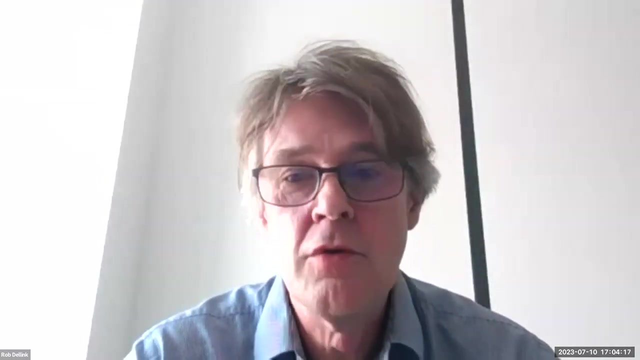 after we have the data run out, and that is, we use gradual convergence across countries with a country-specific element in there and very gradually we have these labor force participation rates converging over time. if somebody knows good improvements of this, i'm happy to have a bilateral conversation. 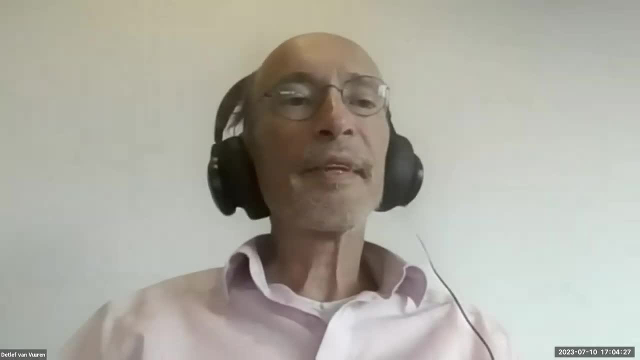 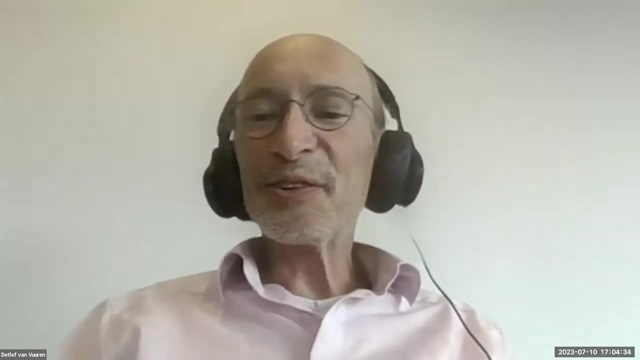 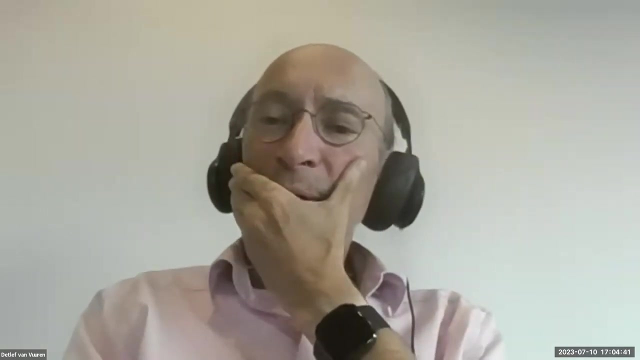 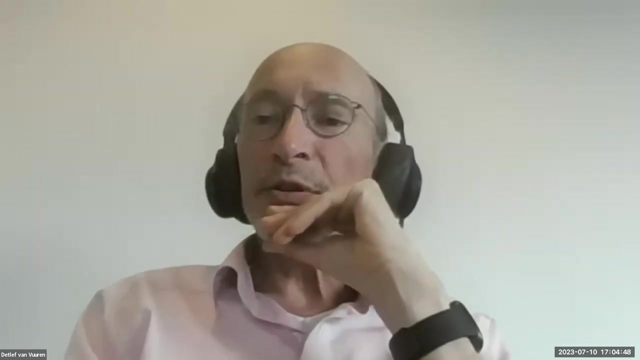 there were also um a suggestion. so there's a question um which came in, is if the- and we discussed it a bit earlier- but the base year of the us dollars, um. so maybe would it be interesting to provide a quick answer to that question, um. i think it's a good question, um. i think it's a good question um. i. think it's a good question, um i i think it's a really good question, um i think it'll be very i think it's a really good question, um i think it's a good question. um i think it's a good question, Lord dosas. yes, 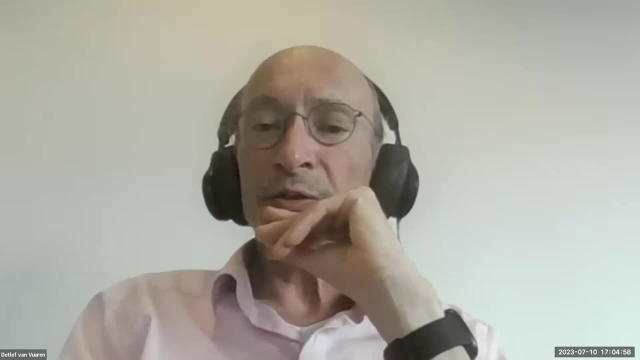 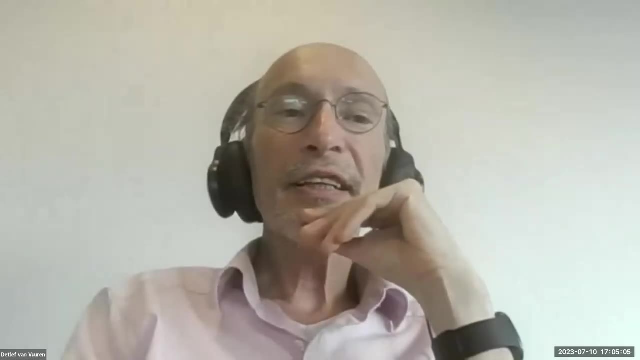 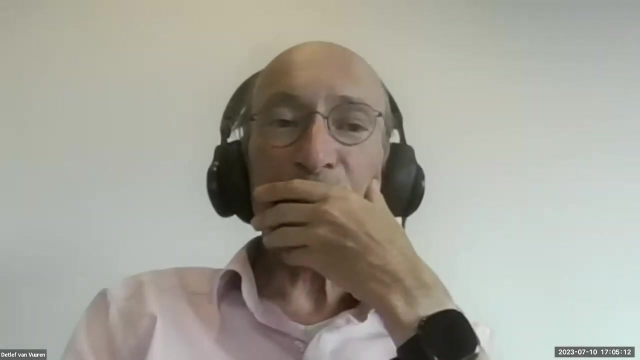 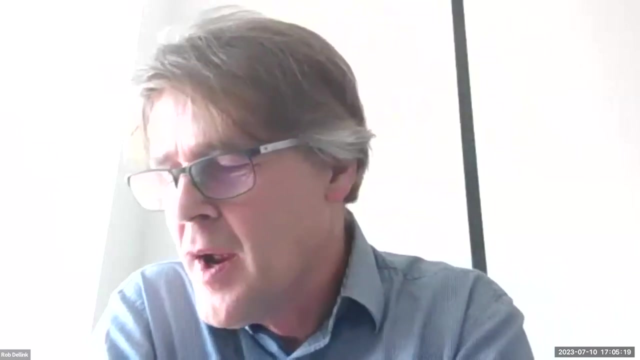 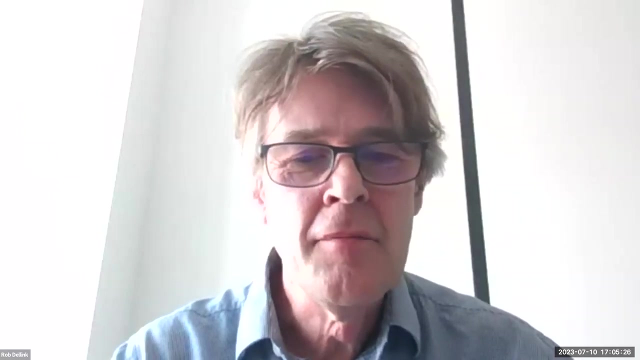 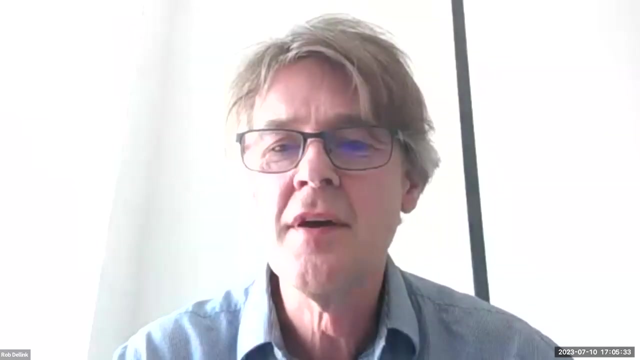 we and you could also refer to a number of devices, but, like, on top of that, we have, uh, a lot of eyebrow extraction rents at the country level, um, and we do have information, for example, on prices, and that's something that bloomberg also provides, but uh, i was at yarmouth. give that comment then. 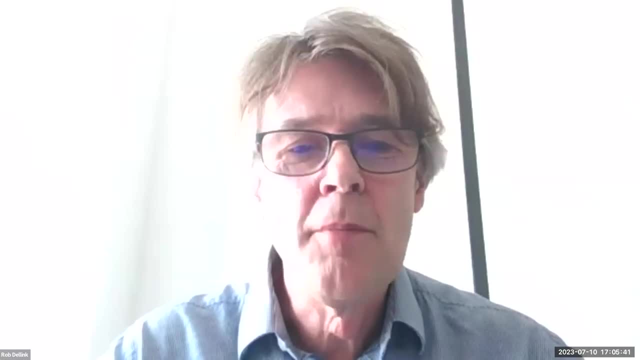 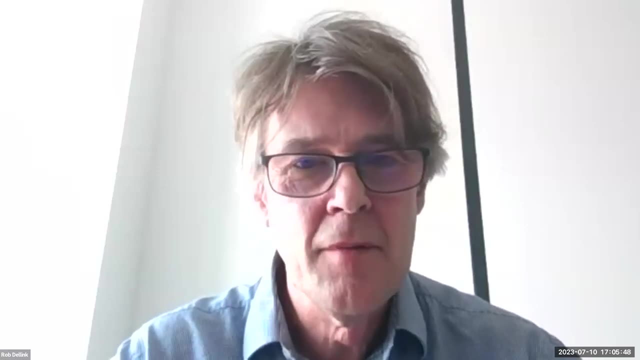 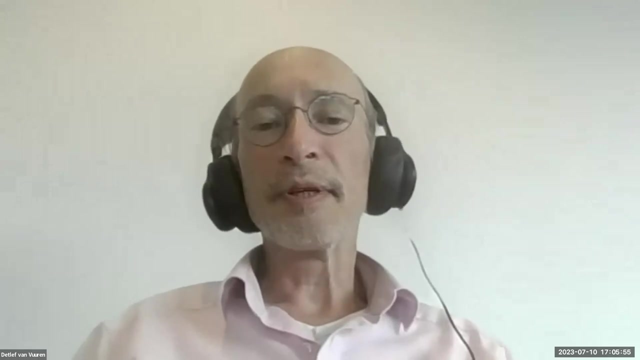 maybe follow up literally and and tell me where to look. um, i might have overlooked. it would be great if we have that information, but i doubt it is exactly what we need. yeah, we are we're slightly over time now and so, um again, if there is questions related much more to the 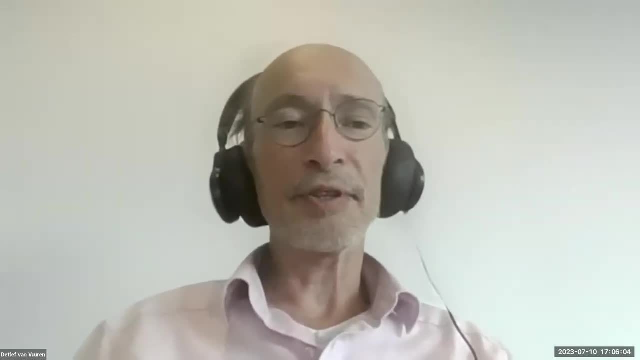 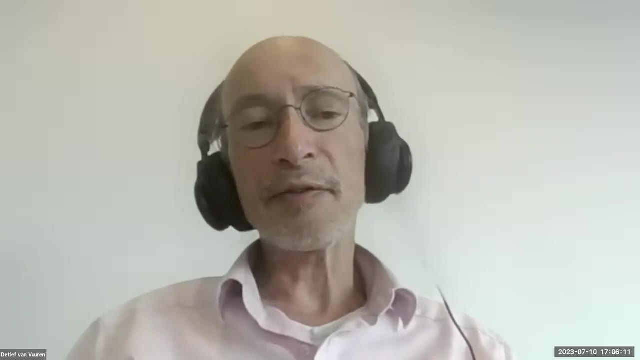 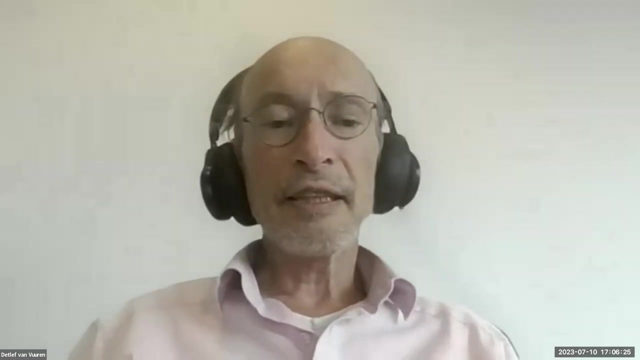 process overall. i think those are would be also really important. uh, so, again, if people have questions about our timeline, our way that we are running the um, um, the review period, please come in because, um, it's the last five minutes, certainly also for that and um amir's warning me that there's a hand raised. 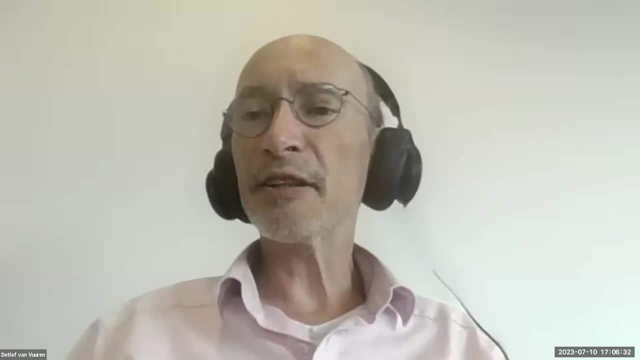 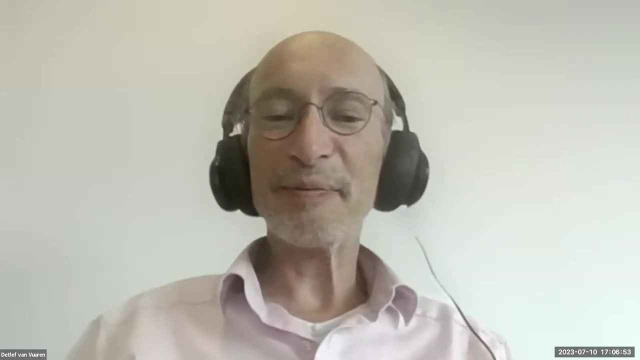 so maybe, maybe, daniel and nevado, let's see whether i can allow you to talk. i think you can immute. can you try that? i think you would need to make him a panelist or so. yeah, everybody did that because you can see him. but uh, okay then, uh, here, daniel still needs to unmute himself, i think. 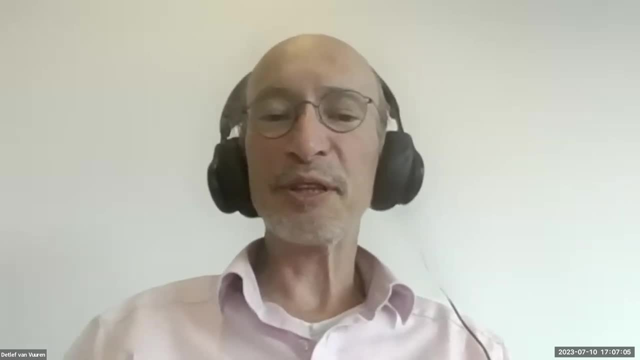 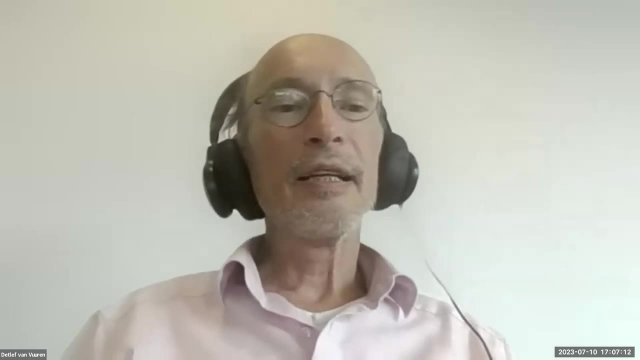 if it doesn't work, daniel, then please put the question into the q a, but in principle, i think you could speak. oh, wow, okay, in the meanwhile, um, let me pick up and one or two questions from the um, from the audience. um, so there's one comment by armo. uh, how important it might be to consider. 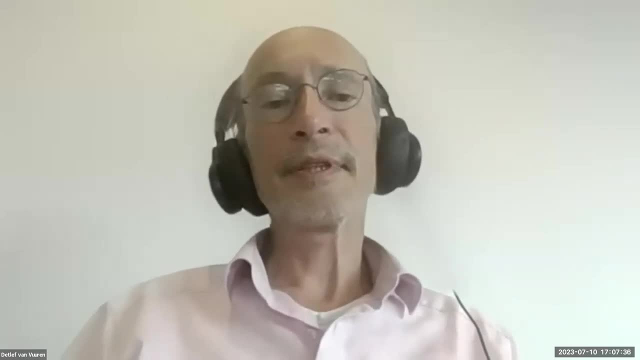 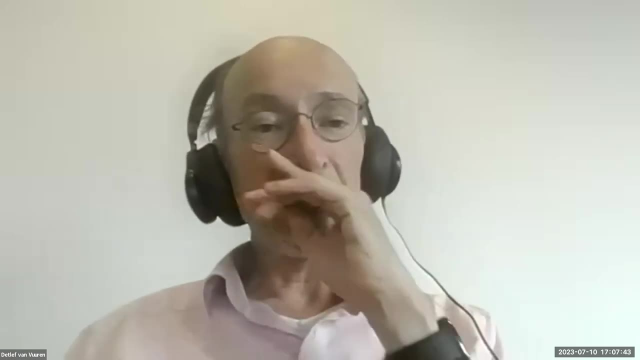 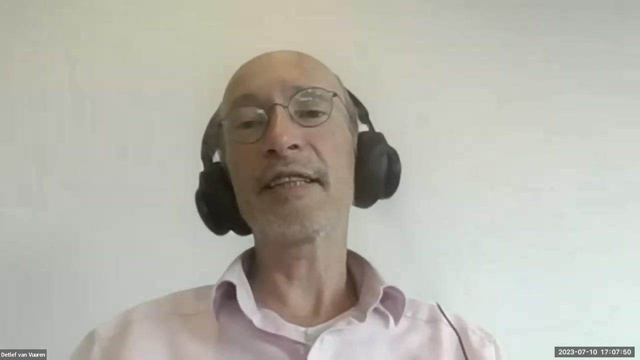 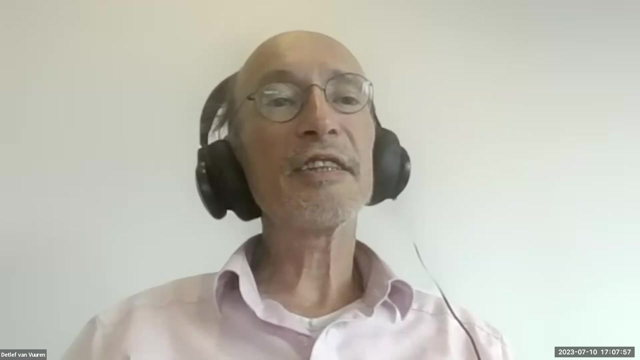 the release of also the underlying data, which would be, let's consider that, how much we can indeed release, and i already heard your response to that, rob. so this is something that you might want to be willing to consider, but not at this stage, and the rest at this point of time, i think, are more seditions and then and anything else. so you 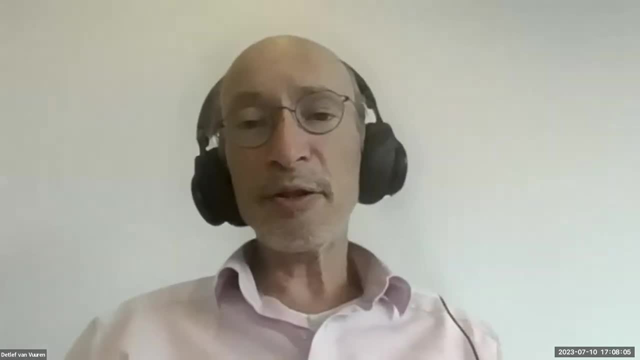 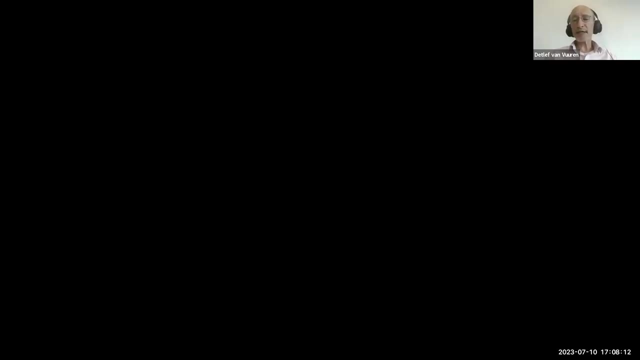 might want to have a look at this, but that means that i think it might be good to start rounding up. it might be good if we share the slide again. i'm trying to do that with the link to where we can. you can provide comments and everyone you would like to say. 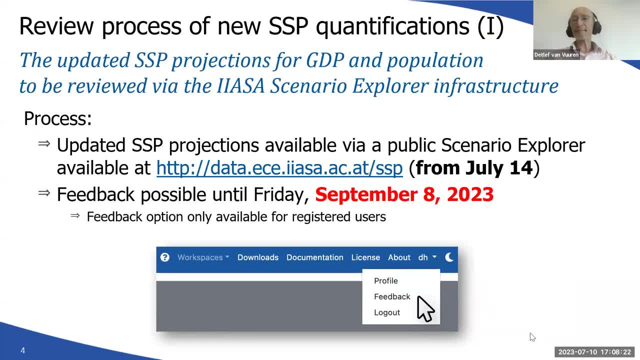 something about that. so come in. actually, i wanted to do exactly the same uh that left. i wanted to share this, uh the slide, so that everybody knows where the link is. um, so if you go to this link here that you see in front of us, so take a screenshot. i think that's the best way to do this. um, on the 14th of july we will. 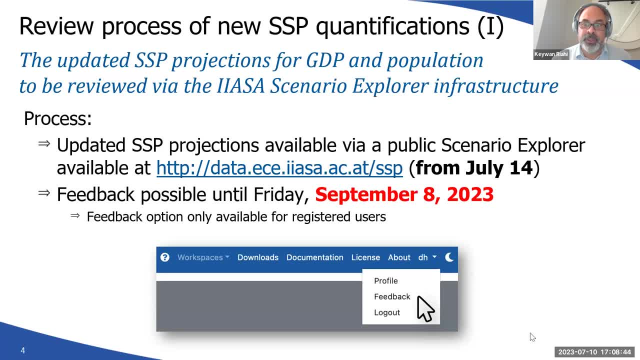 open the database and, as of that time, um, you will be able to send us feedback to this feedback form. um, you, you, you. if you have technical uh problems, uh, you can also get in touch with our colleague, daniel hookman. but the system has been tested so i think it should be possible um to do this and 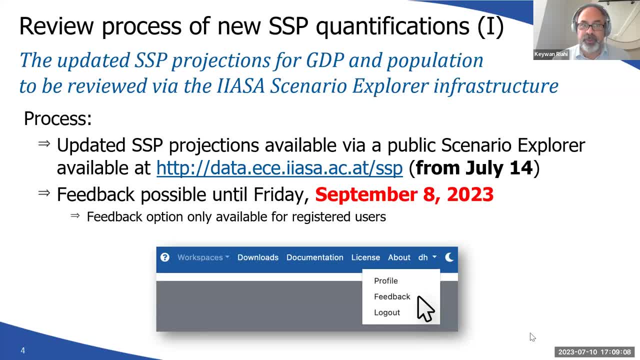 we would look forward to your feedback by 8th of september. i thought it might be useful to repeat that, yes, that's great, and um, we are, we are willing to share the slides. uh, so we have to find a way to best do that as well, because actually, 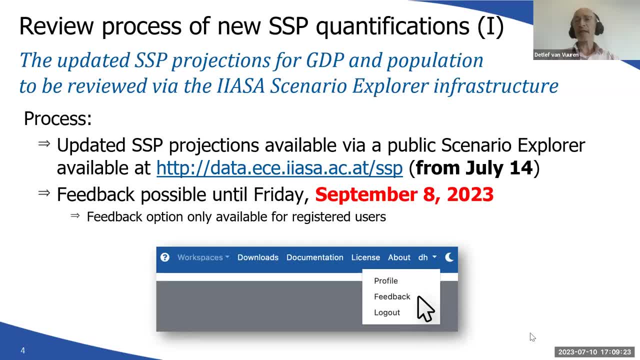 especially the slide deck that uh payone showed, of course, is giving some very helpful guidance on how we would like to run the review so that that slide deck could be shared as widely as possible. i think, yeah, we would. we would put this- that left, i think, on the web page as well. so if 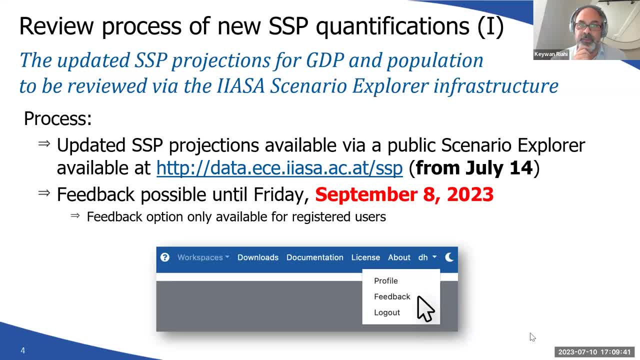 you register, you can then directly download it. download it there, i think. yeah, you don't have. yeah, you will then have all the information there's. there's a slight catchy play to there as well, because you don't have to do that, you don't have to do that, you don't have to do that, you don't. 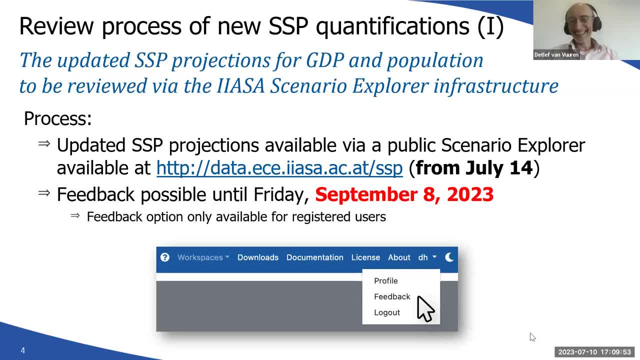 have to link without the presentation. that's actually true. yeah, so that's the better way. yeah, but we can communicate also this uh information via and mailing list to iconics and imc. okay, great, i think this was a great webinar. um, the presentations by samir and um by rob were really, really helpful in trying to understand. 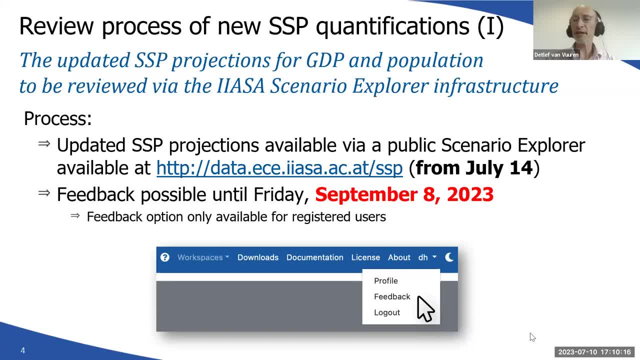 which revisions have been made, and i enjoyed also the conversation on the questions um, so hope to see you soon back at a new iconics webinar, and i hope really that people participate in the review, because we want to make these scenarios as good as possible. thank you, and thank you for the speakers.